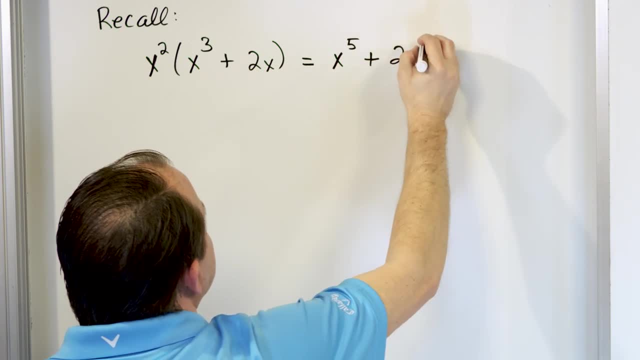 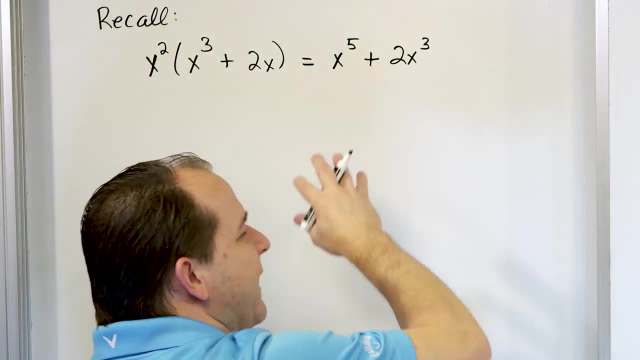 the x squared times the x gives you 2x to the cubed power. The reason that it's a plus is because you have a positive term times a positive term gives you a positive term. If you don't understand that, then you need to go back and review the last several lessons. 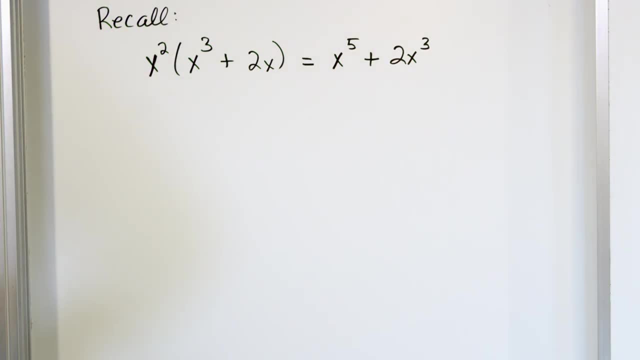 where we've done that kind of work. Now, the next most common thing that we're going to run into- or the next most complex thing, I should say- is what we learned in the last section, And that is that we can take something more. 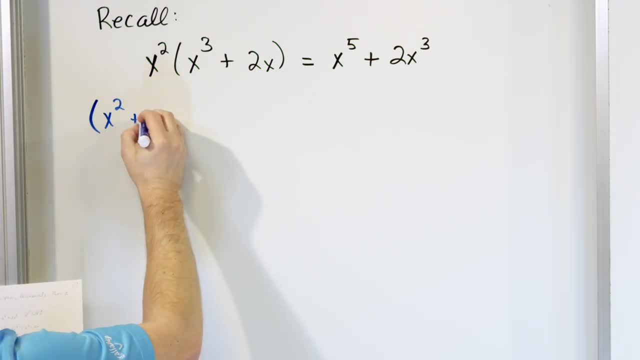 complicated on the outsides. for instance, x squared plus 1 on the outside, and multiply it by a binomial, So we have x cubed Again- let's just make it easy- plus 2x. So you see, here we've had the same exact binomial. Now we're multiplying. it times something a little. 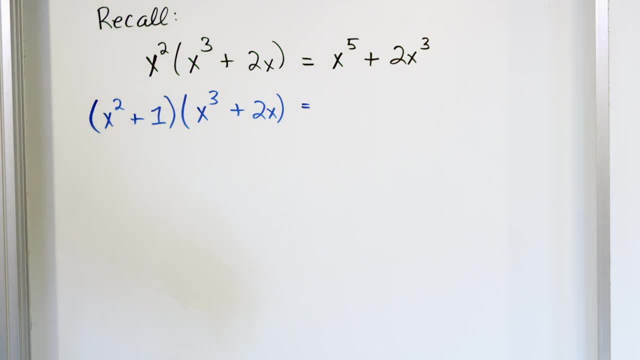 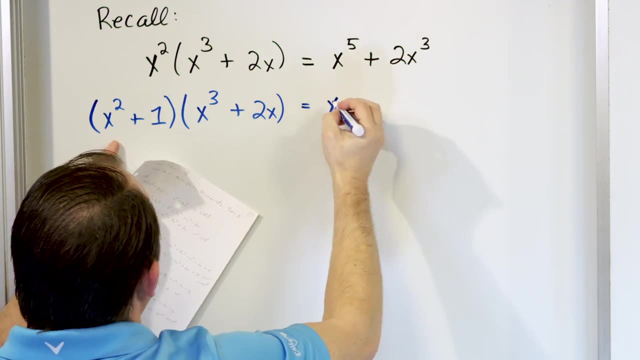 more complicated on the outside, But, as you should know by now, all you do is pretend that the 1 is not there. You take this and distribute it in, And so what you're going to get is what we just got before. You'll have x to the fifth plus 2x to the fifth. 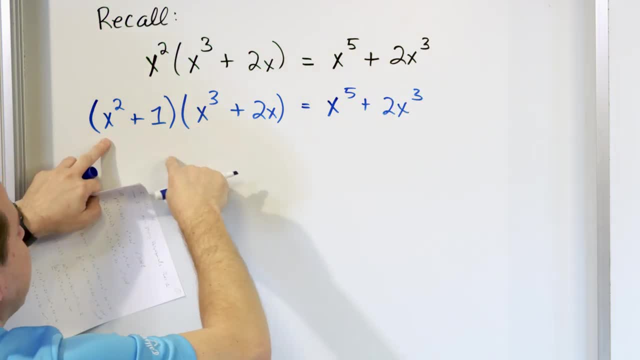 That's 2x to the third. That's this times this and then this times this. Then you pretend this is not here And multiply the 1 in times here. You get another x to the third power And you take this and multiply it times this And that gives you 2x. So you have four terms. 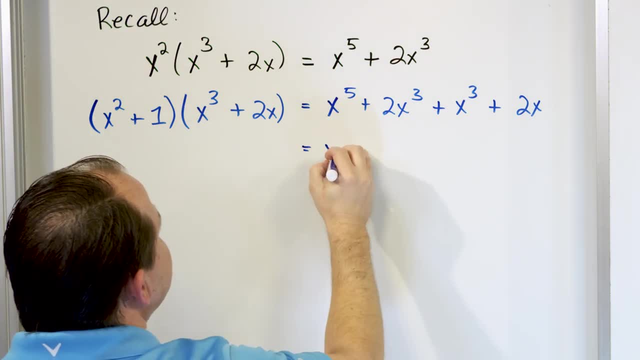 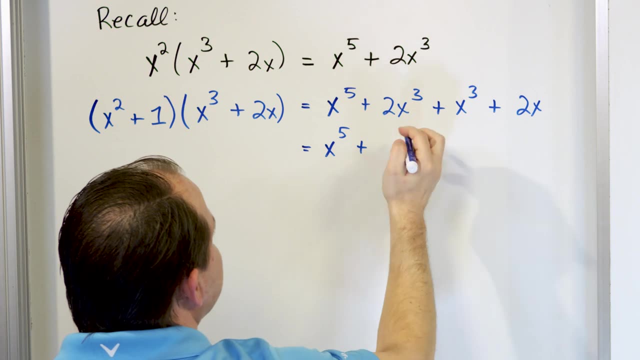 And now you see you have these terms that can be combined together. So for the final answer, you'll have x to the fifth power, plus, since these are the same exact variables and exponents, you can add them together: 2 plus 1 is 3. And you'll have x to the third power. 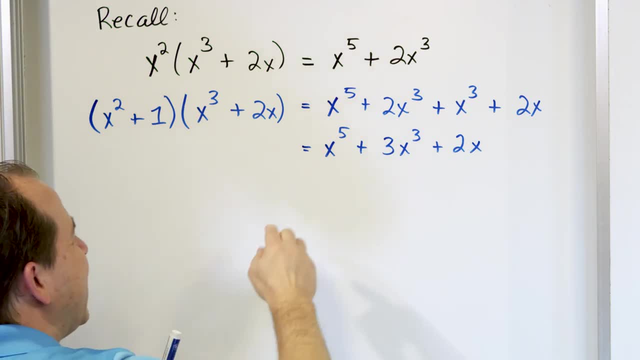 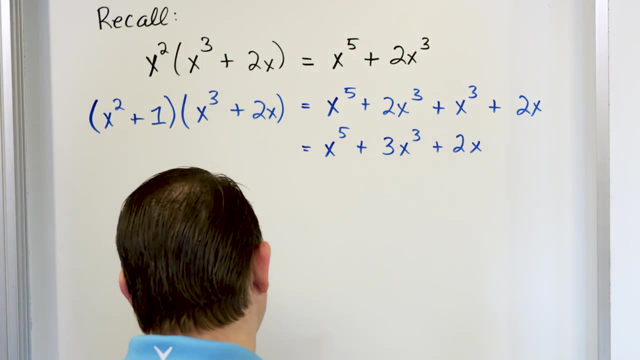 And then this comes along for the ride, because we can't do anything else with it. We cannot add these terms together because they have different exponents of x. This is a different term than this one, which is different than this one. So you have x to the fifth. 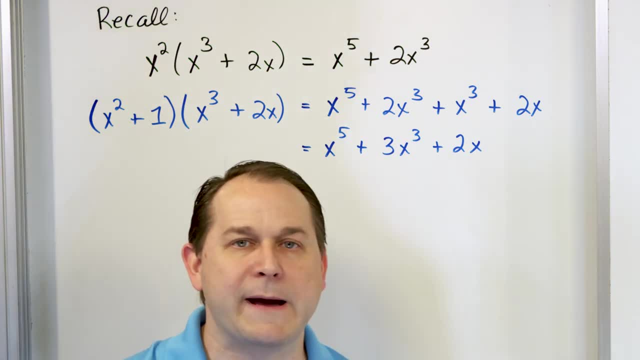 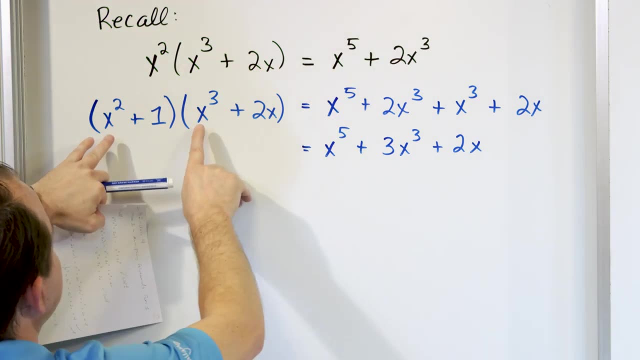 plus 3x to the third, plus 2x. Now, what we talked about in the last section was the concept of FOIL, And that's what we just did. I just didn't call it FOIL. But what you have here is this first term is the first, the f term, the first terms, And then the outside terms. 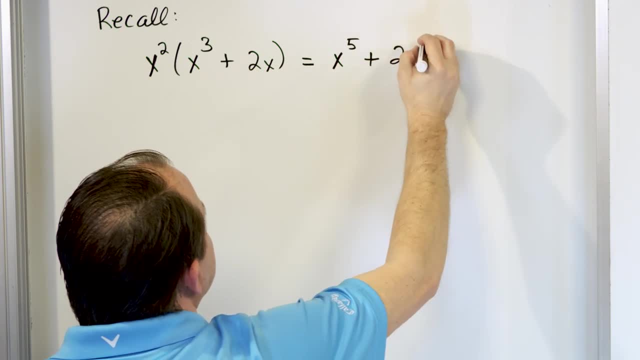 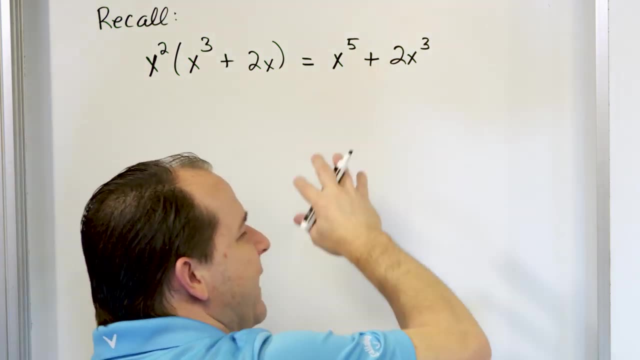 the x squared times the x gives you 2x to the cubed power. The reason that it's a plus is because you have a positive term times a positive term gives you a positive term. If you don't understand that, then you need to go back and review the last several lessons. 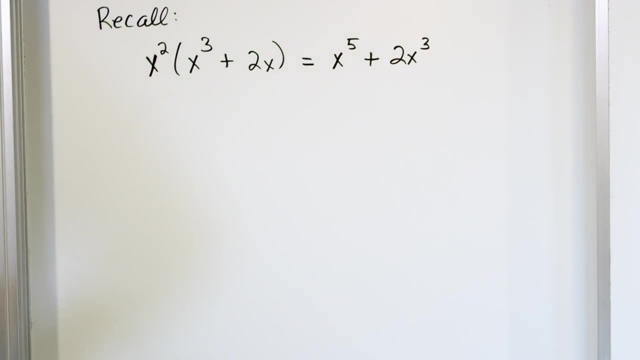 where we've done that kind of work. Now, the next most common thing that we're going to run into, the next most complex thing, I should say, is what we learned in the last section. There was further explanation of this two sobre. We just 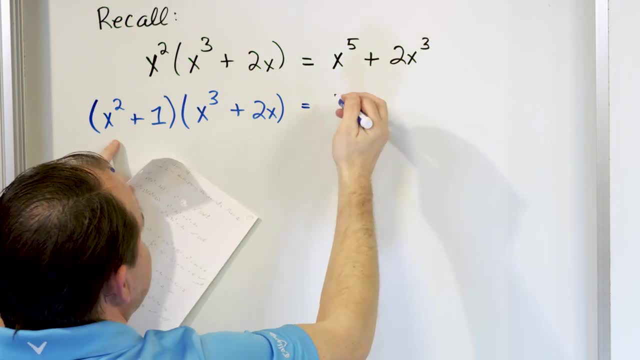 ignore this formula today. It's still not very important and it's kind of unloaded, Just kind of that catch up alright. So you begin to graduate and finally we get to learn about's math. Desktop Boston. We're going to have a冷 허. And then we're going to move these things around. so the geometry needs to work, And that's always a very complex provision. I think Sewing something down here might take a lot of time, So we're going to interpret it in this way. 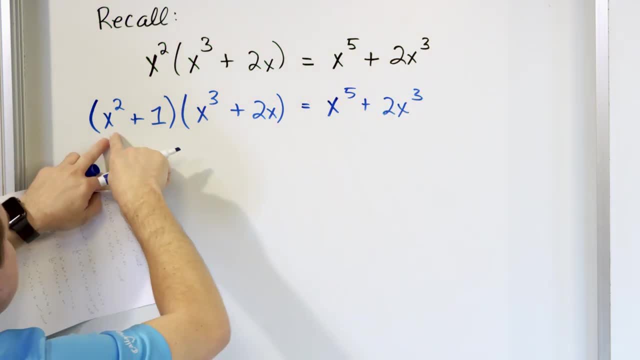 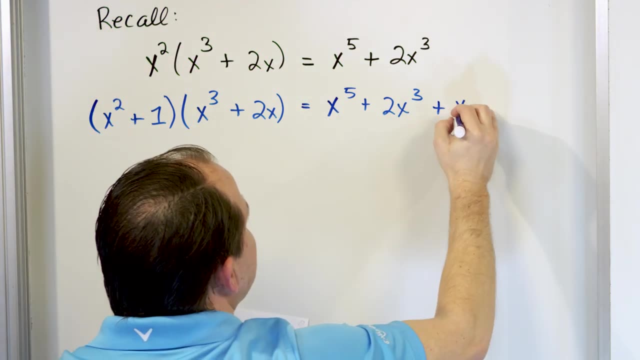 How many times does it take to get this right and how do you predict where you want it toО? tell this: females plus 2x to the third, That's this times this and then this times this. Then you pretend this is not here and multiply the one n times here. You get another x. 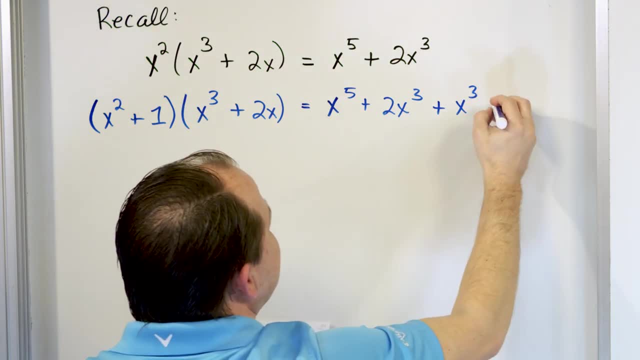 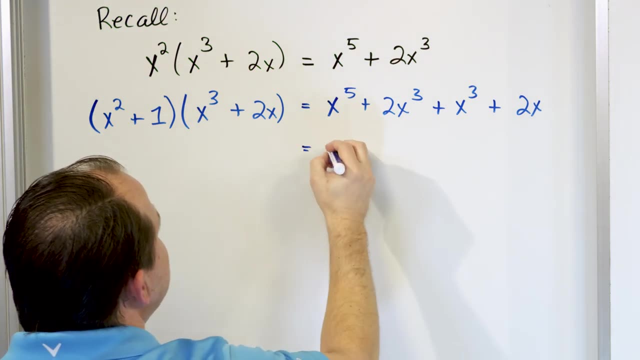 to the third power and you take this and multiply it, times this and that gives you 2x. So you have four terms. and now you see you have these terms that can be combined together. So for the final answer you'll have x to the fifth power. 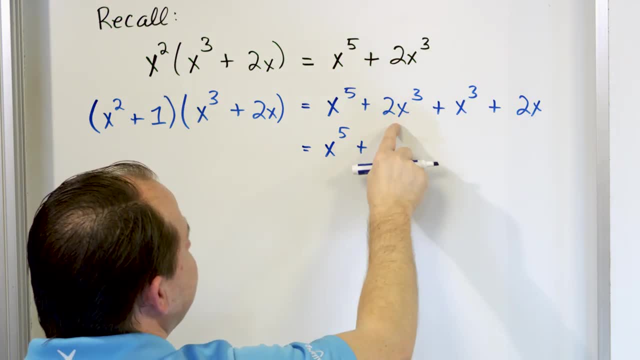 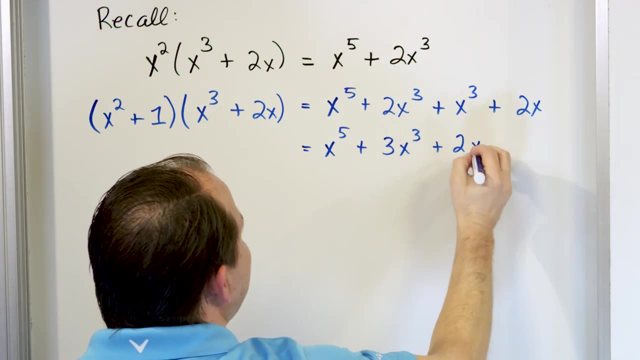 plus, since these are the same exact variables and exponents, you can add them together. 2 plus 1 is 3 and you'll have x to the third power. and then this comes along for the ride, because we can't do anything else with it. We cannot add. 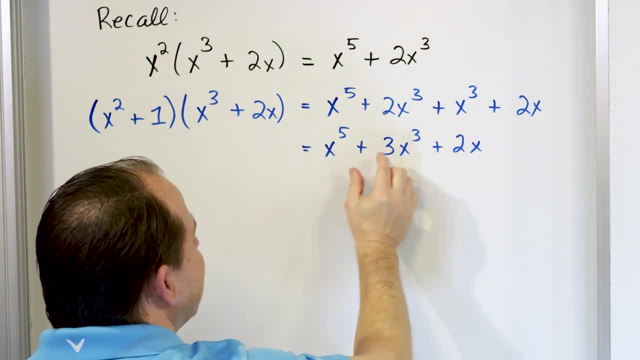 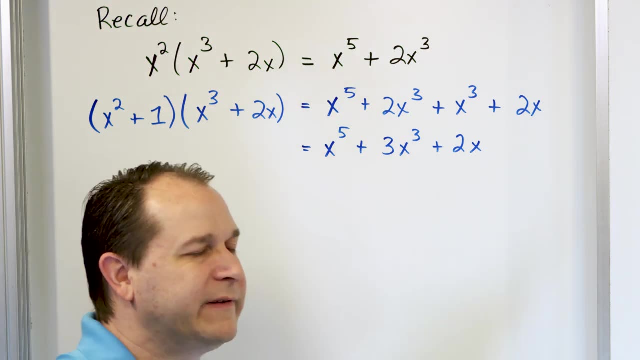 these terms together because they have different exponents of x. This is a different term than this one, which is a different than this one. So you have x to the fifth plus 3x to the third plus 2x. Now what we talked about in the last. 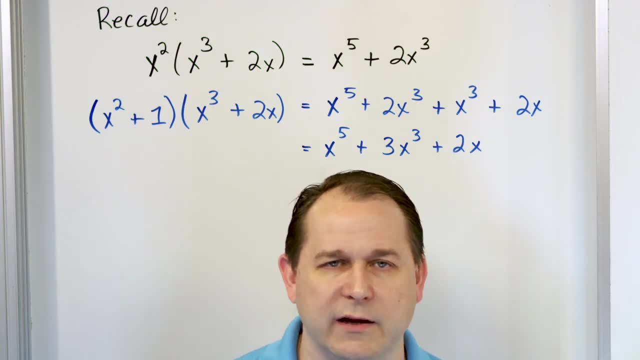 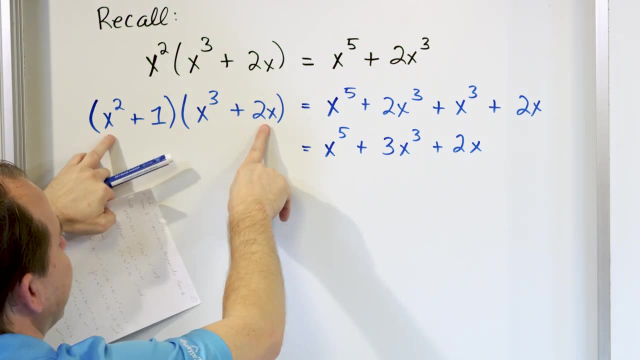 section was the concept of FOIL, and that's what we just did. I just didn't call it FOIL. But what you have here is this first term is the first, the f term, the first terms, and then the outside terms. are these two giving you this one? The inside terms? are these two giving you? 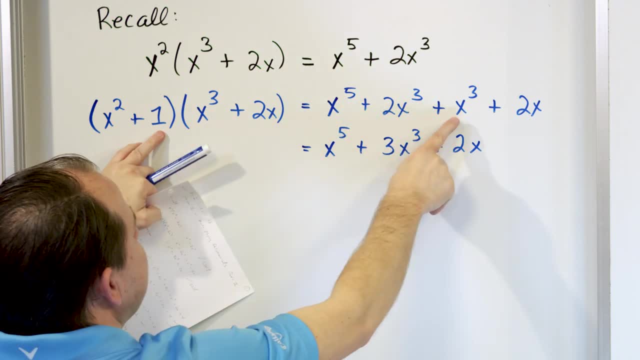 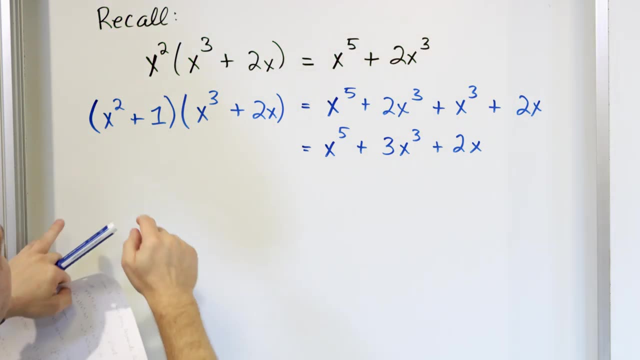 are these two giving you this one? The inside terms: are these two giving you this one? And the last term: are these two giving you this one? So think of it as FOIL, Or what I like to say is think of it as covering this up, distribute this in and then cover this. 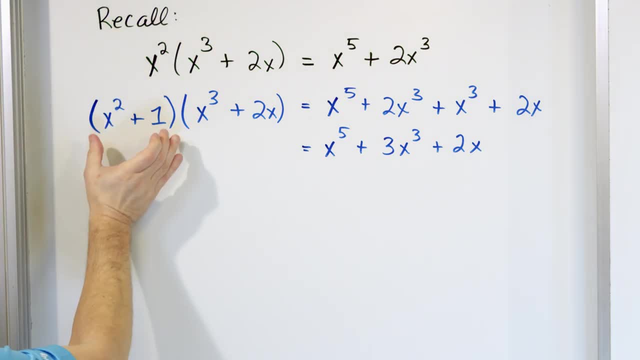 up, distribute this in. Basically, everything on the outside has to go in and multiply by everything on the inside. And the reason why I'm explaining to you that way is because in this lesson we're going to be multiplying more complex things than this. Let's say: 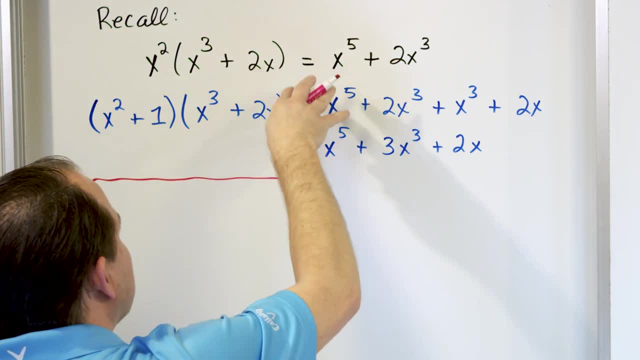 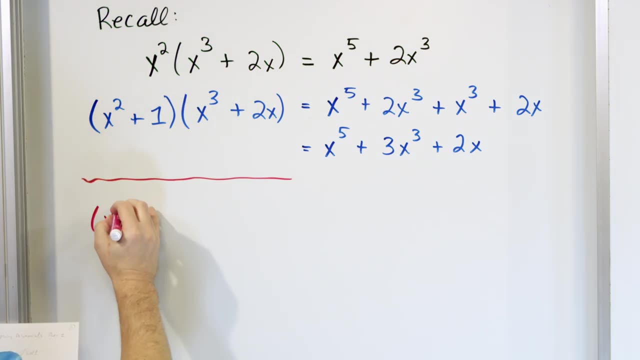 for example, let's get to the material of today's lesson, A little more complicated than what we've done. By extension, what if I have the same thing on the outside here? Let's call it x squared plus 1 on the outside, But on the inside I change this and make it a little more complicated. 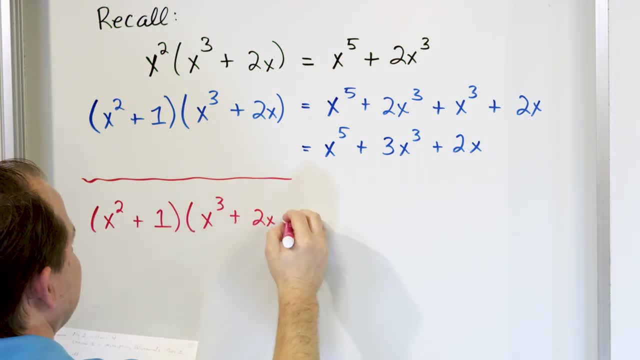 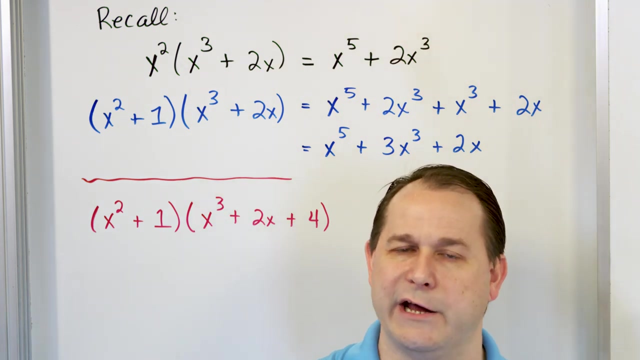 x to the third power, plus 2x, plus, let's say, plus 4.. Now if you didn't learn it this way, then you might be very confused about how to handle that, Because most students, when you're taught this, you learn binomial times, binomial- You learn FOIL first, outside, inside. 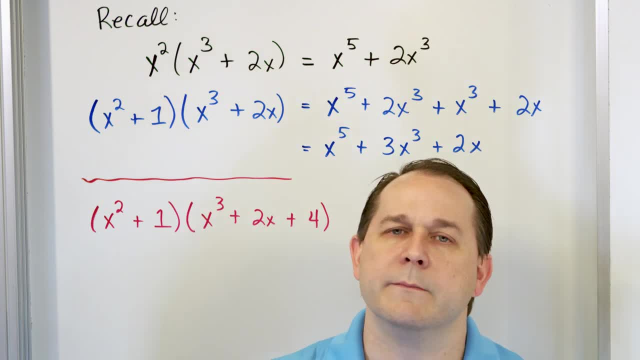 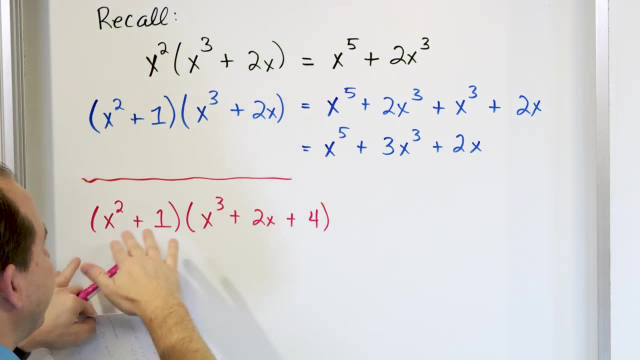 inner last, First outside inner last. You just learn to do it right. But the problem is, if you just memorize FOIL, then you have no idea how to handle this because you don't know which are the first terms, which are the last terms. I mean, you might guess these. 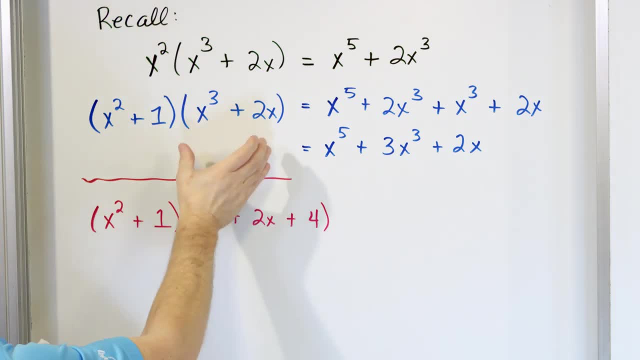 are the last terms, but which ones are the inside and the outer? because it doesn't match this cookie-cutter thing. So that's why this whole time I've been telling you: visualize it as x squared times this, these two terms separately, and then cover this and visualize it as these two terms. 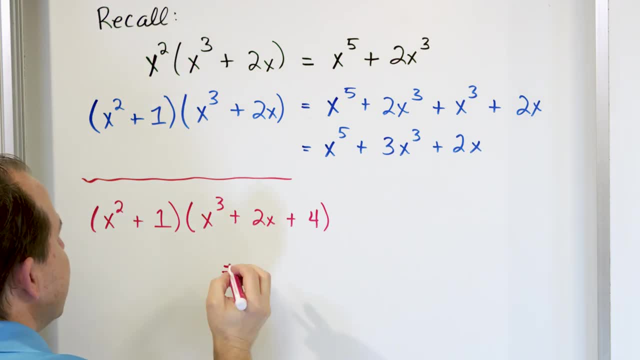 Why did I do that? Because now that we have a more complex problem, you don't memorize FOIL. What you do is you cover up the one and you pretend all you have is this: So these two terms multiplied together is x to the fifth power, And then again the one is not there. Then you distribute. 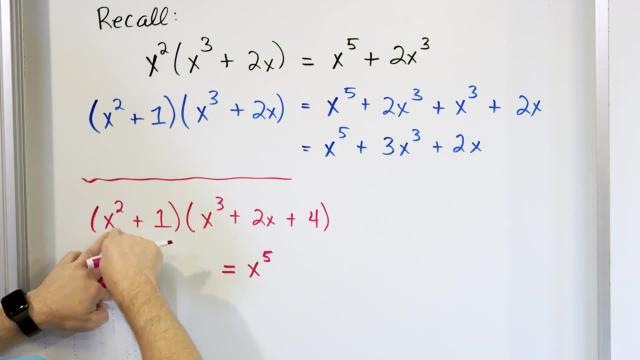 this one into this one. 2x times the x squared gives you 2x to the third power. We just add these exponents, Then you take this one and you go into the last one and you'll have four times the one gives you four, and then x squared is right there. 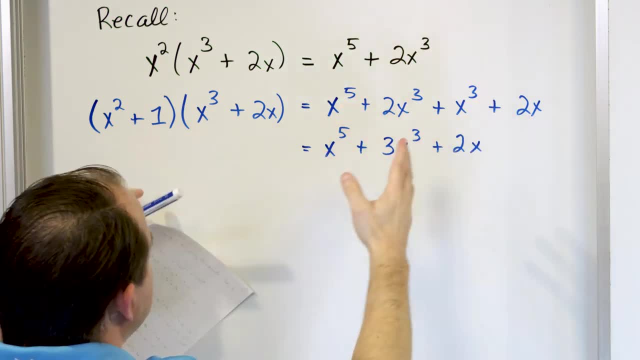 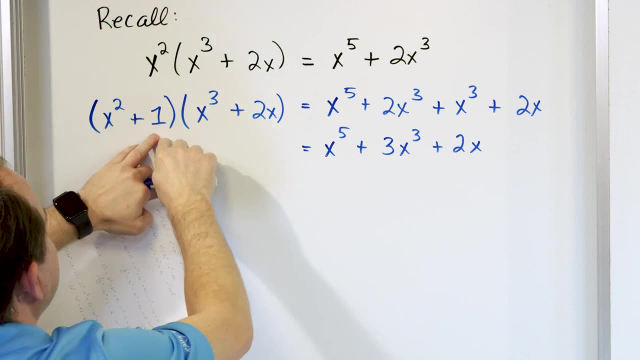 this one, and the last term are these two giving you this one. So think of it as FOIL, or what I like to say is think of it as covering this up, distribute this in, and then cover this up, distribute this in Basically everything on the. 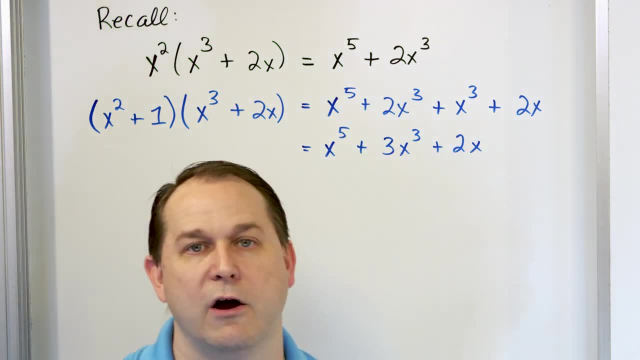 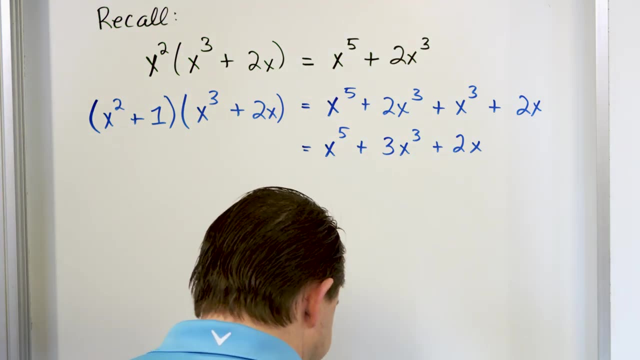 outside has to go in and multiply by everything on the inside. And the reason why I'm explaining to you that way is because in this lesson we're going to be multiplying more complex things than this. Let's say, for example: let's get to the material of today's lesson A little more complicated than 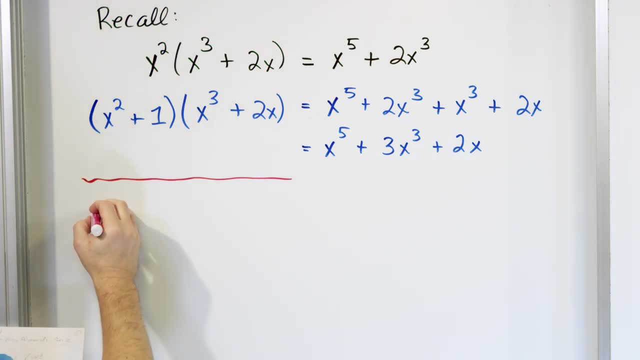 what we've done by extension. What if I have the same thing on the outside here? let's call it x squared plus 1 on the outside, but on the inside I change this and make it a little more complicated. x to the third power plus 2x, plus, let's. 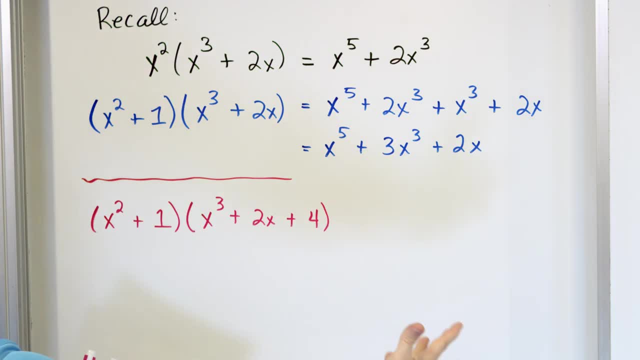 say plus 4.. Now, if you didn't learn it this way, then you might be very confused about how to handle that, because most students, when you're taught this, you learn binomial times, binomial, you learn FOIL, First outside inner, last First outside inner. 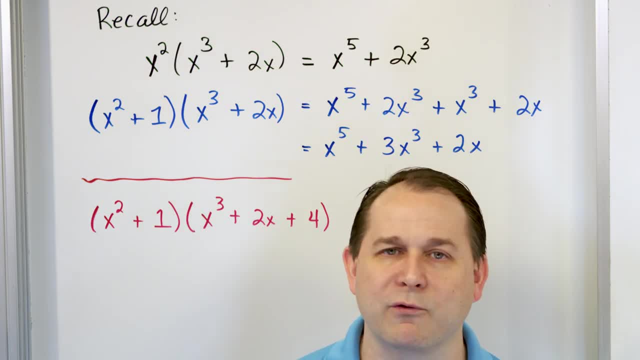 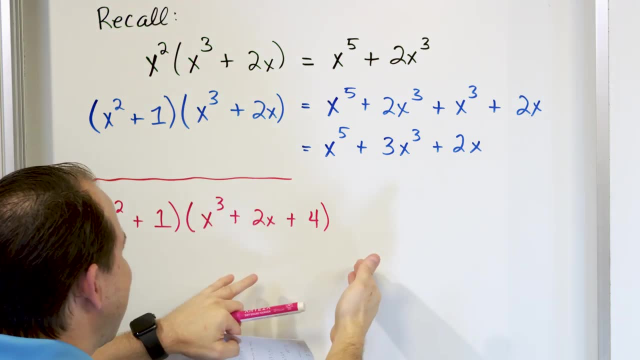 last. You just learn to do it right. But the problem is, if you just memorize FOIL, then you have no idea how to handle this because you don't know which are the first terms, which are the last terms. I mean, you might guess these are the last. 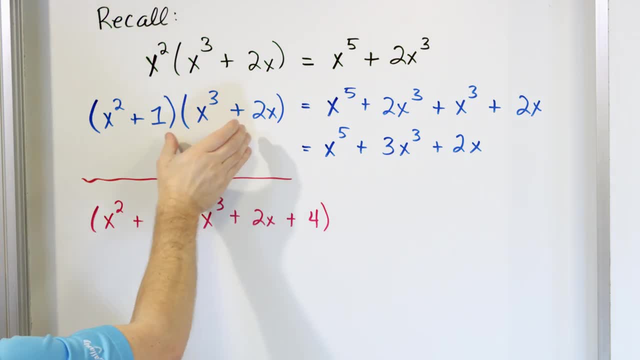 terms, but which ones are? the inside and the outer? because it doesn't match this cookie cutter thing. So that's why, this whole time I've been telling you, visualize it as x squared times this, these two terms separately, and then cover this and visualize it as these two terms. Why did I do that? Because now, 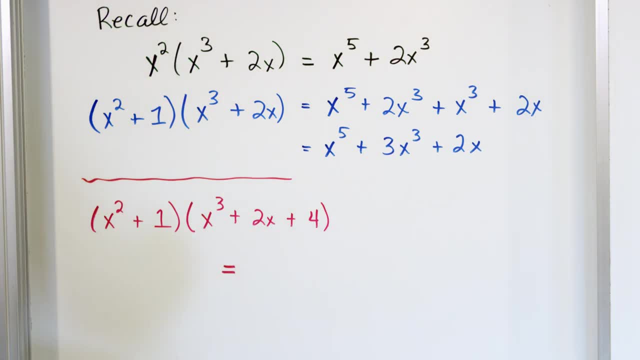 that we have a more complex problem. you don't memorize FOIL. What you do is you cover up the one and you pretend all you have is this: So these two terms multiplied together is x to the fifth power, and then again you. the one is not. 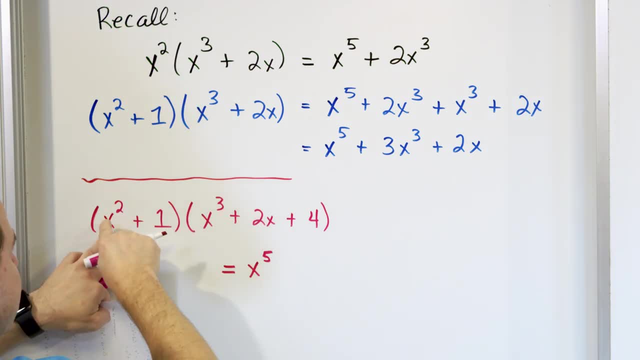 there. Then you distribute this one into this one. 2 times the, 2x times the x squared gives you 2x to the third power. We just add these exponents. Then you take this one and you go into the last one and you'll have 4 times the. 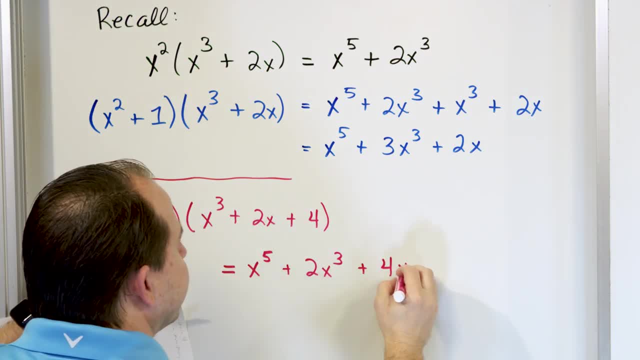 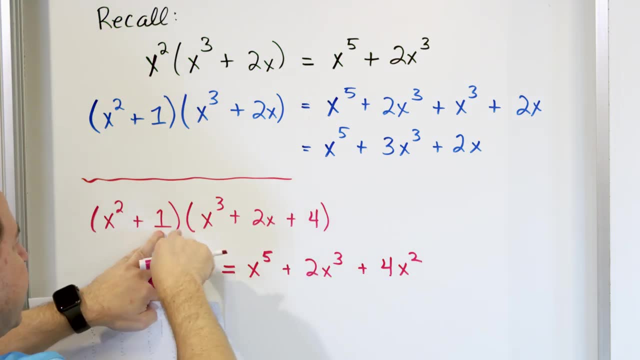 one gives you 4 and then x squared is right there. So you've completely distributed this outside term times everything. Now you cover them up, pretend he's not there. This term now needs to go in and distribute itself to everything inside. So 1 times x, cubed is going to be x. 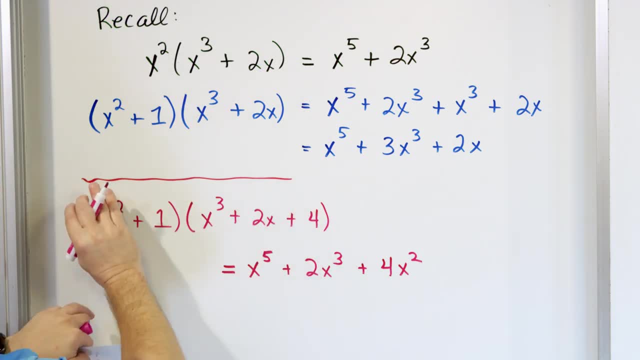 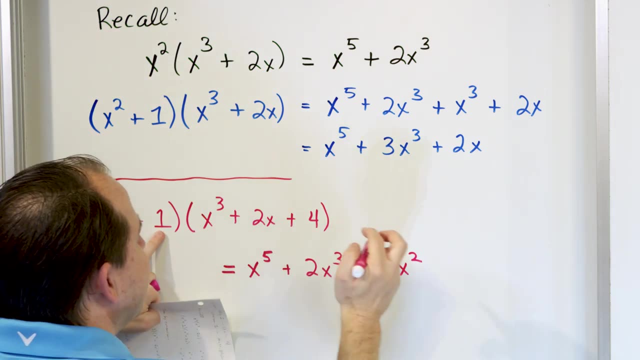 Now you've completely distributed this outside term times everything. Now you cover him up, pretend he's not there. This term now needs to go in and distribute itself to everything inside. So one times x cubed is going to be x cubed, One times 2x is going to just give. 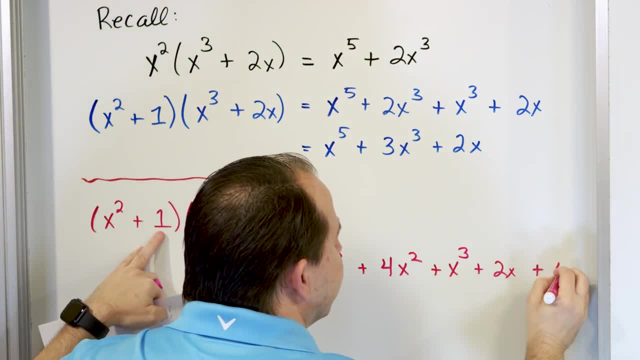 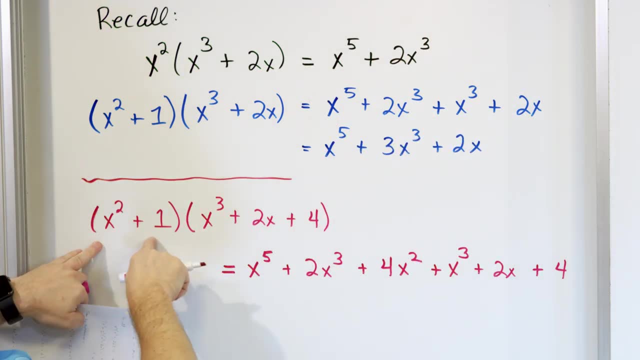 you 2x and one times four is just going to give you four. So you see how, in the case of the binomials, because of the number of terms, you had four terms in the answer. Because of this one, you have two times three, six terms in the. 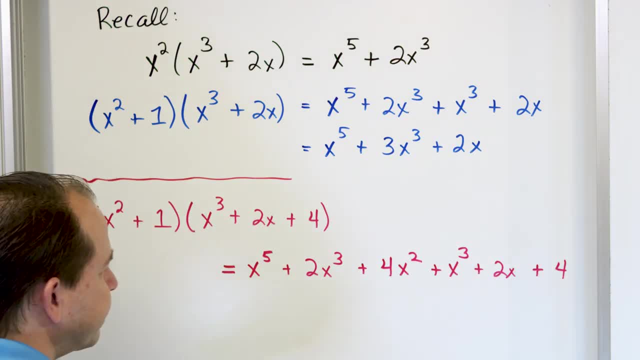 answer. So what we're going to do is that a lot of them are similar, right, Because you have 2x cubed and then you have x cubed right here, so that you can actually simplify these. So we're just going to look for same terms, see if we come across anything. 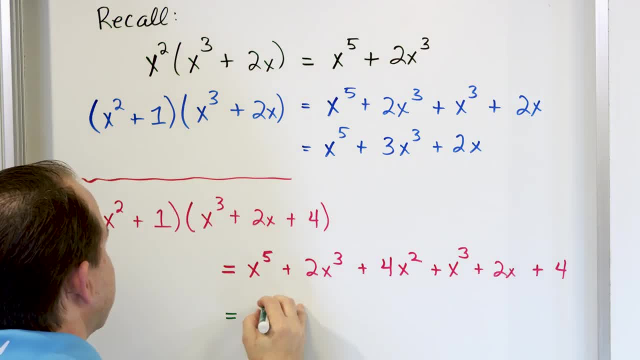 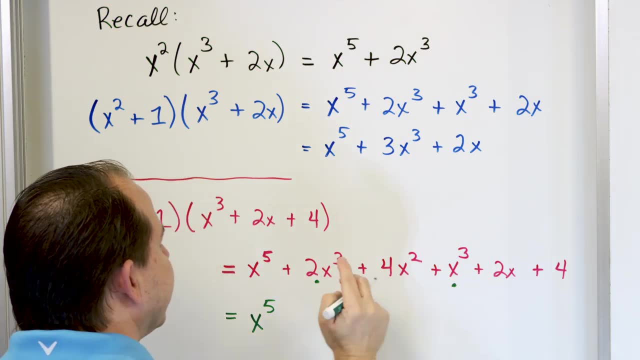 X to the fifth. we don't have any other x to the fifth terms, So this becomes the final term in the answer. Then we have this term matches this one, so we can add these together. Two plus one is three, Three. what Three x cubes? We have the 4x squared. We don't have 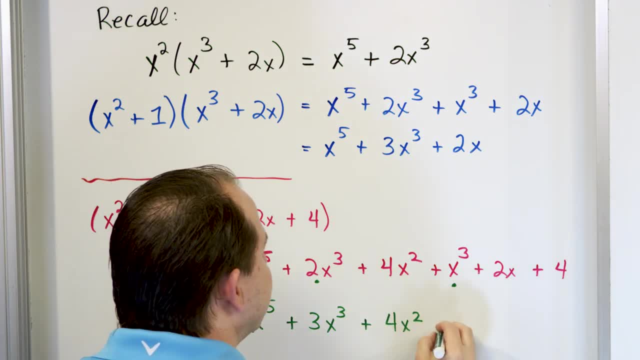 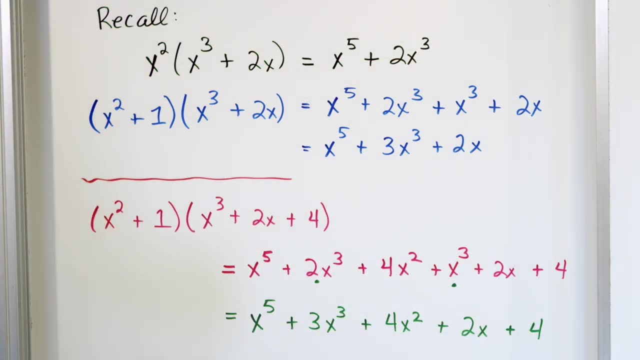 any other x squared terms. so we have 4x squared, And then we have the 2x- We don't have any other x terms- by itself- And then we have the constant four. We don't have any other numbers. So the final answer is x to the fifth plus 3x to the third, plus 4x squared plus 2x plus. 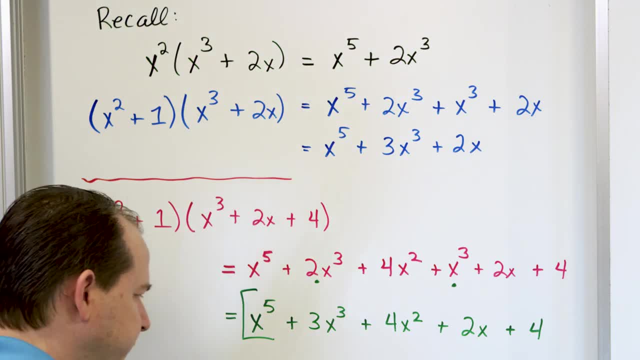 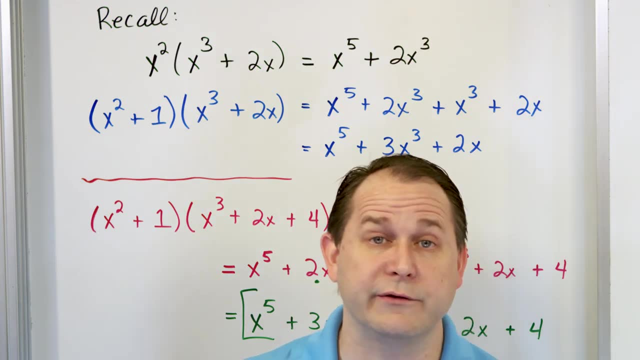 four, And this is the final answer, so you can circle this guy. If you really do understand what I've just done- and I've tried to break it down as simple and as step by step as I can- but if you understand this, then there will be no problem. I can give you that will. 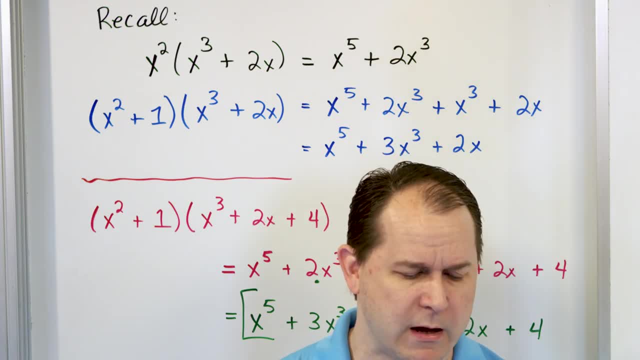 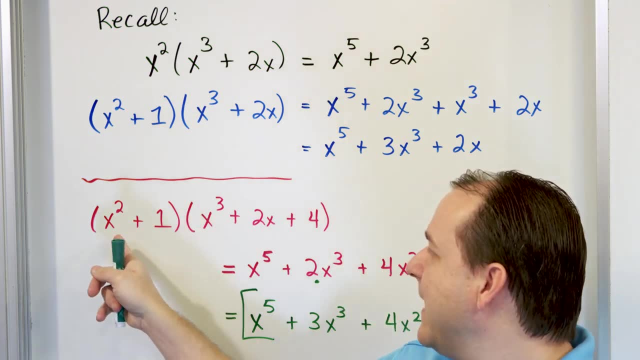 be actually hard. All of the problems that follow are going to basically be doing the same thing over and over again. for practice. The only thing is sometimes you have minus signs. See, I had every term in here was positive, so I didn't have any negatives to give me a chance. 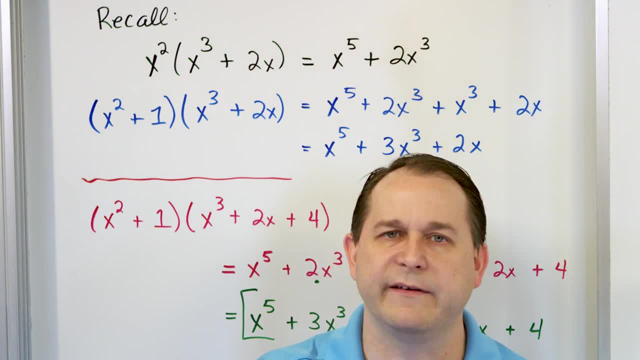 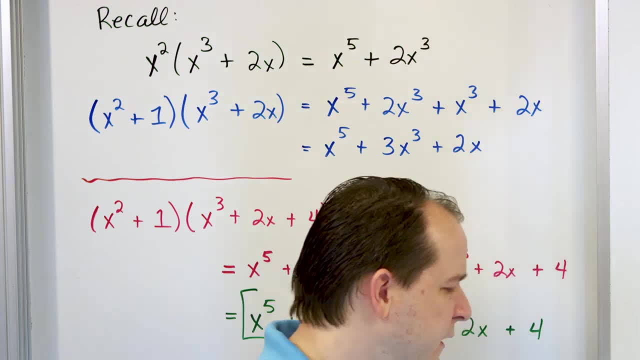 to make an error or whatever, But the point is that there's going to be more chances to make errors as I make the problems longer, but the process never, never changes. So let's go to the next example, just to kind of get a little more practice. 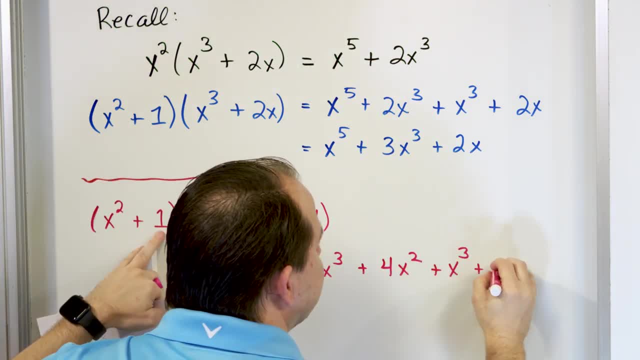 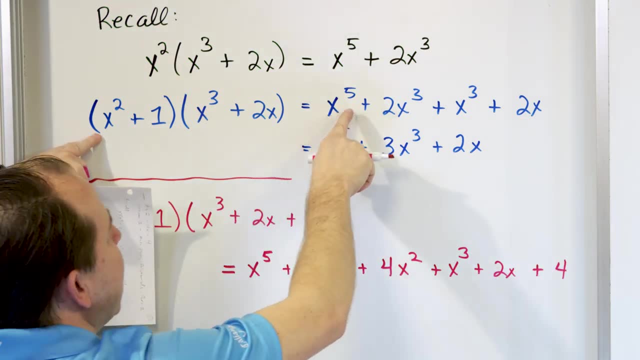 cubed, 1 times 2x is going to just give you 2x, and 1 times 4 is just going to give you 4.. So you see how, in the case of the binomials, because of the number of terms, you had four terms in the answer, Because of: 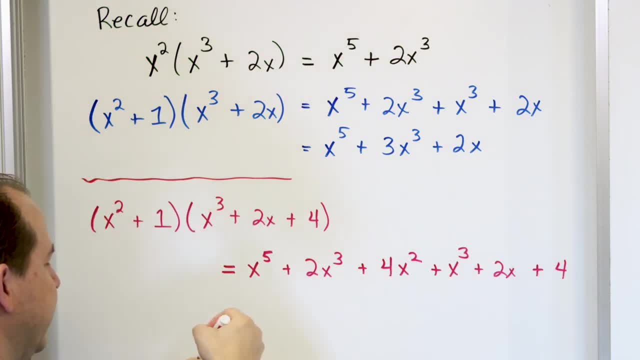 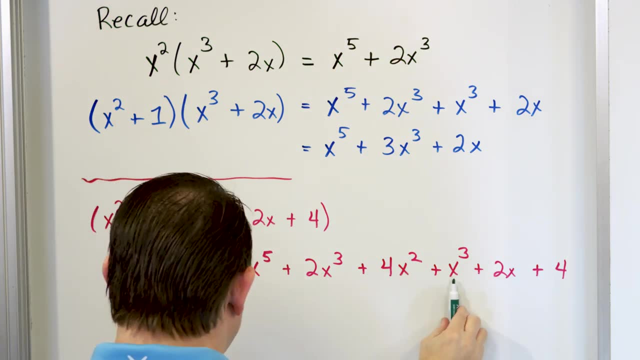 one. you have 2 times 3, 6 terms in the answer, But notice that a lot of them are similar, right? Because you have 2x cubed and then you have x cubed right here so that you can actually simplify these. So we're just going to look for same. 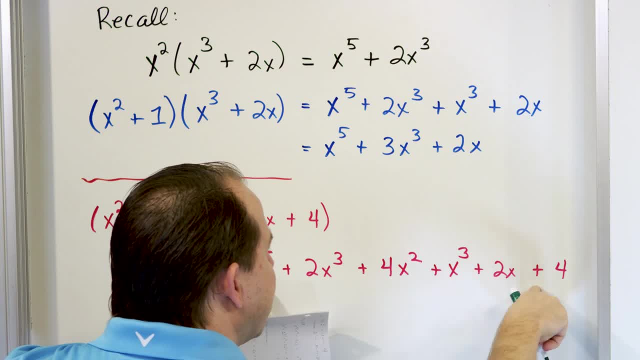 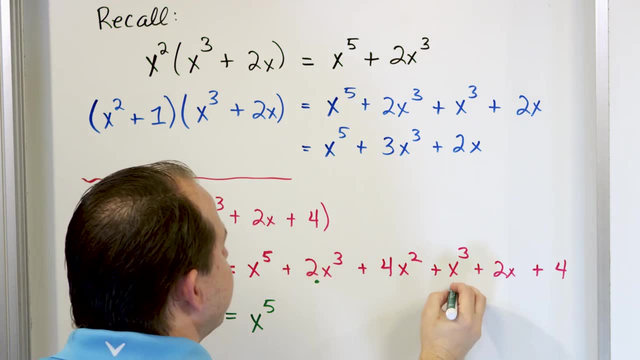 terms. See, if we come across anything x to the fifth, we don't have any other x to the fifth terms, So this becomes the final term in the answer. Then we have this term matches this one, so we can add these together: 2 plus 1 is 3.. 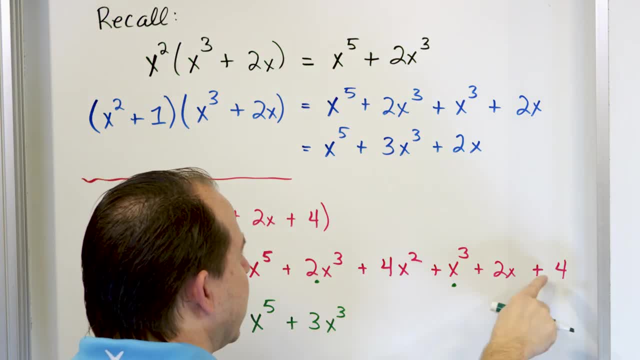 3. what 3x cubes. We have the 4x squared. We don't have any other x squared terms. We have 4x squared. And then we have the 2x. We don't have any other x terms by. 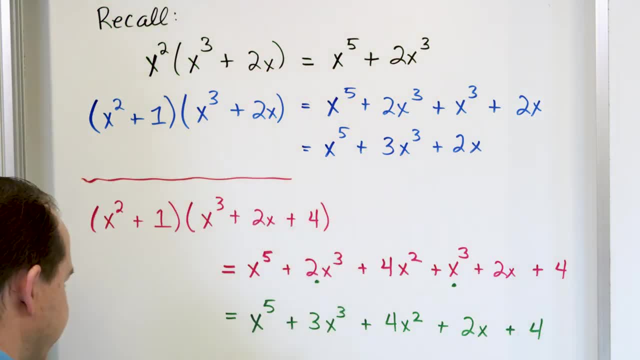 itself, And then we have the constant 4.. We don't have any other numbers. So the final answer is x to the fifth plus 3x to the third, plus 4x squared plus 2x plus 4.. And this is the final answer. so you can circle this guy, If you really do. 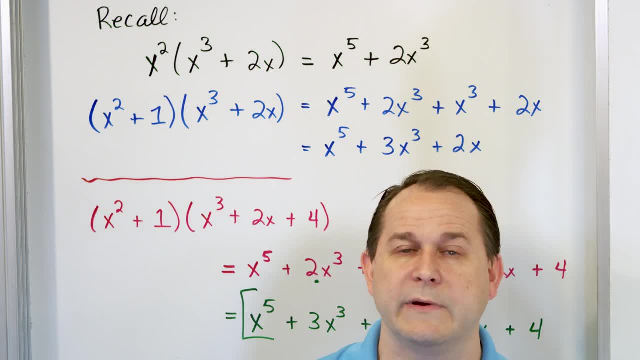 understand what I've just done and I've tried to break it down as simple and as step-by-step as I can. But if you understand this, then there will be no problem I can give you. that will be actually hard. All of the problems that follow are going to basically be doing the same thing over. 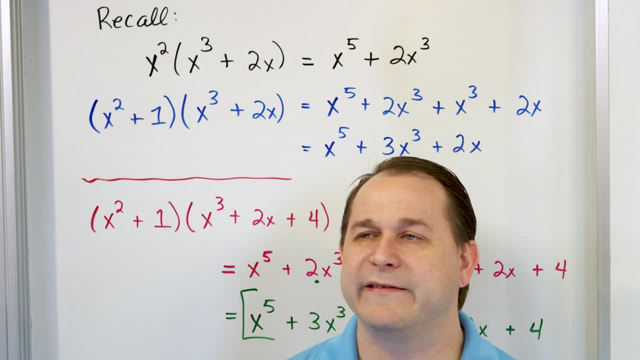 and over again for practice. The only thing is sometimes you have minus signs. See, I had every term in here was positive, so I didn't have any negatives to give me a chance to make an error or whatever. But the point is is that there's going to be more chances to make errors as I make the problems. 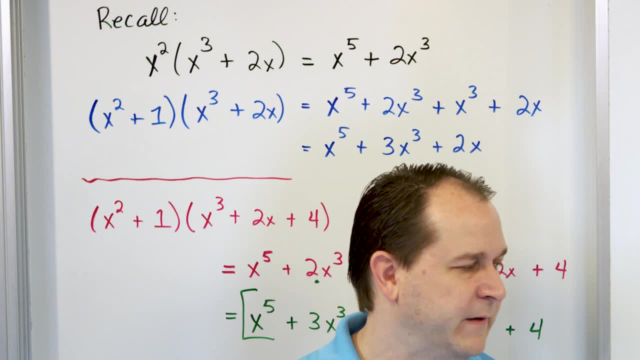 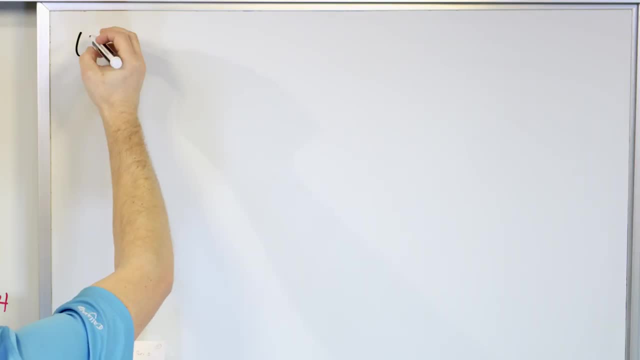 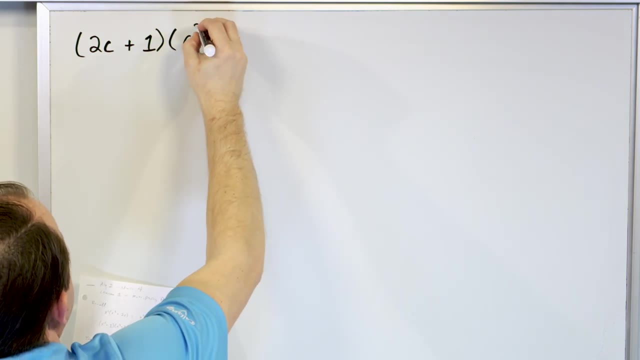 longer, but the process never, never changes. So let's go to the next example. Just to kind of get a little more practice. What if we had the example 2 times c plus 1? and I'm multiplying that, binomial times c, squared minus 3 times c. 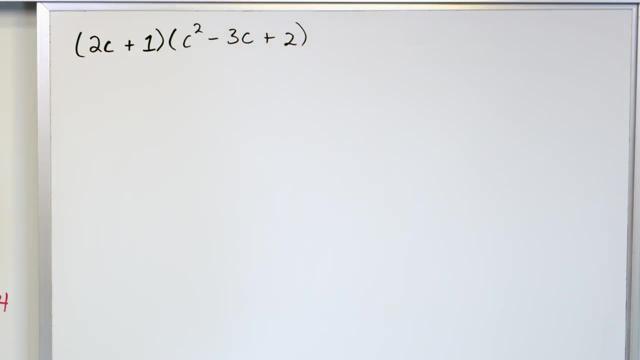 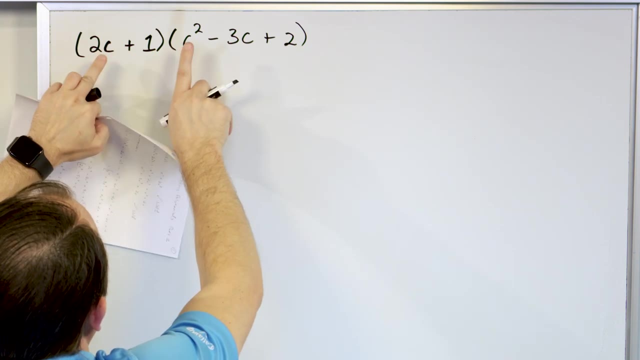 plus 2.. Alright, so again I pretend the 1 is not there and I distribute this into each term separately. So the first terms, and I do encourage you on your paper, put your fingers on there to help you keep track of it: 2c times c squared. 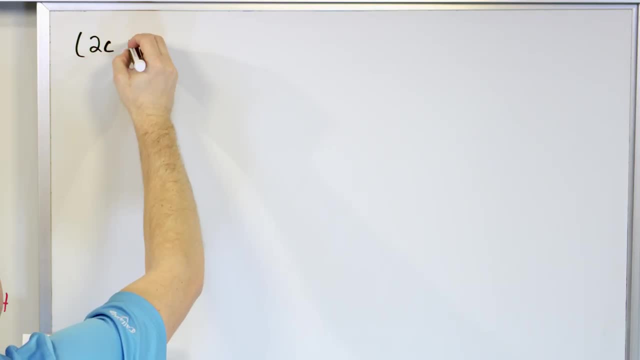 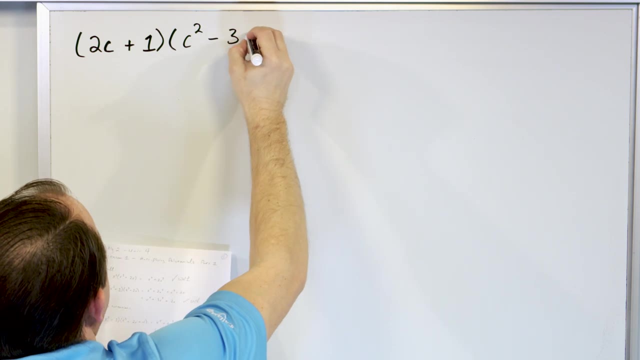 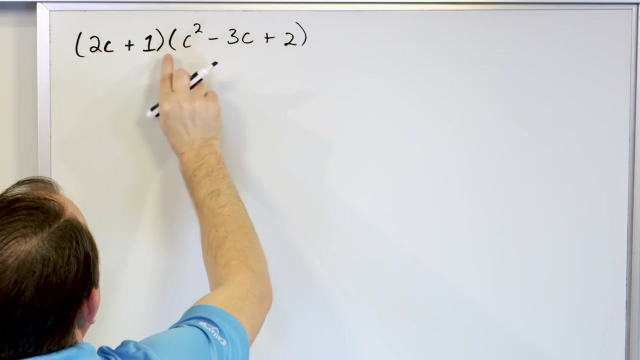 What if we had the example 2 times c plus 1, and I'm multiplying that binomial times c, squared minus 3 times c plus 2.. All right, so again I pretend the 1 is not there and I distribute this. 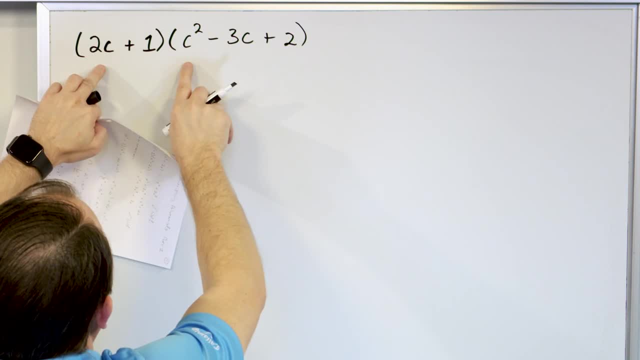 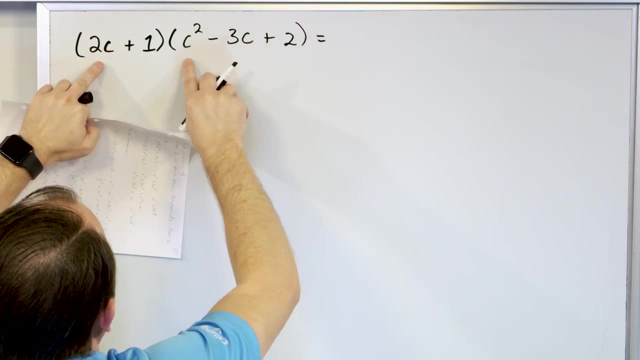 into each term separately. So the first terms, and I do encourage you on your paper, put your fingers on there to help you keep track of it: 2c times c squared is going to give you what You're going to have: 2c cubed, because you're just going to add the exponents of the c variable. Then this: 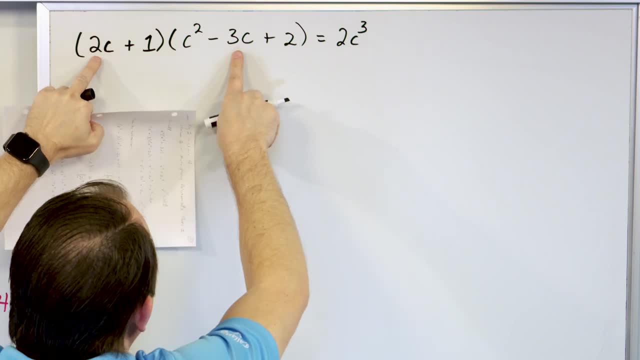 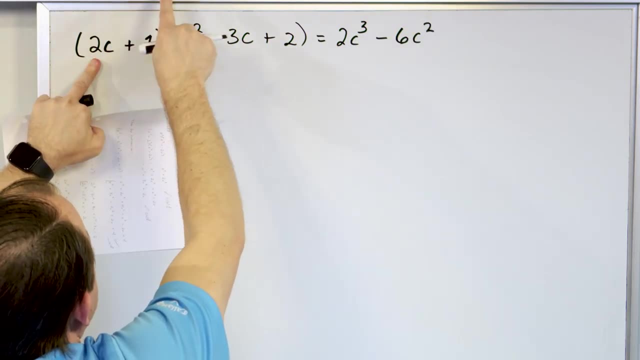 one gets multiplied in but it's times negative 3. now Negative 3 times 2 is negative 6.. So the negative 6 is here and the c times the c is c squared. Then you take this one and go times the. 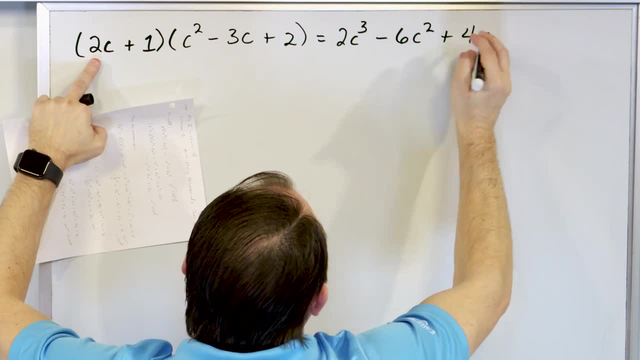 2. 2 times 2 is 4, positive 4, times c, because, don't forget, I have a c right here and there's no c here, so it has to come along for the ride. Now. I've kind of run out of space here, so I'm. 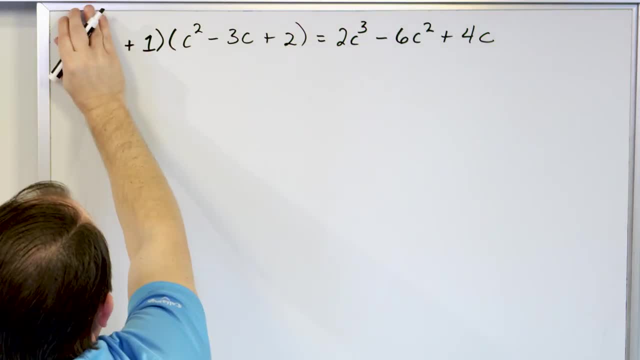 just going to continue on the next line, but now I'm going to pretend that I have a c here and the 2c is not there at all. 1 times c will be positive, or I should say 1 times c squared will. 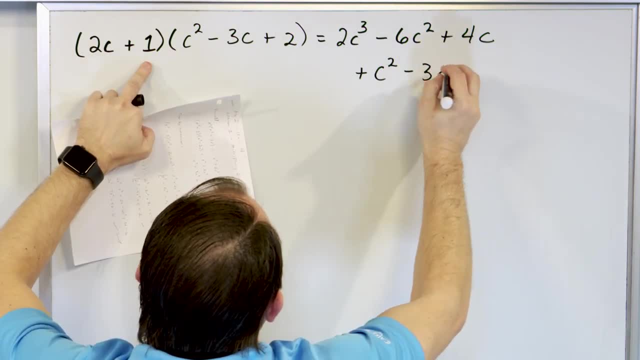 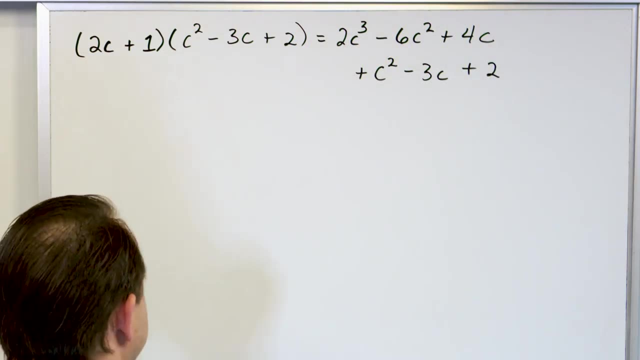 be c squared 1 times the negative, 3c is negative. 3c 1 times 2 is 2.. So I have all of this stuff plus this stuff, and then all I have to do is simplify terms. So 2c cubed, I don't have any. 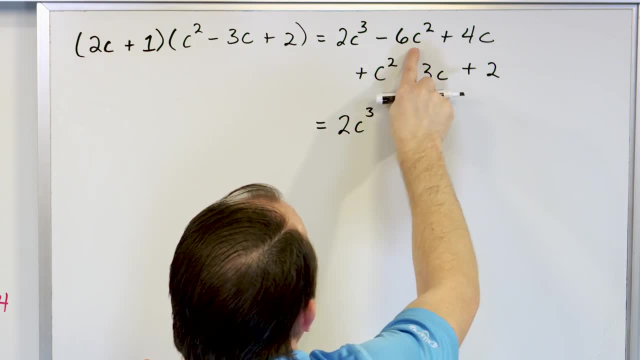 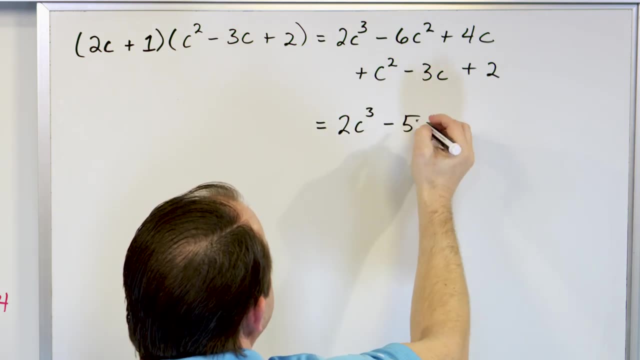 other c cubes. so that stays in the answer: c squared. here's the only other c squared I have. so negative 6 plus a positive 1.. What's negative 6 plus positive 1? It's negative 5.. 5, what 5c squares? So this term, this term and this term are already taken care of. Now the 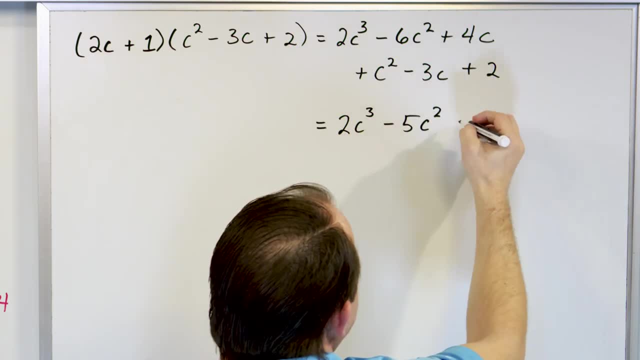 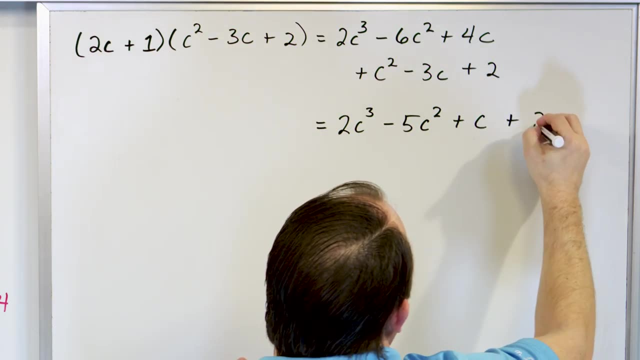 4 plus the negative 3, or you can think of it as 4 minus 3, is just going to be 1, and 1, what 1c? You don't have to put the 1 in front there. And then I have a constant of 2 there, no other. 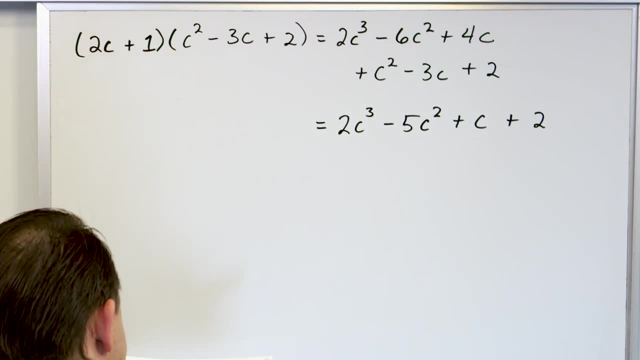 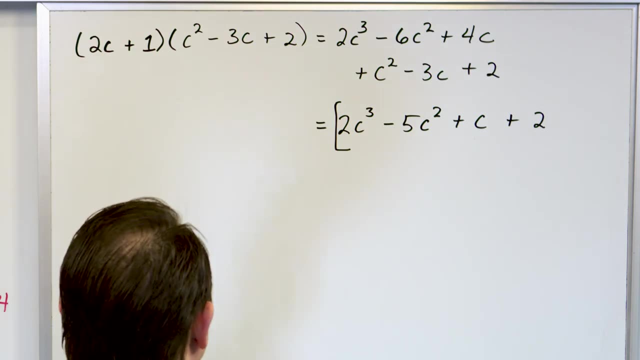 constants in my answer. So I get 2c cubed minus 5c squared plus c plus 2.. This is the final answer. So every other problem that we're going to do in this lesson is going to be very, very similar. 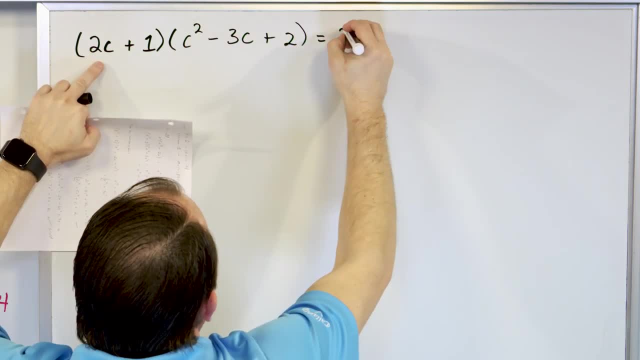 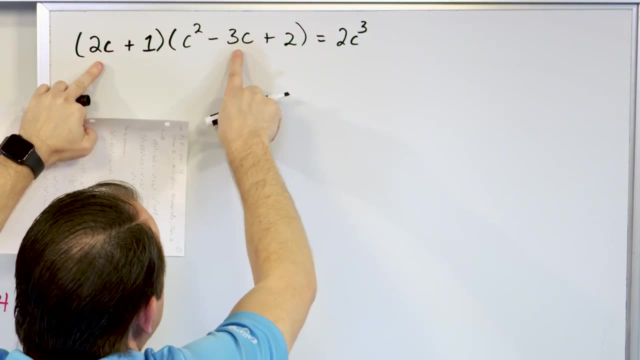 is going to give you what You're going to have 2c cubed, because you're just going to add the exponents of the c variable. Then this one gets multiplied in, but it's times negative 3 now Negative 3 times 2 is negative 6.. So the 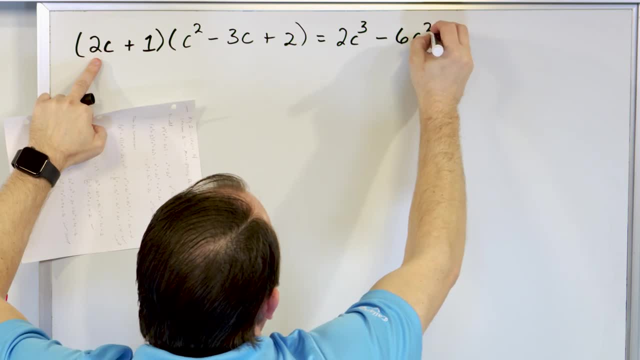 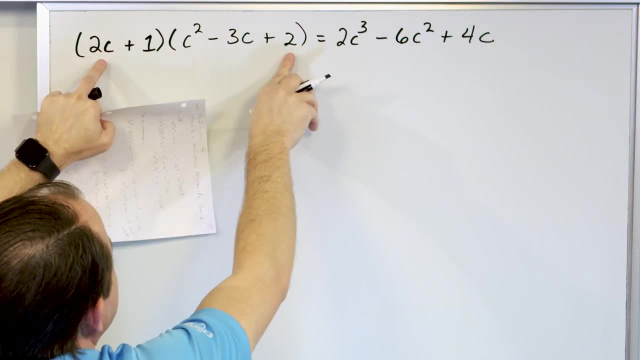 negative: 6 is here and the c times the c is c squared. Then you take this one and go, times the 2.. 2 times 2 is 4.. Positive: 4 times c. because, don't forget, I have a c right here and there's no c here, so it has to come along for the ride Now. I've 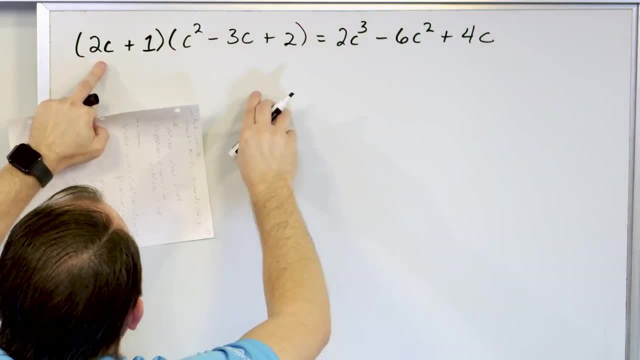 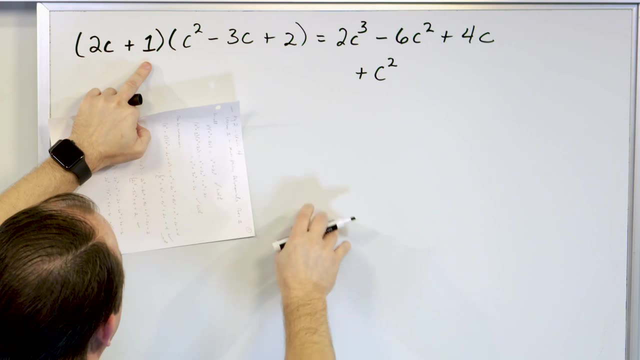 kind of run out of space here, so I'm just going to continue on the next line. but now I'm going to pretend the 2c is not there at all. 1 times c will be positive, or I should say 1 times c squared will be c squared 1. 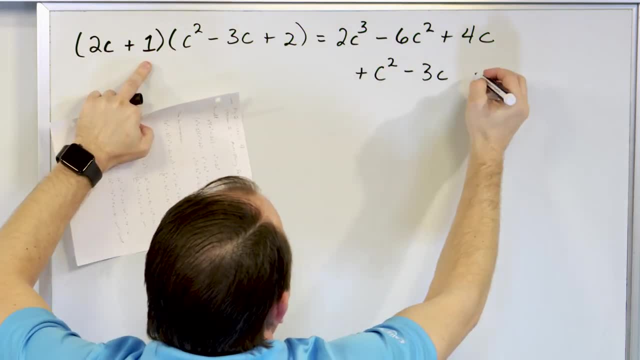 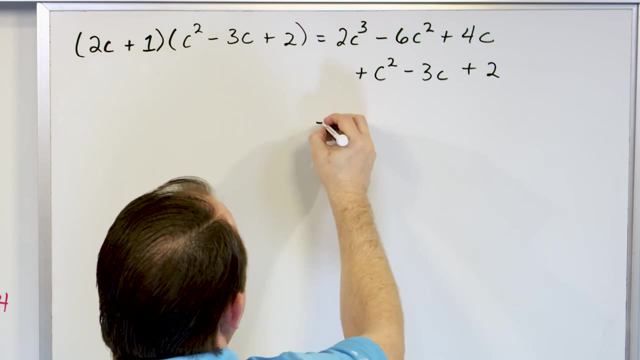 times the negative. 3c is negative. 3c. 1 times 2 is 2.. So I have all of this stuff plus this stuff, and then all I have to do is simplify terms. So 2c cubed- I don't have any other c cubes, so that stays in the answer: c squared. here's the. 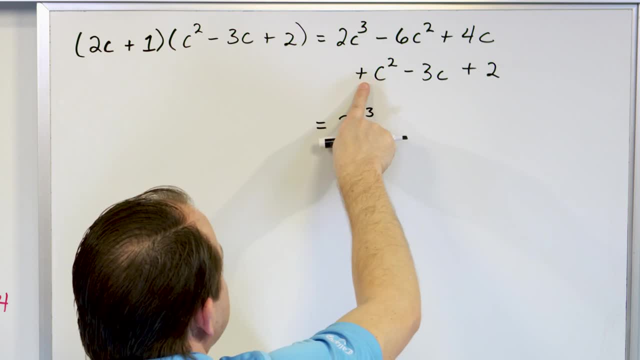 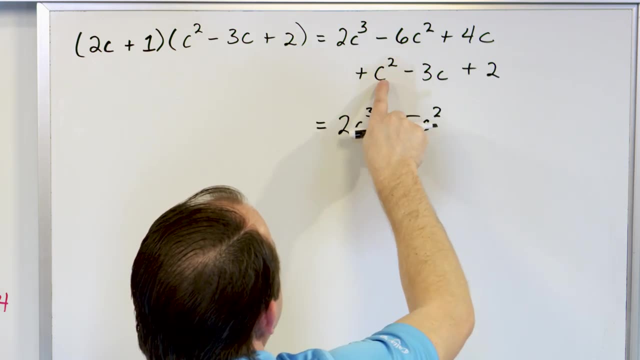 only other c squared. I have So negative 6 plus a positive 1.. What's negative? 6 plus positive 1 is negative 5.. 5, what 5c squares? So this term, this term and this term are already taken care of. Now the 4 plus the negative 3, or you can. 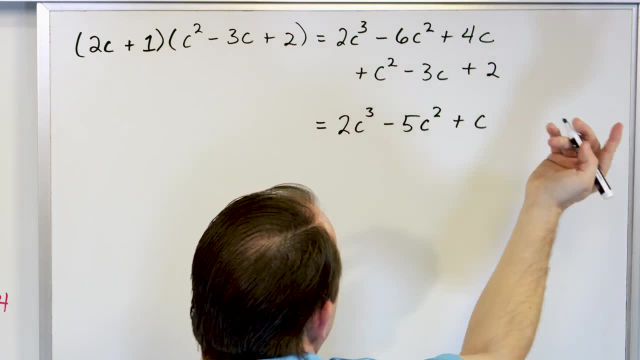 think of it as 4 minus 3 is just going to be 1 and 1. what 1c? You don't have to put the 1 in front there, And then I have a constant of 2. There are no other. 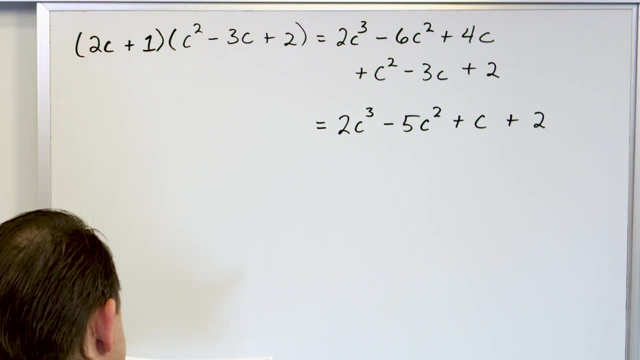 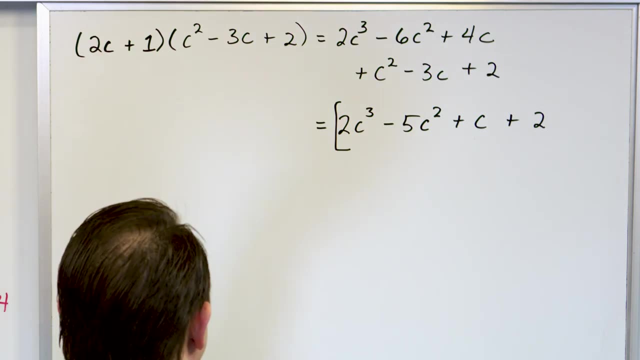 constants in my answer. So I get 2c cubed minus 5c squared plus c plus 2.. This is the final answer. So every other problem that we're going to do in this lesson is very similar, but we're just going to have slightly more complex scenarios here, For 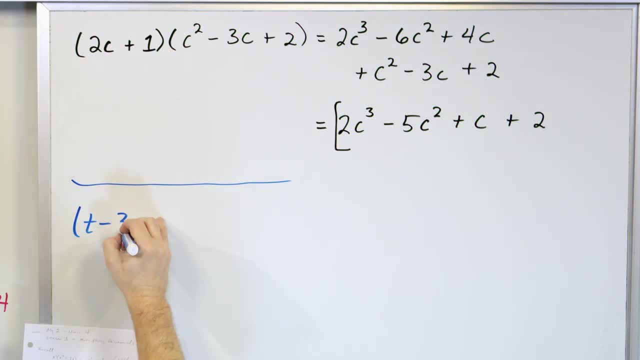 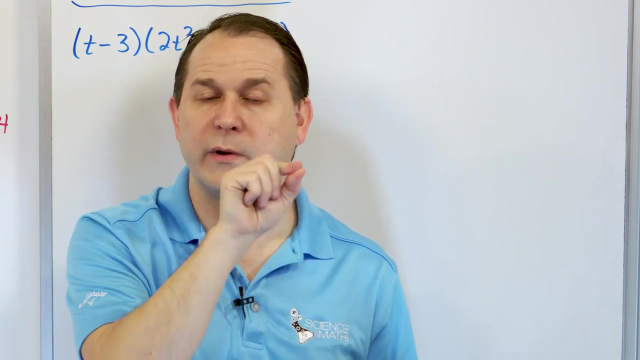 instance, what if we have t minus 3? 2t squared minus t plus 2.. Now the only thing that makes this tricky is I have a minus sign here and a minus sign there. So as I do my distribution, I do need to be careful when I multiply negatives and positives to get the right signs. 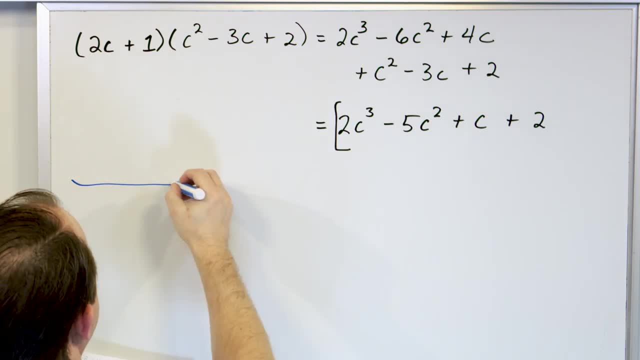 but we're just going to have slightly more complex scenarios here. For instance, what if we have t minus 3? 2t squared minus t plus 2.. Now, the only thing that makes this tricky is I have a minus sign here and a minus sign there. So, as I do my distribution, I do need to be careful when 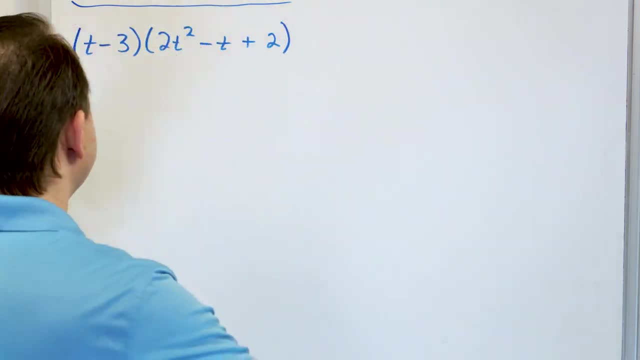 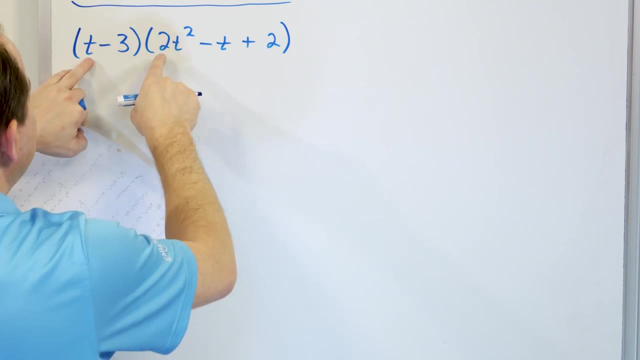 I multiply negatives and positives to get the right signs. So what I'm going to do, instead of doing it this way, I'm going to write my equal sign underneath so I can fit everything on one line. So what do I have? t times the first term, which is 2t, squared. 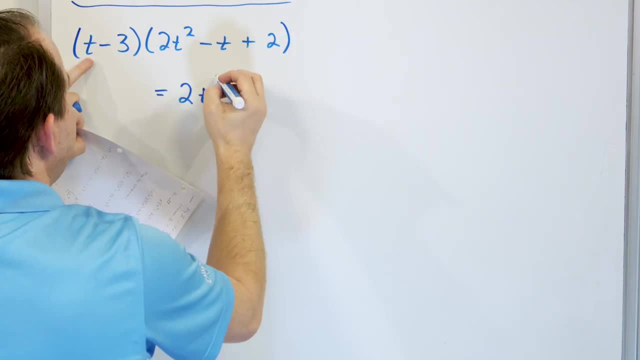 will give you 2.. 2 times 1 is 2.. And then you get the t's and you add those exponents together, giving you t cubed. Then this one times this one, This is negative. So negative 1 times the. 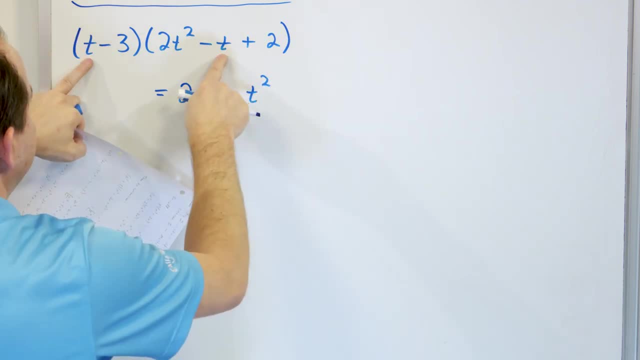 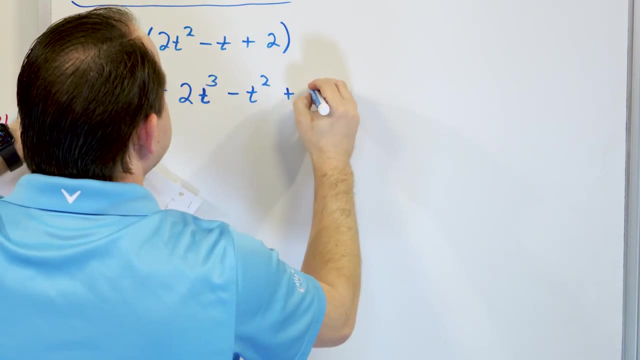 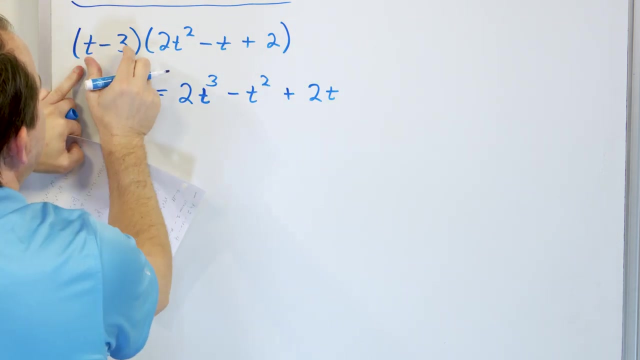 positive gives you negative t squared. I add these exponents together: t times the 2 here is going to give you 2 times t. Right Now, I've done that. I've distributed that into every term. Now I cover this up and pretend I have only the second one outside, But that negative. 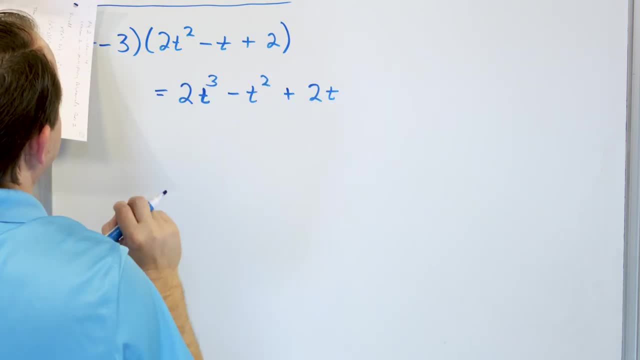 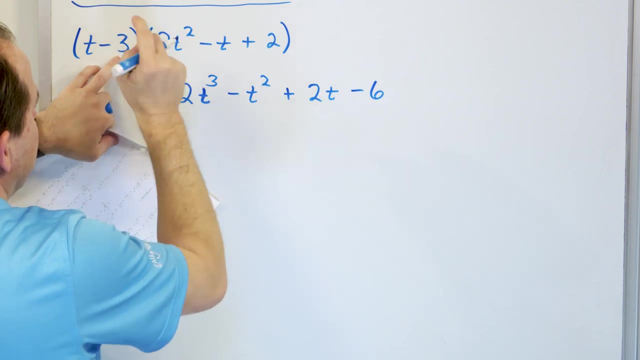 sign is still there. So when I distribute this in, it's negative 3 times each of these guys. So what's this one going to be Negative 3 times positive. 2 gives me negative 6.. t squared times: nothing. there is just going to give you the t squared Right, Then negative 3 times negative. 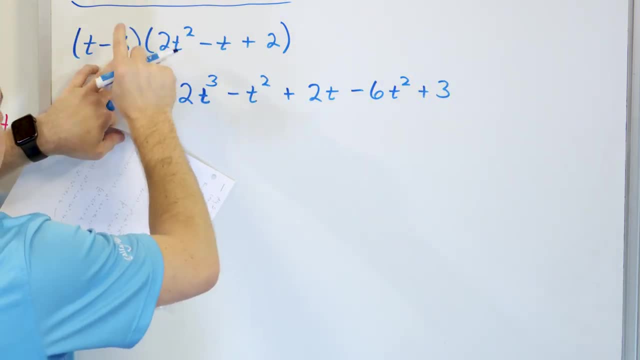 1 gives me positive 3. And then the t goes with. there's nothing else there, So the t is just coming along for the ride. Then negative 3 times the positive 2 gives me negative 6. That's the term. So then I start looking for similar terms or like terms. So this one, there are no other t. 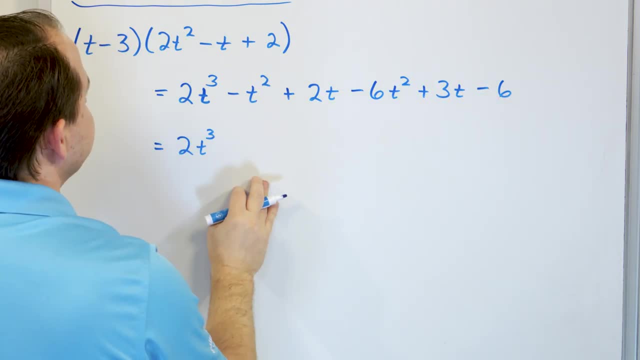 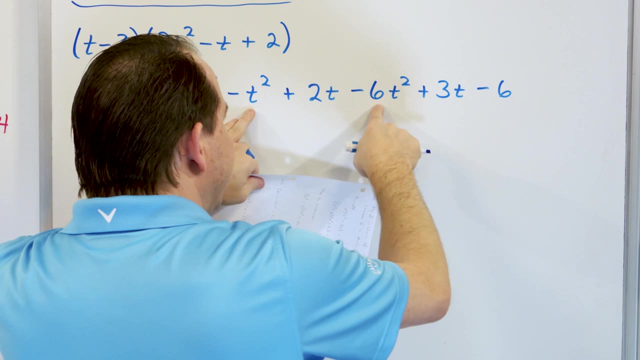 cubes anywhere. So I say 2t to the third power. So that takes care of this term. Then I have t squared. This is the only other t squared here. What's minus 1 plus a negative 6?? Or you can think. 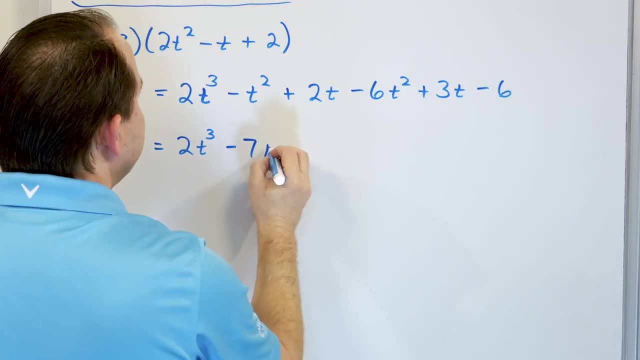 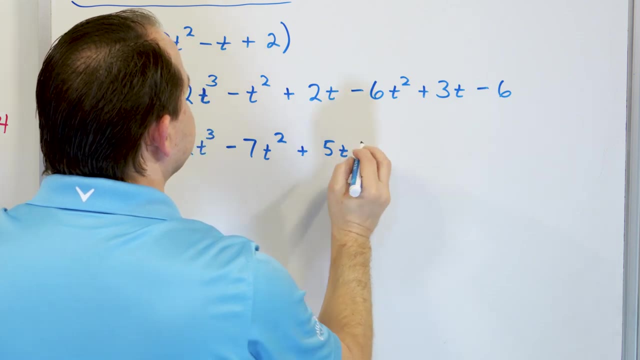 of it as negative: 1 minus 6.. That's going to give you negative 7 t squared. Then I have this term and this term. These are similar. 2 plus 3 is 5. t Right, And then the only thing left in the answer: 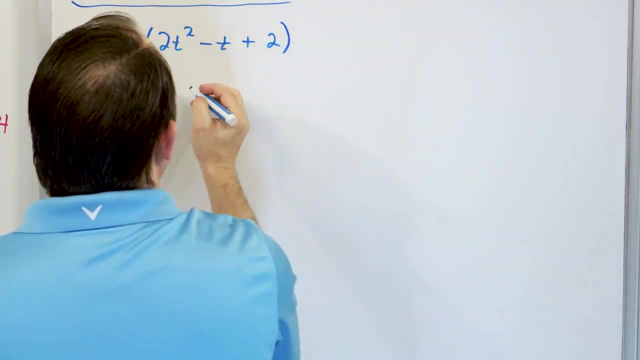 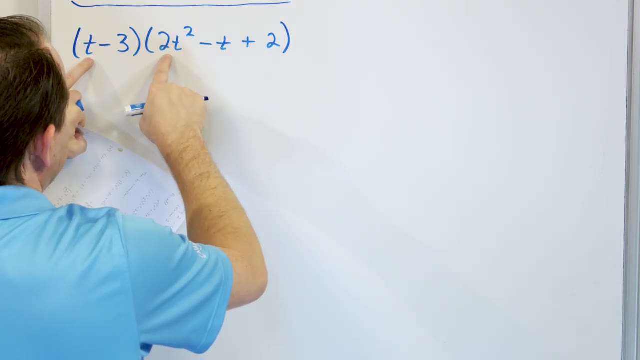 So what I'm going to do, instead of doing it this way, I'm going to write my equal sign underneath, so I can fit everything on one line. So what do I have? t times the first term, which is 2t squared, will give you 2.. 2 times 1 is 2.. And then you get the t's and you add: 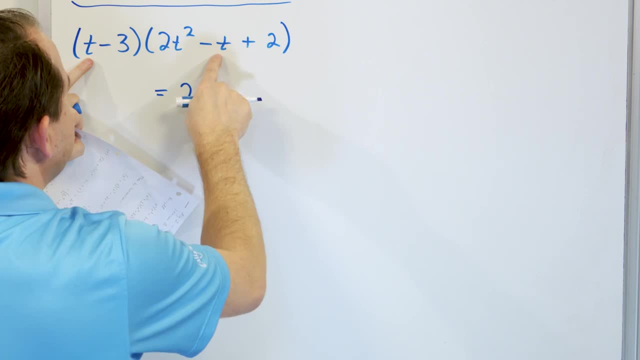 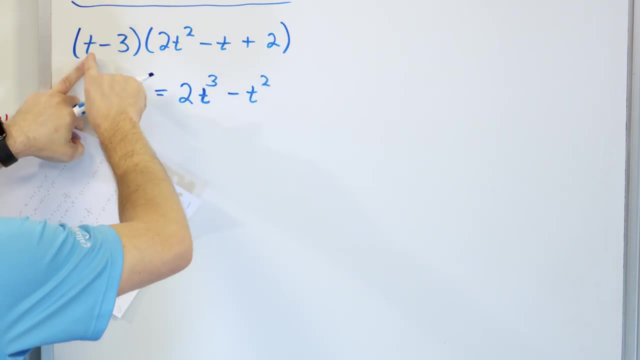 those exponents together, giving you t cubed. Then this one times this one. This is negative, So negative 1 times the positive gives you negative t squared. I add these exponents together: t times the 2 here is going to give you. 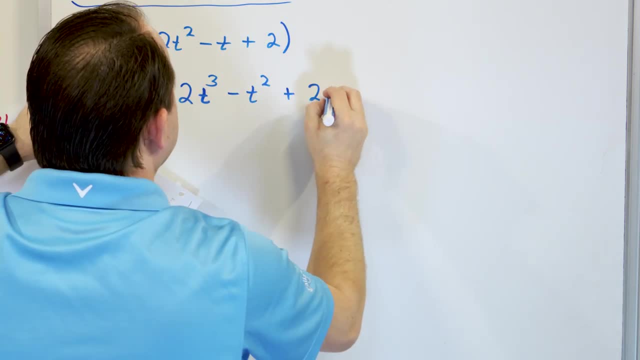 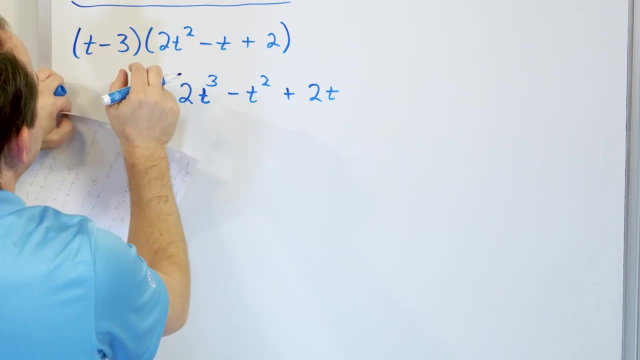 2t squared 2 times t. right Now, I've done that, I've distributed that into every term. Now I cover this up and pretend I have only the second one outside, But that negative sign is still there. 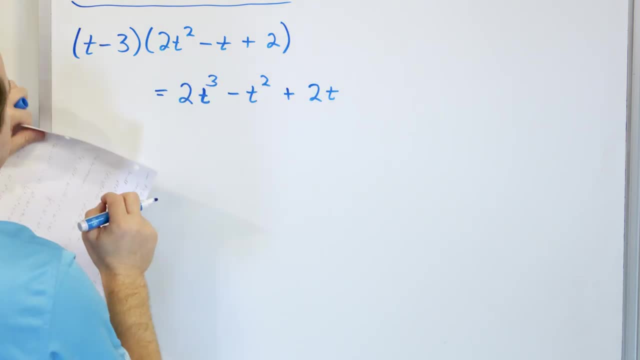 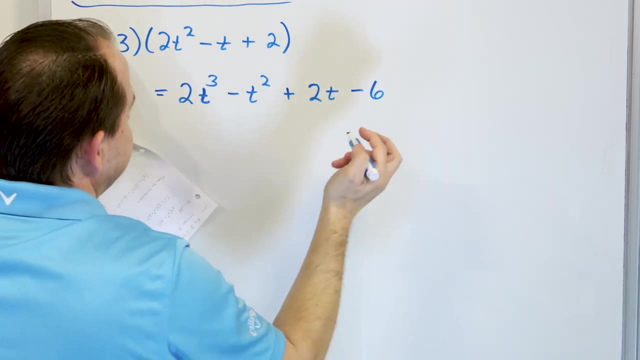 So when I distribute this in, it's negative 3 times each of these guys. So what's this one going to be? Negative 3 times positive. 2 gives me negative 6.. t squared times: nothing. there is just going to give you the t squared right. Then, negative 3 times negative. 1 gives me positive 3.. 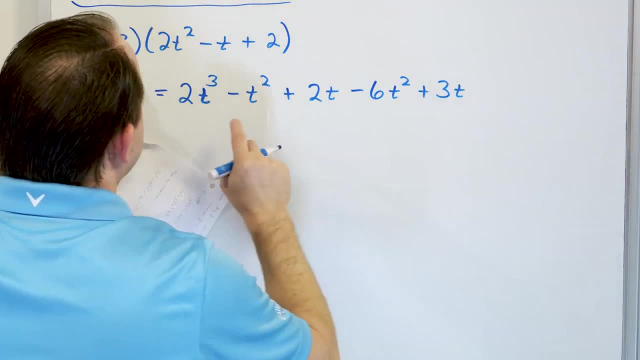 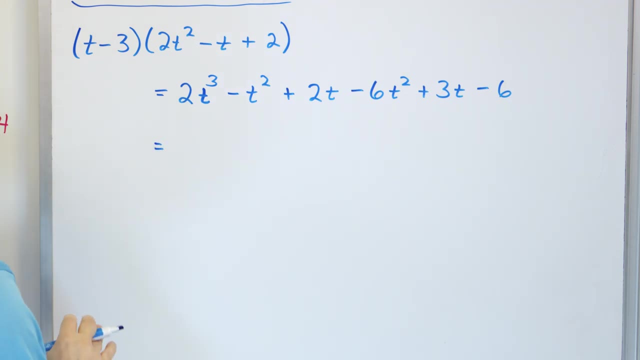 And then the t goes with. there's nothing, Nothing else there, So the t is just coming along for the ride. Then negative 3 times positive 2 gives me negative 6. That's the constant term. So then I start looking for similar terms or like terms. 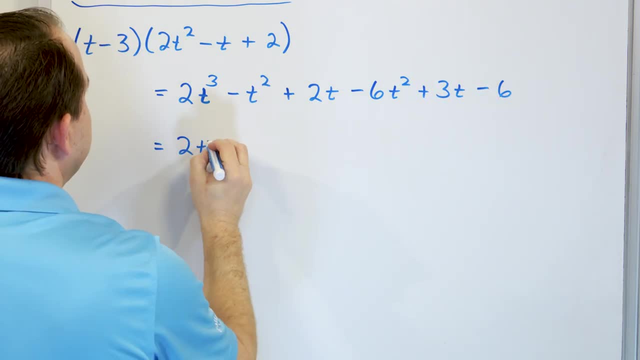 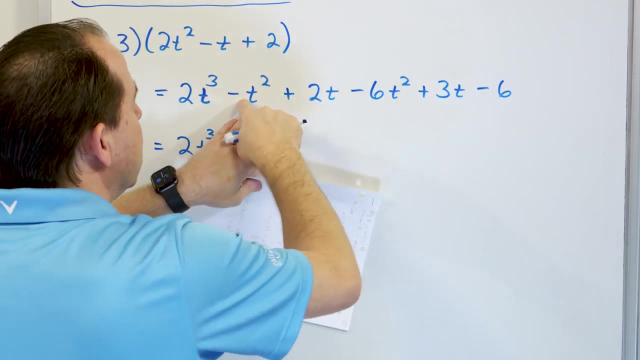 So this one. there are no other t cubes anywhere. So I say 2t to the third power. So that takes care of this term. Then I have t squared. This is the only other t squared here. What's minus 1? 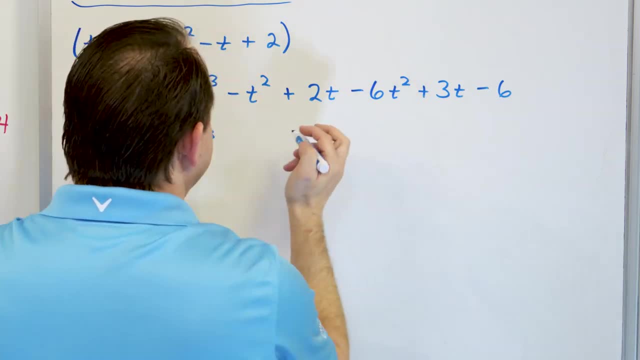 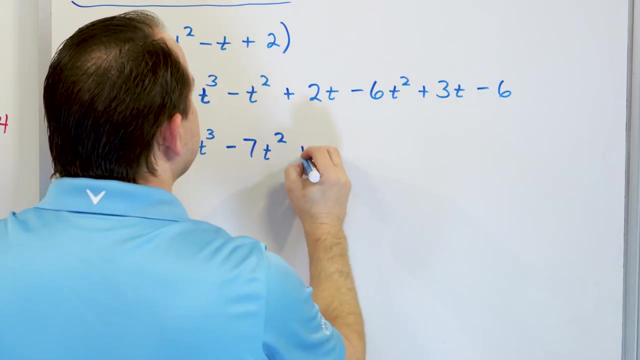 plus a negative 6?? Or you can think of it as negative 1 minus 6.. That's going to give you negative 7 t squared. Then I have this term and this term. These are similar. 2 plus 3 is 5t, right, And then the only thing left in the answer is negative 6.. This is the 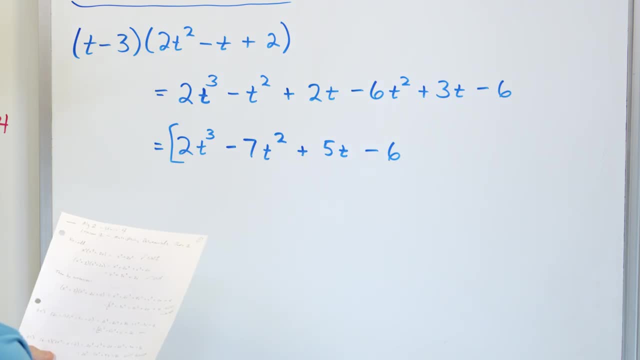 final answer. Let's double check: 2t cubed minus 7t squared plus 5t minus 6.. And that's correct. So I hope you're starting to get some familiarity for how we're doing this. I cannot stress how important it is to master the skill, though, because 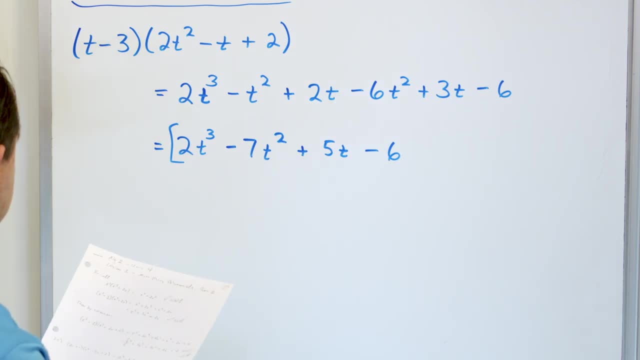 is negative 6.. This is the final answer. Let's double check: 2t cubed minus 7t squared plus 5t minus 6. And that's correct. So I hope you're starting to get some familiarity for how we're. 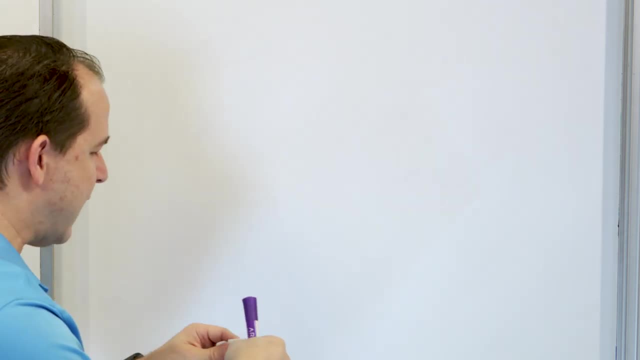 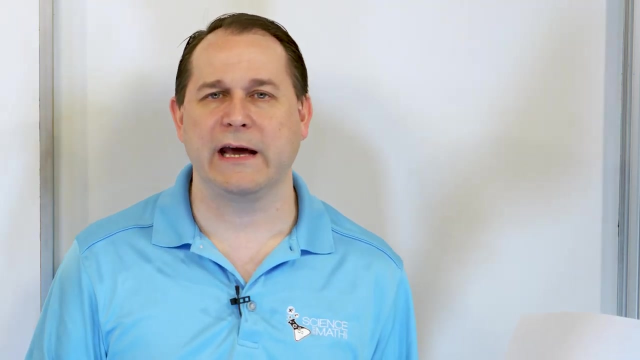 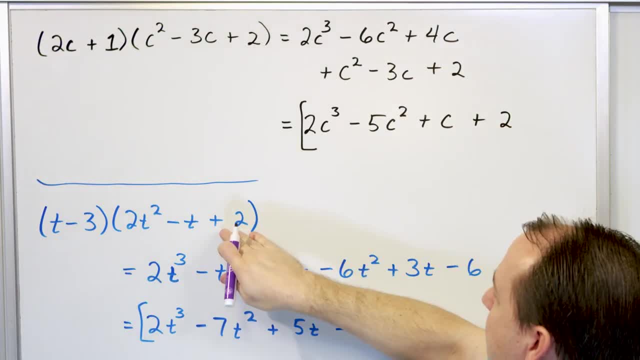 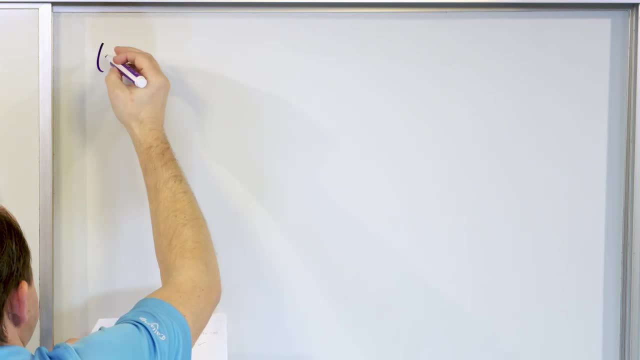 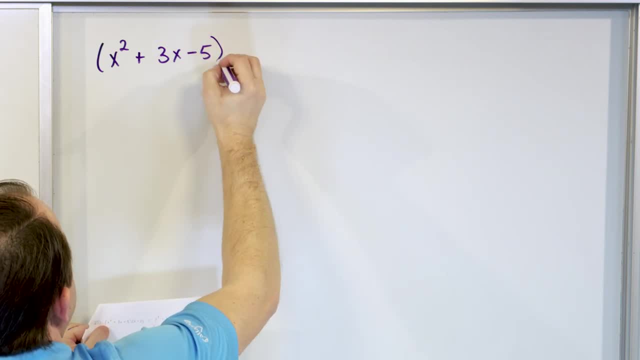 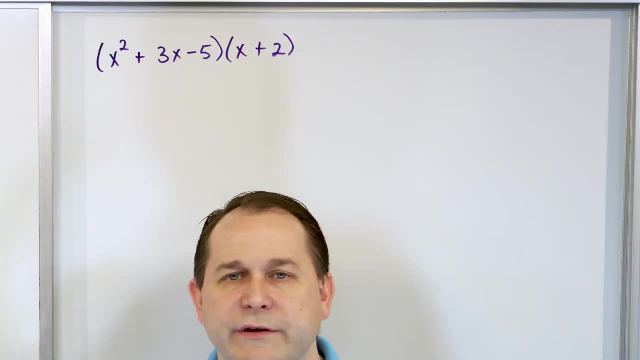 plus 3x minus 5? And then I'm multiplying that times x plus 2.. Now see, if you're just memorizing things like FOIL F-O-I-L, not only do you not know how to do the last type of problem, 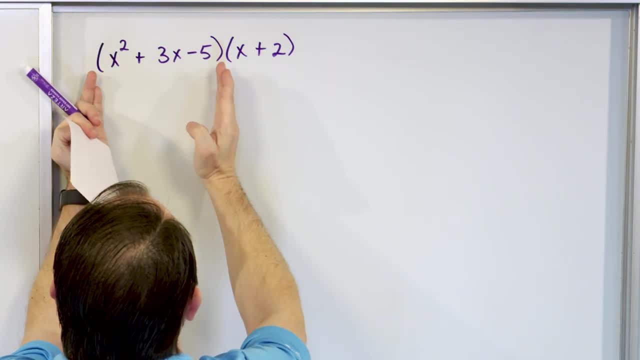 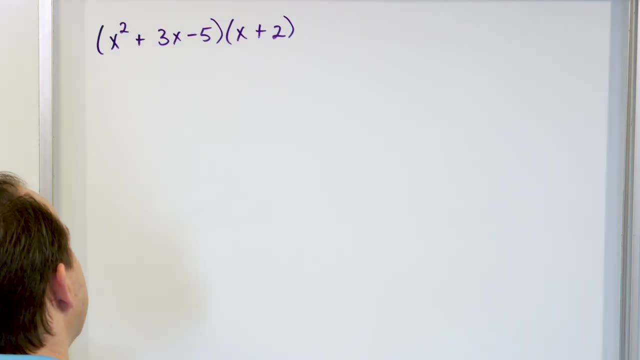 but you don't know how to do this one, because what's in front is actually three terms Multiplied by two terms. So it differs even more than in the past. But now you know you're not going to fall for that. All you have to do to multiply. this is every one of these terms has. 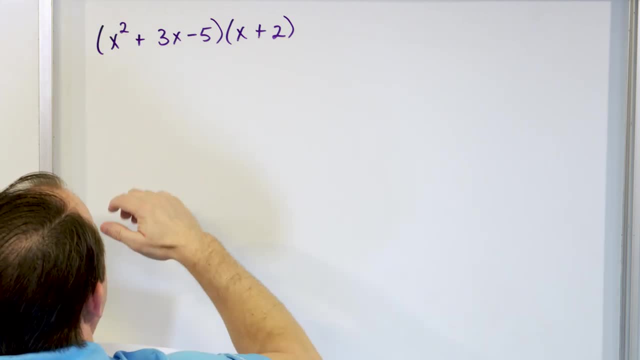 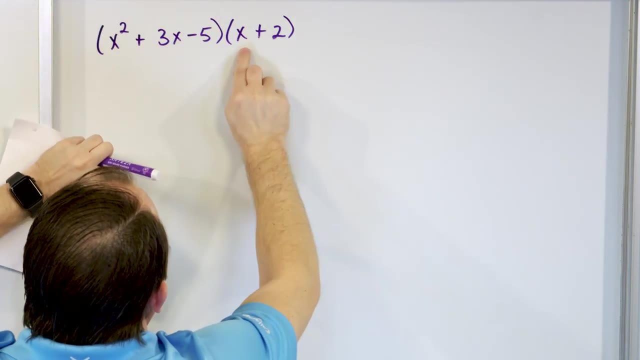 to individually go in and multiply times everything over here. So what you do is you cover both of these up, Pretend they're not there. This has to be multiplied in by those terms, Then you cover both of these. This one has to then be multiplied by both terms, Then you cover both. 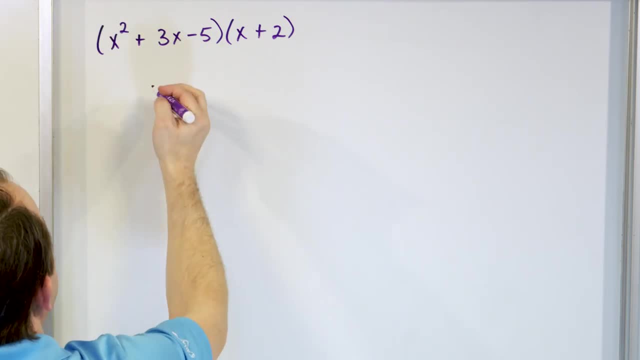 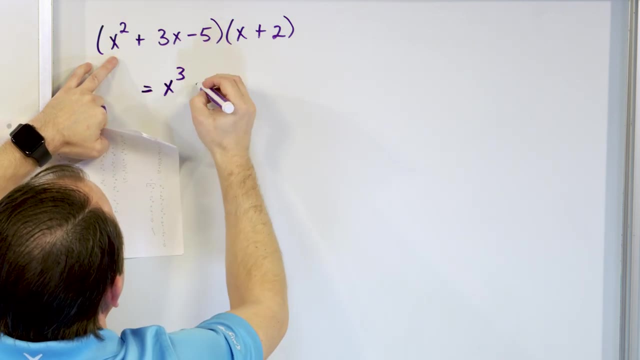 of these, This one has to go in and multiply by both terms. So what you have is: what is x squared times x? You're going to get x to the third. Add the x immersed So that x squared times 2 is going. 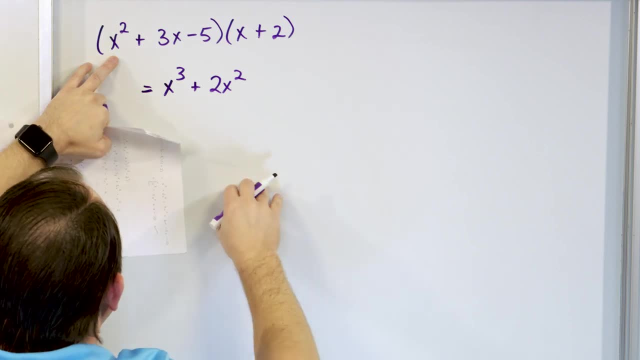 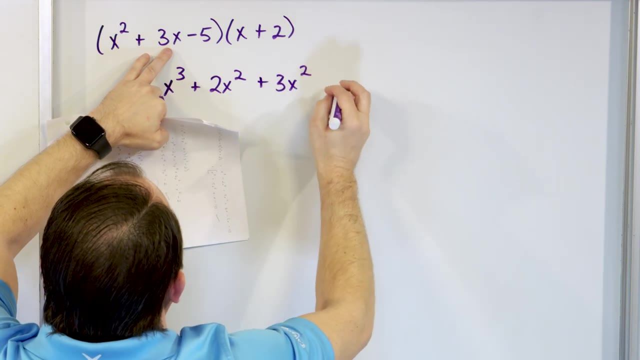 to give you 2x squared. Then you move to the next term. This one has to go into both of them. So 3x times x is 3x squared, And then 3x times 2 is 3 times 2 is 6.. So you're going to have 6x, right. 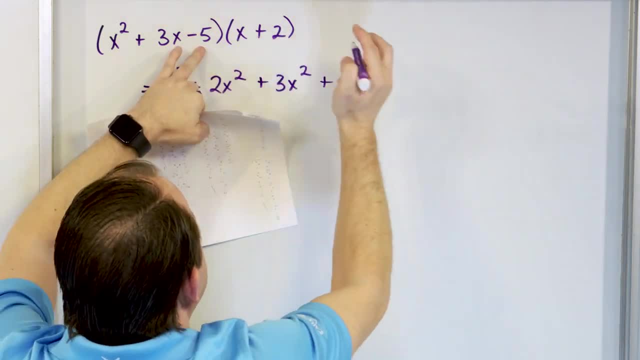 there. Now this one's a minus 5. Negative 5. So negative 5 times is x is negative 5 x, And then negative 5 times 2 is negative 10.. So you see, We still have the same way We. 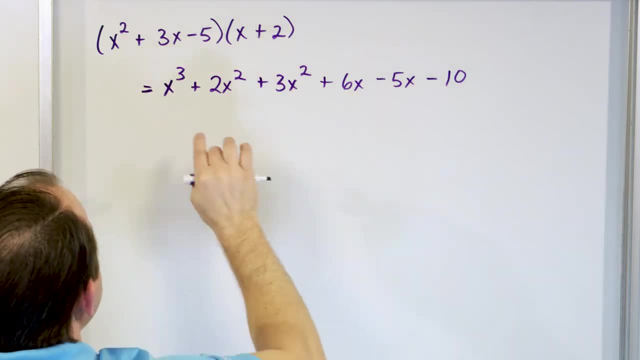 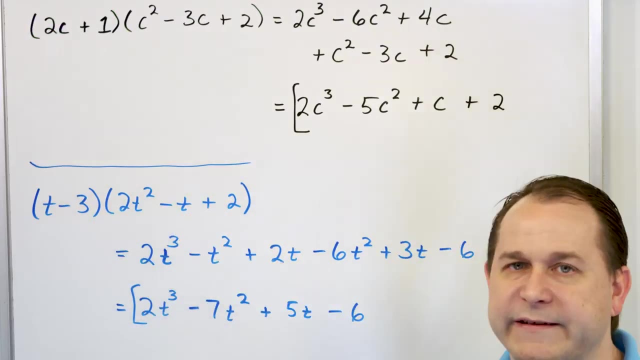 the same number of terms: One, two, three, four, five, six. Why? Because we have three terms on the outside, two terms on the inside. Three times two is six. We get six terms. Just like here. we have: two times three is six. So you see the order you have to be. 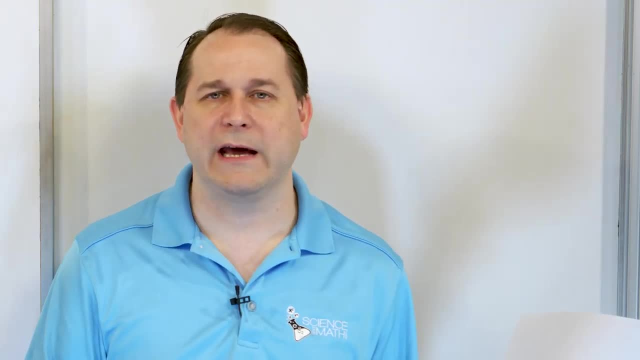 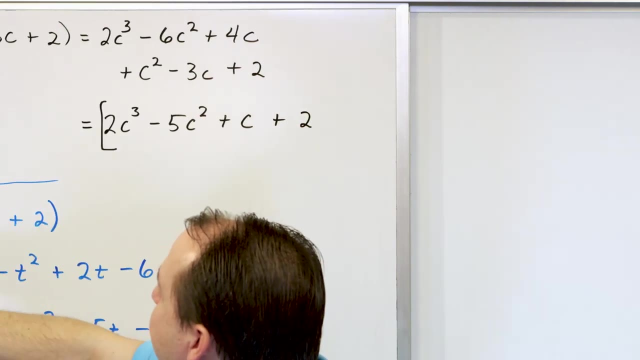 every topic that we do from here on out will have these polynomial multiplications in them, So you do need to get good at it, And that's where we're doing a lot of problems. Now let's turn it around a little bit. In all of these problems, I had two terms out here. 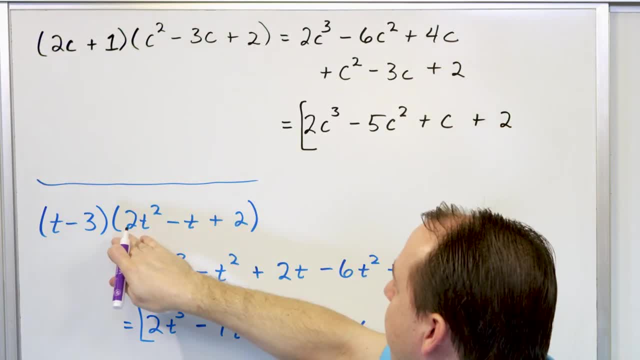 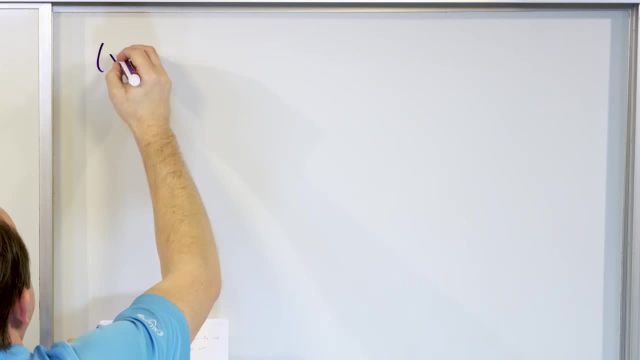 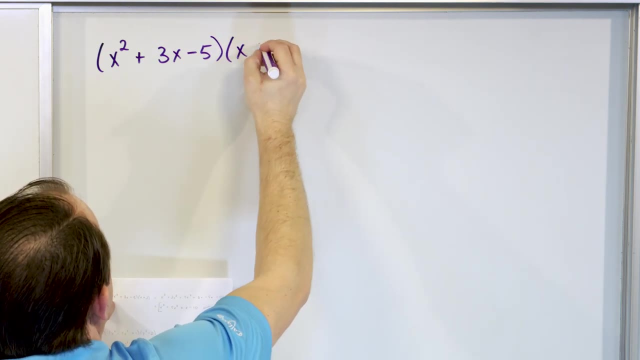 like here's: two terms multiplied by this trinomial, which is three terms. So two binomial times trinomial. Now take a look at how this one differs. What if I have x squared plus 3x minus 5.. And then I'm multiplying that times x plus 2.. 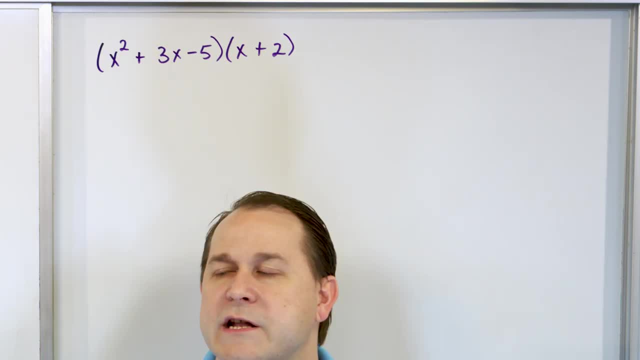 Now see, if you're just memorizing things like FOIL F-O-I-L, not only do you not know how to do the last type of problem, but you don't know how to do this one, because what's in front is actually: 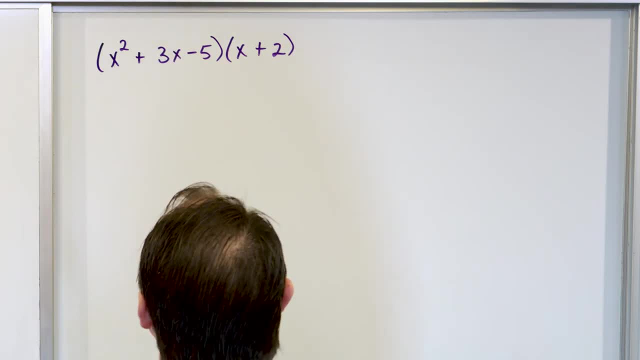 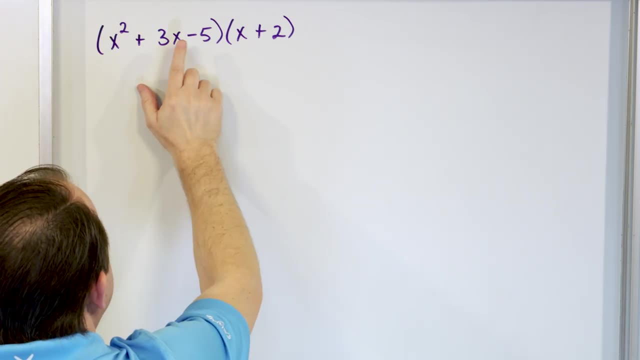 three terms multiplied by two terms. So it differs even more than in the past. But now you know you're not going to fall for that. All you have to do to multiply. this is, every one of these terms has to individually go in and multiply times everything over here. So what you do, 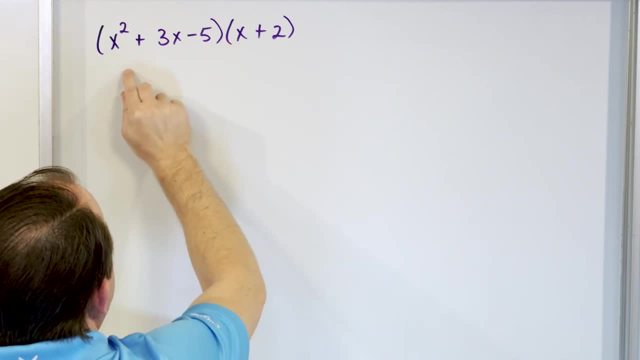 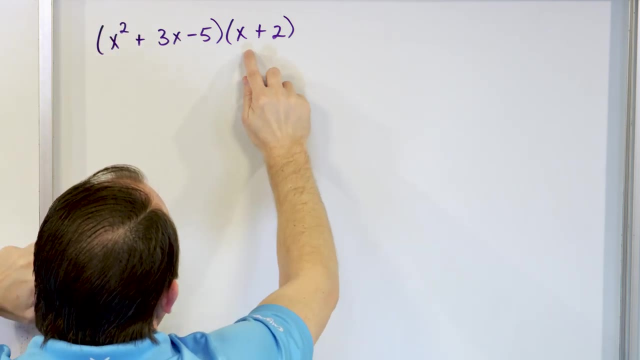 is: you cover both of these up, Pretend they're not there. This has to be multiplied in by those terms, Then you cover both of these. This one has to then be multiplied by both terms, Then you cover both of these. This one has to go in and multiply by both terms. So what you have is what is x. 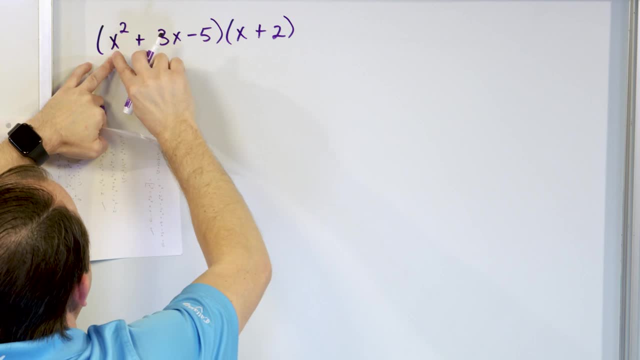 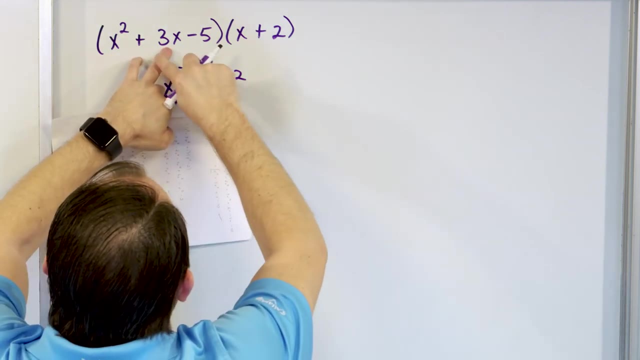 squared times x, You're going to get x to the third. Add the exponents: x squared times 2 is going to give you 2x squared. Then you move to the next term. This one has to go in to both of them. 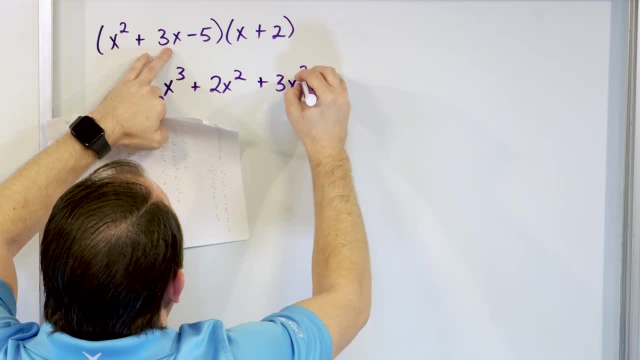 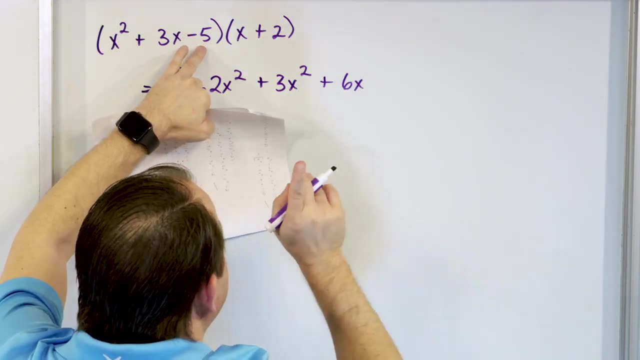 So 3x times x is 3x squared, And then 3x times 2 is 3 times 2 is 6.. So you're going to have 6x right there. Now this one's a minus 5, negative 5.. So negative. 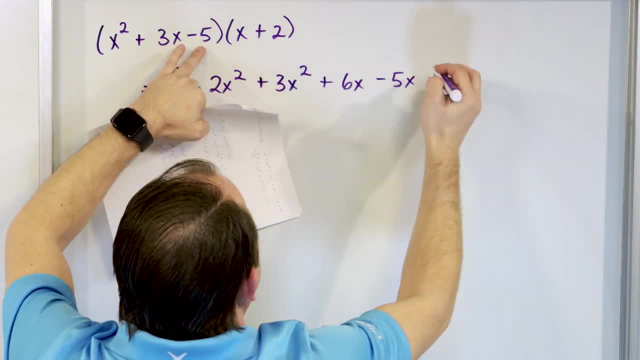 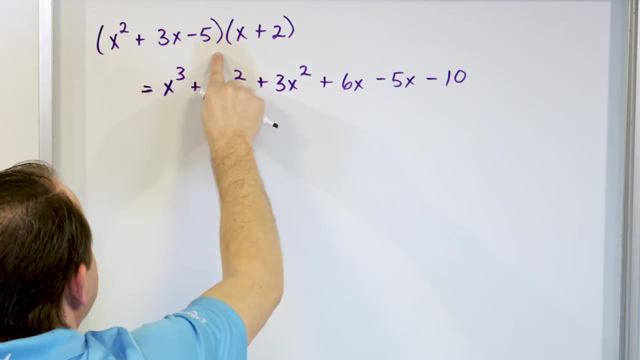 5 times x is negative 5x, And then negative 5 times 2 is negative 10.. So you see, we still have the same number of terms: 1,, 2,, 3,, 4,, 5, 6.. Why? Because we have 3 terms on the outside. 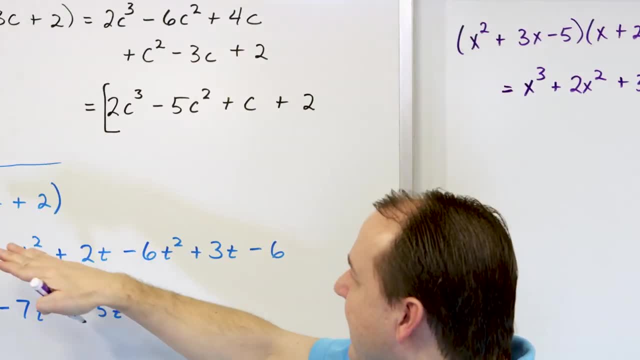 2 terms on the inside. 3 times 2 is 6.. We get 6 terms, Just like here we have. 2 times 3 is 6.. So you see the order. you have to be careful, You have to just make sure and distribute. 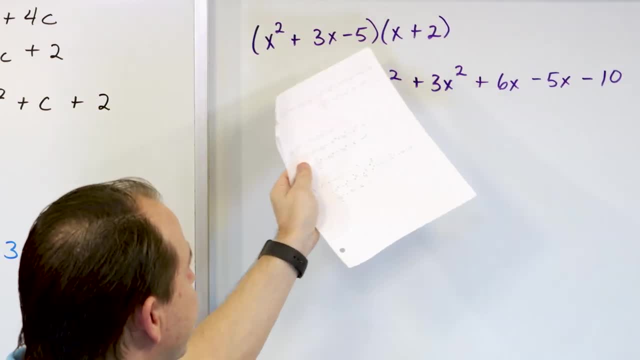 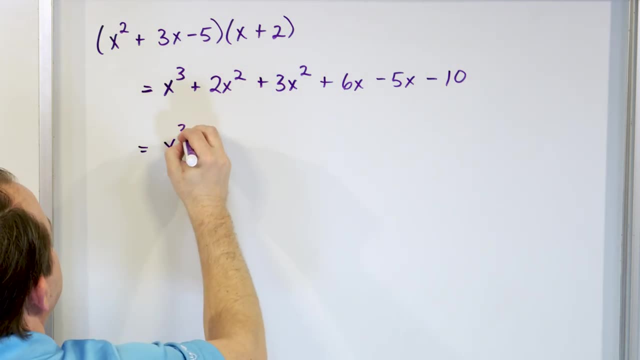 everything in, But we still expect to get 6 terms because of the total number of terms we have over here. So then we say: how many x cubed do we have? We have none, So this is just going to remain x cubed. How many x squares do we have? Well, I have one. 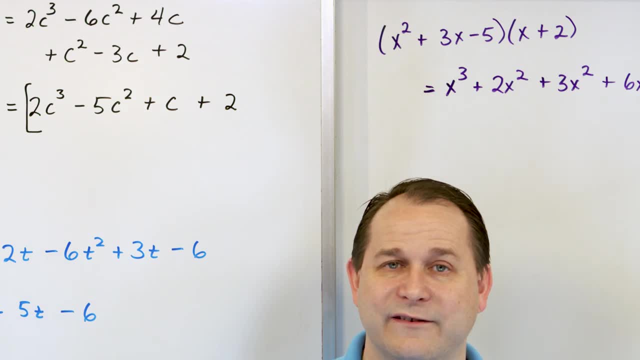 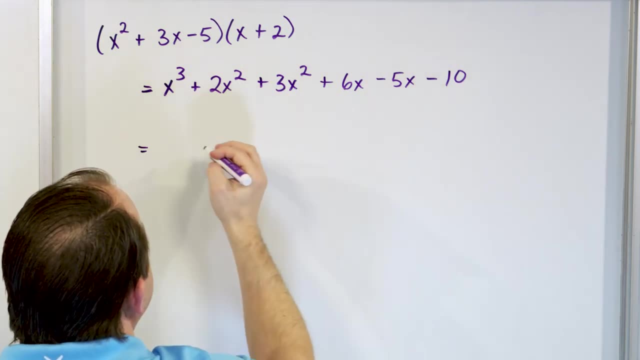 careful. You have to just make sure and distribute everything in. but we still expect to get six terms because of the total number of terms we have over here. So then we say, how many x-cubes do we have? We have none, so this is just going to remain. 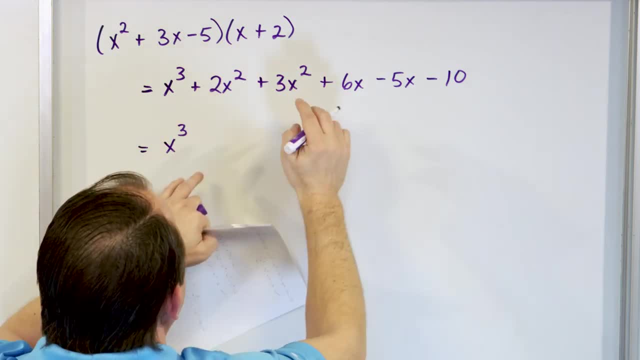 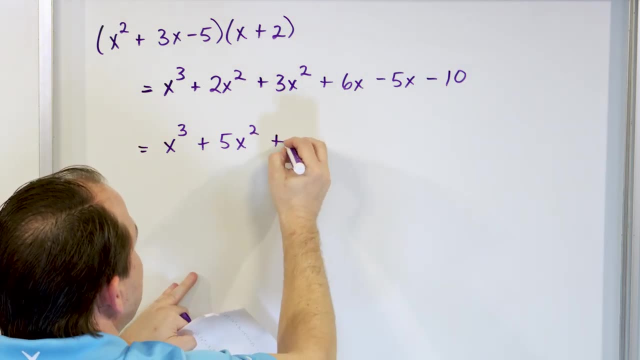 x-cubed. How many x-squares do we have? Well, I have one right next door. so two plus three is five x-squared. And then these are like terms. What is six minus five? It's going to give you one, so just write it as x, because it's really one x, And then you have minus. 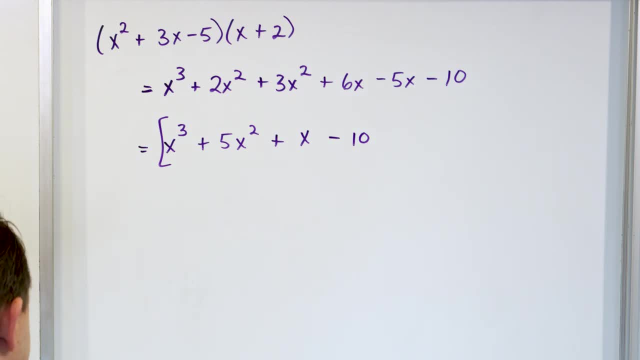 ten, And this is the final answer. Let's double check: X-cubed plus five, x-squared plus x minus ten. So that's the final answer. All right, Let's take a look at one that's about the same complexity We're just getting. 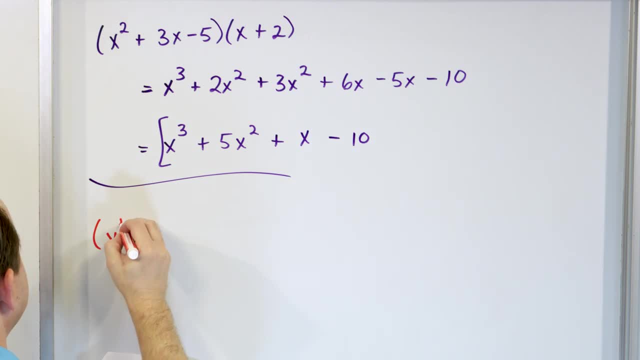 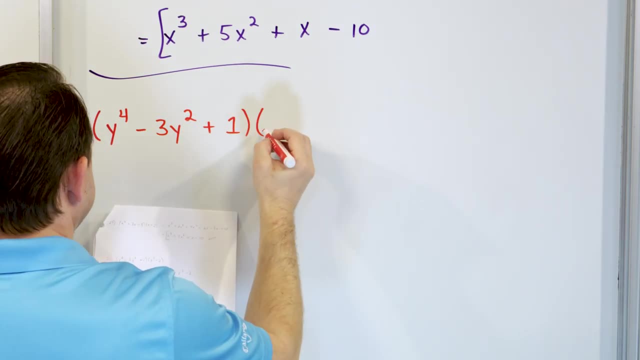 some practice A little bit higher exponents. It's the only real difference. What about y to the fourth power minus three, y-squared plus one multiplied times y-squared minus two? The only real difference between this and this is I have higher values of exponents. 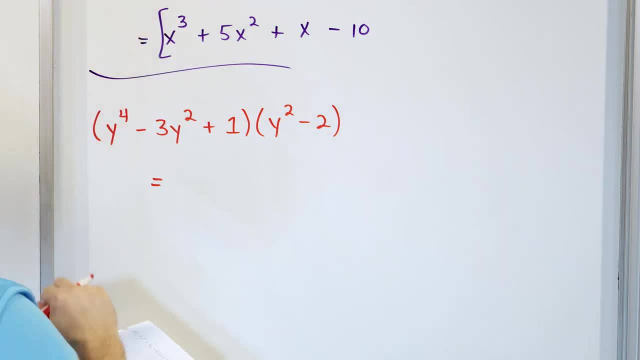 but exactly the same thing is done solution-wise. So we start with the first term and we start multiplying it in times, both of these. What do these two multiply together? We add the exponents together, because the base is the same. So that becomes y to the sixth power. 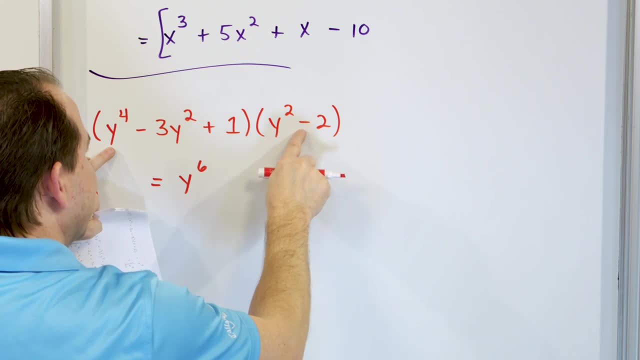 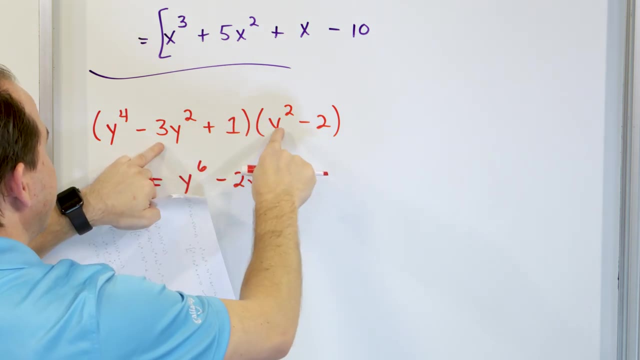 Four plus two is six Y can multiply times the negative two. Don't forget this is negative. So you get negative two y to the fourth power. when we multiply these, Then we move here and we do the same thing again. So the first term, negative three times one, is negative three y. We add the 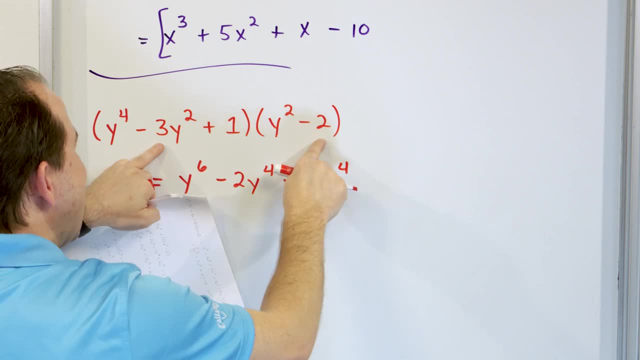 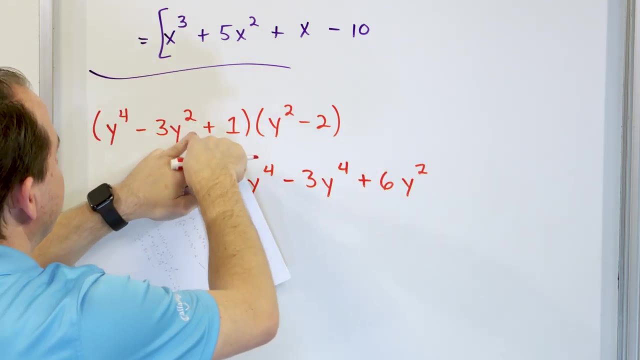 exponents. fourth power. Then negative three times negative two- don't forget your signs- makes it a positive six. And then you have the y-squared from here- Now we're done with this term, So we shift our finger here. One times y is y-squared. 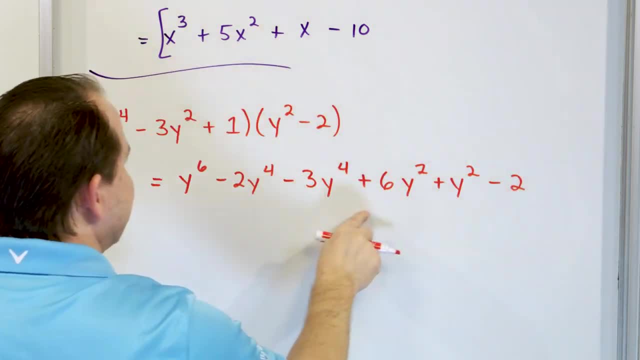 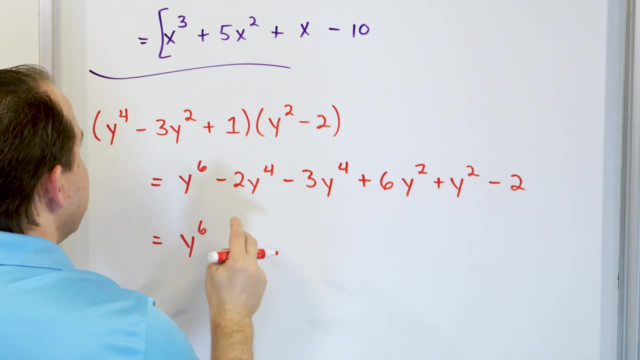 And then one times negative two is negative two And we should have six terms, And I think you can convince yourself that you do have six terms. So y to the sixth. we don't have any other terms like that, So he's going to stay in the front. Now we have y to the fourth. 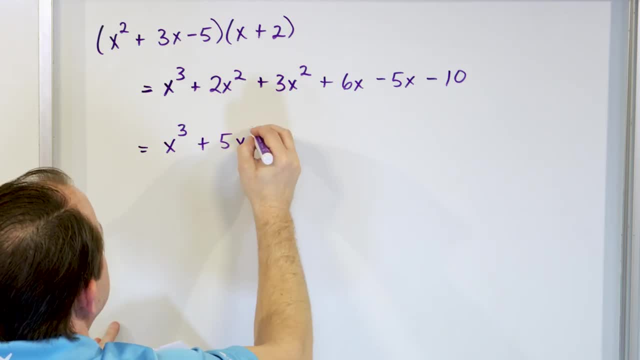 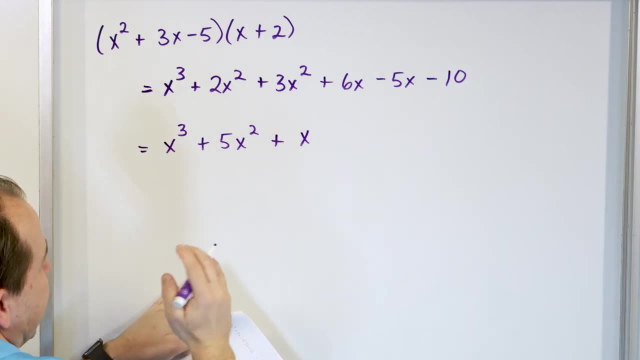 right next door. So 2 plus 3 is 5x squared. And then these are like terms. What is 6 minus 5?? It's going to give you 1.. So just write it as x, because it's really 1x, And then you have minus. 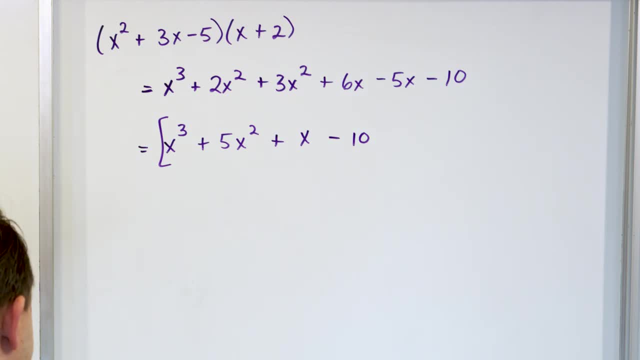 10.. And this is the final answer. Let's double check: x cubed plus 5x squared plus x minus 10.. So that's the final answer. All right, Let's take a look at 1.. That's about the same complexity, We're just getting some practice A little bit higher. 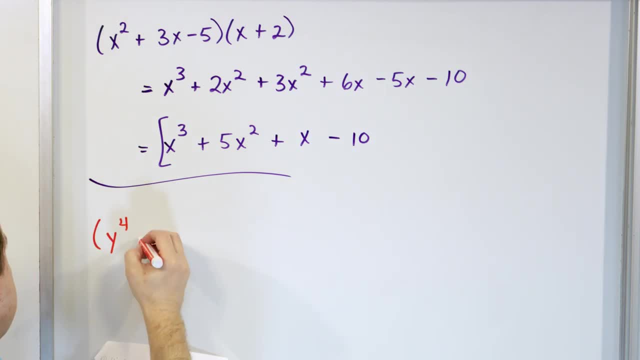 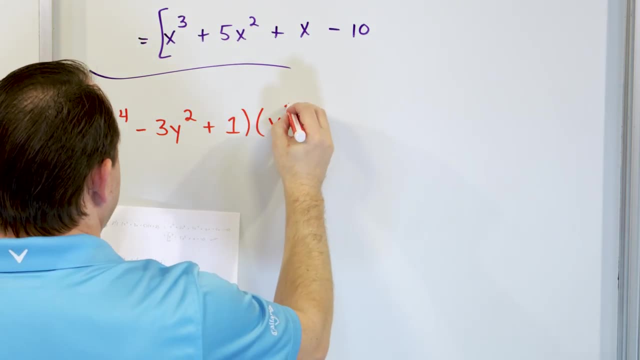 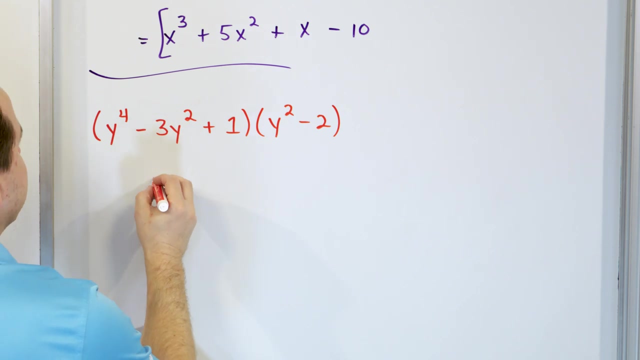 exponents. It's the only real difference. What about y to the fourth power minus 3y squared plus 1, multiplied times y squared minus 2?? The only real difference between this and this is I have a higher values of exponents, But exactly the same thing is done solution-wise. So we start with. 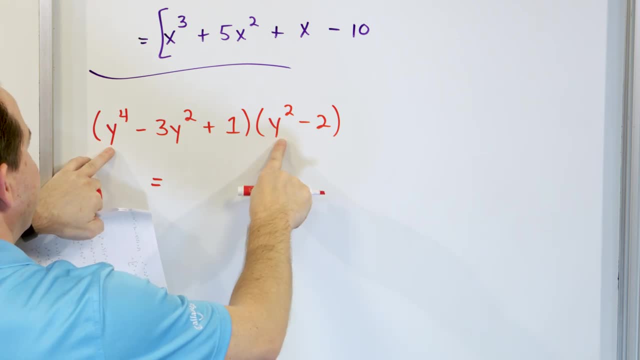 the first term And we start multiplying it in times, both of these. What do these two multiply together? We add the exponents together. We add the exponents together. We add the exponents together because the base is the same, So that becomes y to the sixth power. 4 plus 2 is 6.. 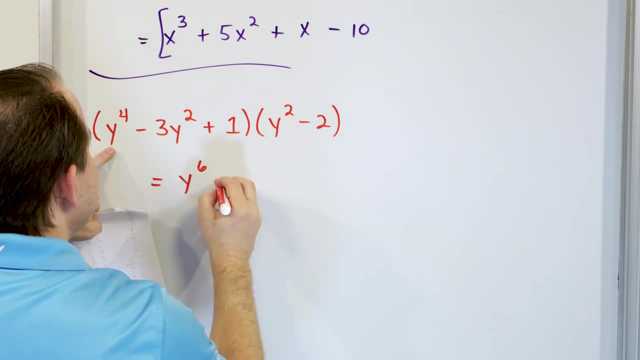 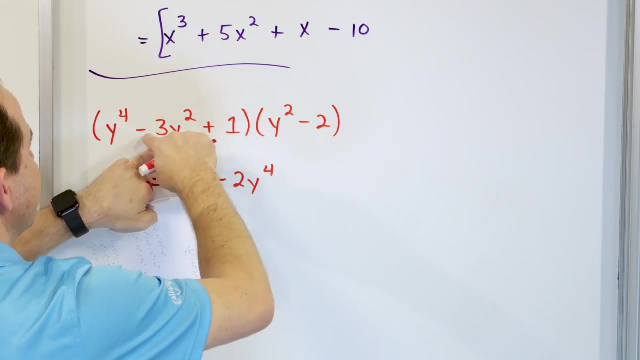 Then we take and multiply times the negative 2.. Don't forget: this is negative. So you get negative 2y to the fourth power when we multiply these. Then we move here And we do the same thing again. So the first term, negative 3 times 1, is negative 3y. We add the exponents fourth power, Then 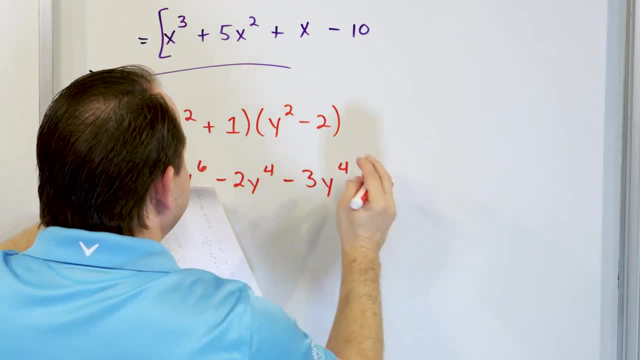 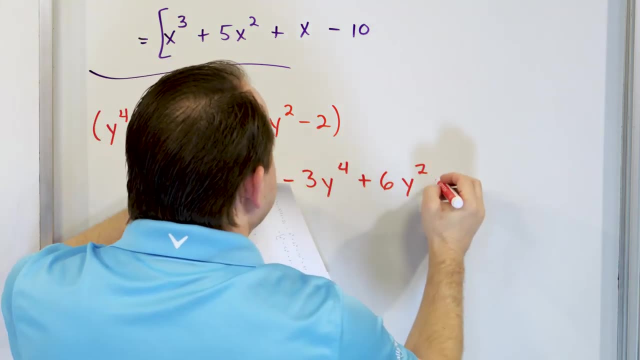 negative. 3 times negative 2, don't forget your signs- makes it a positive 6.. And then you have the y squared from here- Now we're done with this term- We shift our finger here: 1 times y is y squared, And then 1 times negative, 2 is negative 2.. 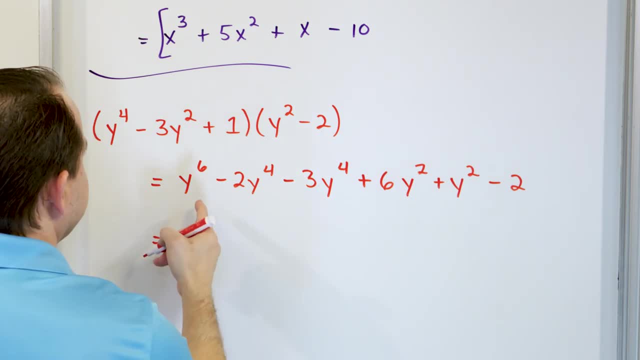 We should have six terms, And I think you can convince yourself that you do have six terms. So y to the sixth. We don't have any other terms like that, So he's going to stay in the front. Now we have y to the fourth. What's negative 2? Minus 3 gives you negative 5.. y to the fourth. 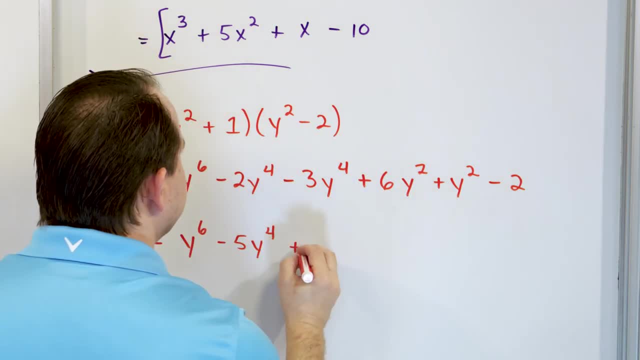 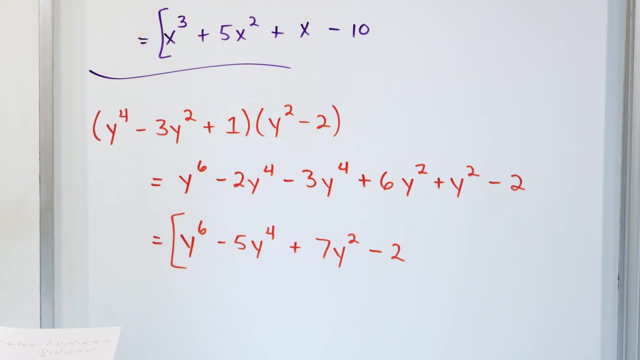 power. These terms are the same: 6 plus 1 is 7.. y squared. And then the minus 2 comes along the side. So let's go ahead and circle that and check it. y to the sixth power minus 5y to the fourth. 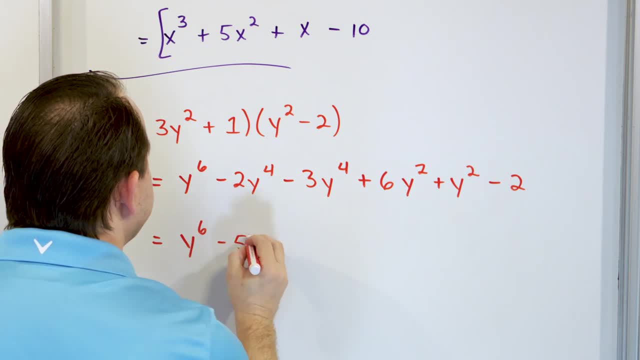 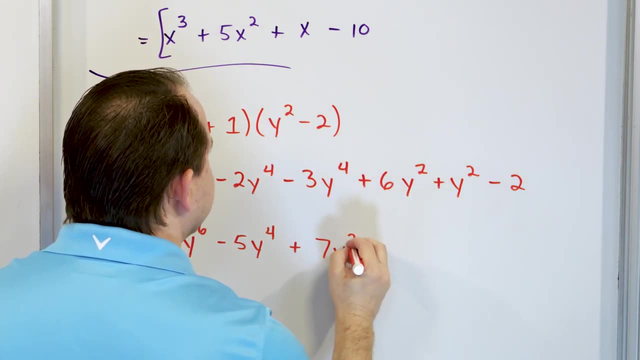 What's negative? two Minus three gives you negative five. Y to the fourth power- These terms are the same: Six plus one is seven y-squared, And then the minus two comes along the ride. So let's go ahead and circle that and check it. Y to the sixth power minus five. 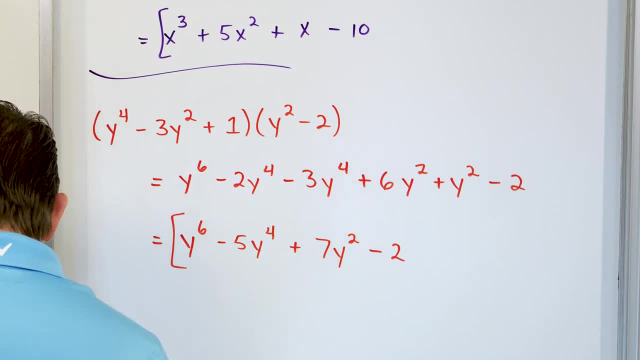 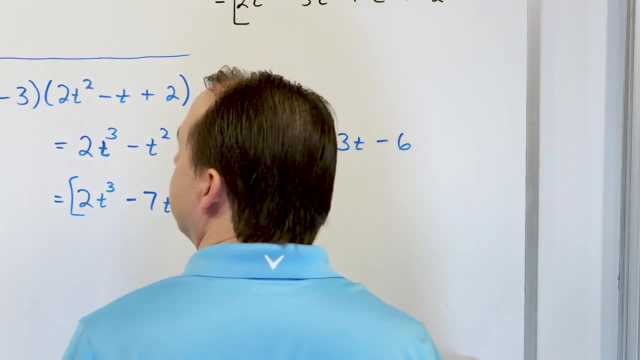 y to the fourth plus seven y-squared, And then the minus two comes along the ride, So it's seven y-squared minus two. All correct Now only one more problem in this lesson. Notice that what we've done is we've started with. 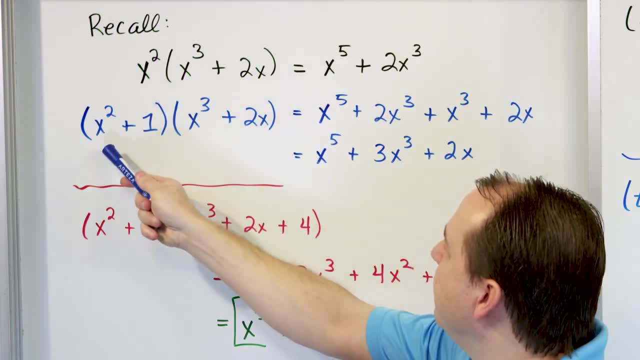 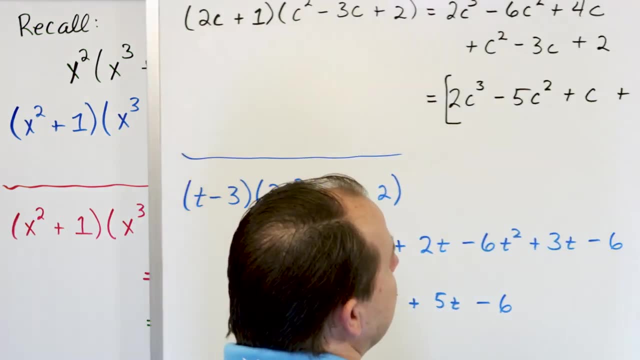 the simplest thing: Distribute on the outside. We got that. OK, What happens if we have two things on the outside? We distribute both of them. OK, What if you have something bigger? We just distribute each thing in, as we've always done. What if you have three things? 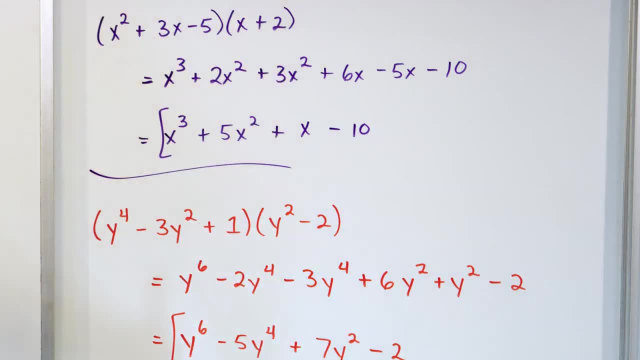 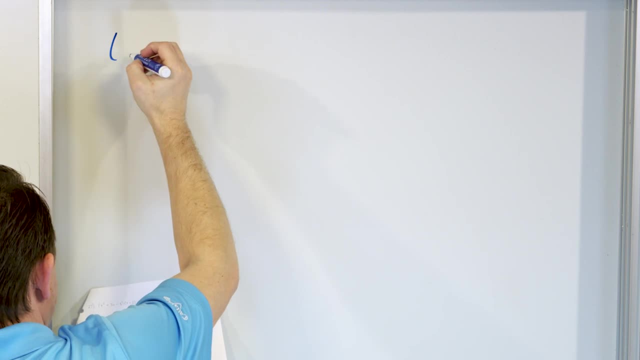 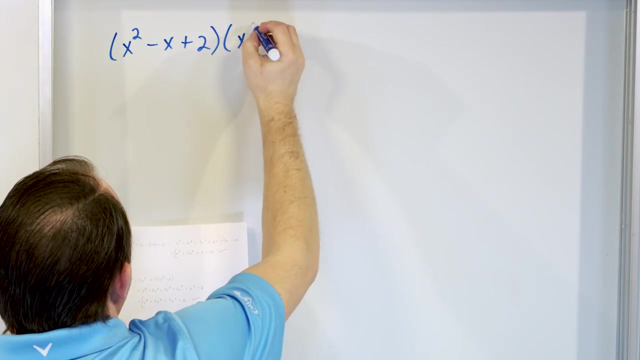 on the outside. Well, you just distribute each term in from the outside to the inside. Now for our final problem of this lesson. We should see the pattern by now. What do you do if you have this? What do you have? six-squared minus x plus two, multiplied by six-squared plus x minus one. 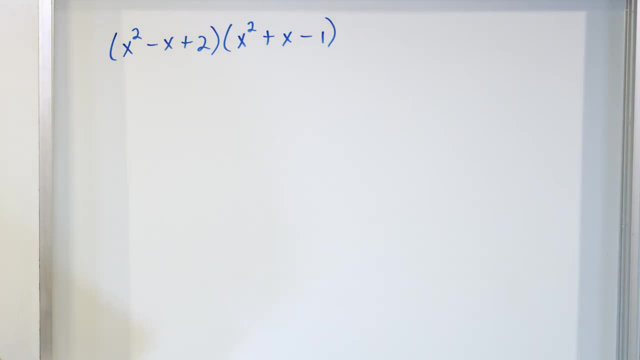 So this is three terms times three terms. So this one's larger than any of the other problems before. But by now you should see the pattern. We just take this first thing and distribute it in Boom, boom, boom. That's three terms. 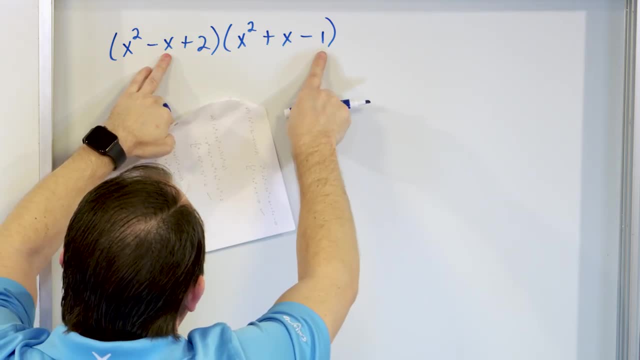 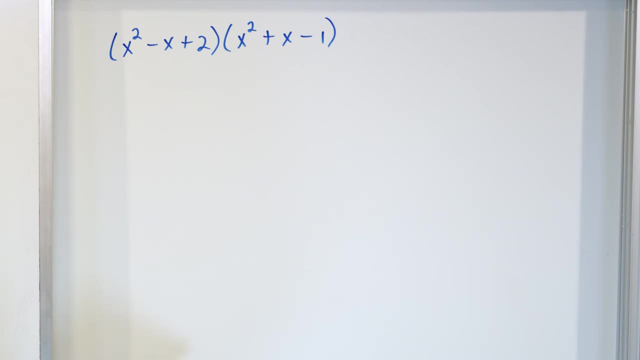 right there. Then we move here, We distribute it in broom boom, boom. That's three more terms. Then we move this one in boom boom, boom. that's three more terms. So three times three, we should expect to see nine terms all together. 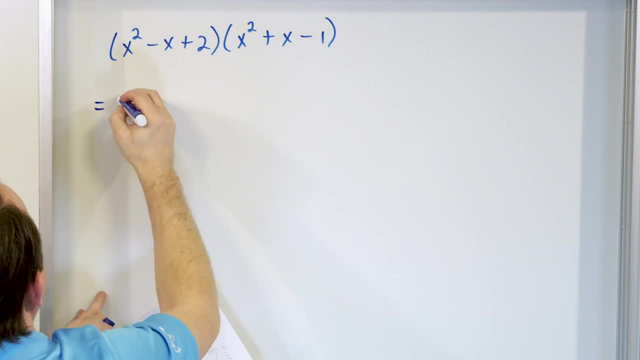 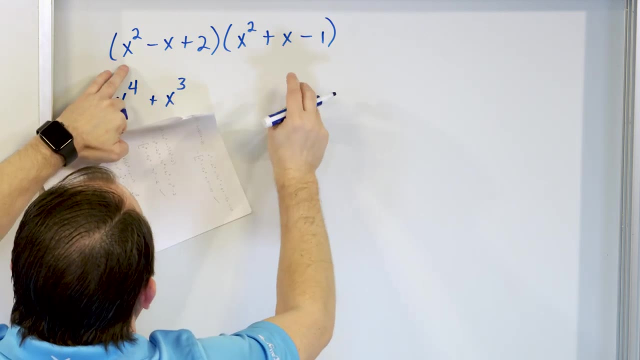 Let's just double check and see what we get. So we have x squared. times x squared gives you x. add the exponents to the fourth power. This times this gives you x to the third. This times this negative one here times that gives you negative one: x squared, so negative. 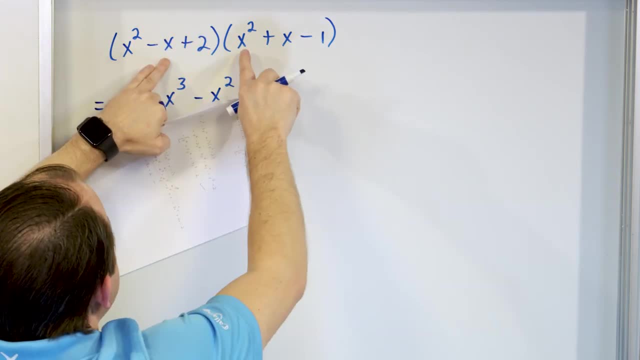 x squared is what you write down. Then you shift your finger to this. this is a negative x. times this negative one times the positive one means you get a negative x. You add the exponents and make it to the third power. 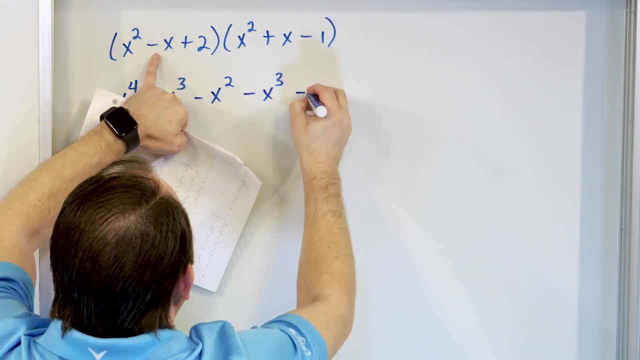 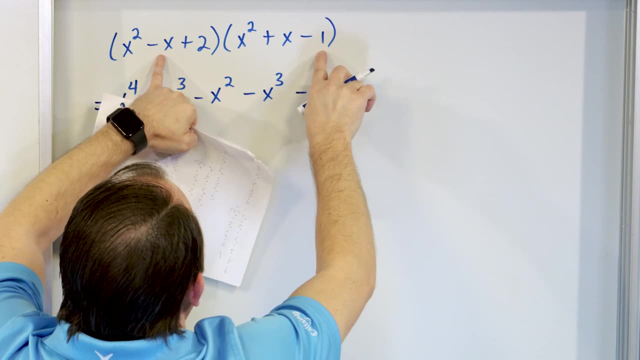 Then this one times this one- this is negative times- positive- gives you negative x and you add the exponents, which means x squared. Then, whoops, we have one more times the negative one. Negative times. negative is positive x. x times one is x, right. 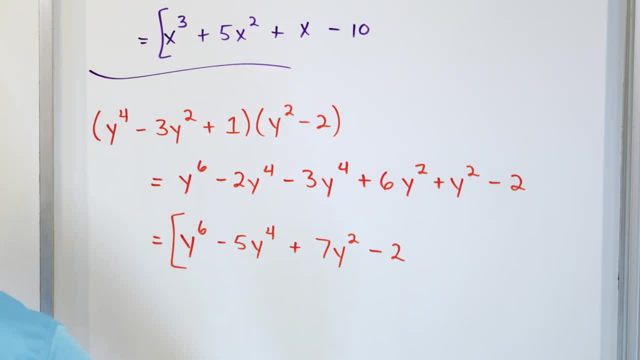 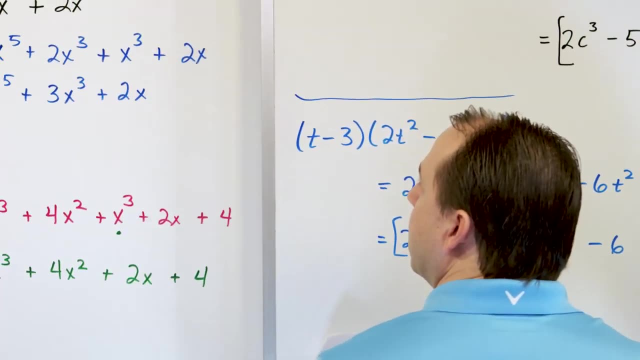 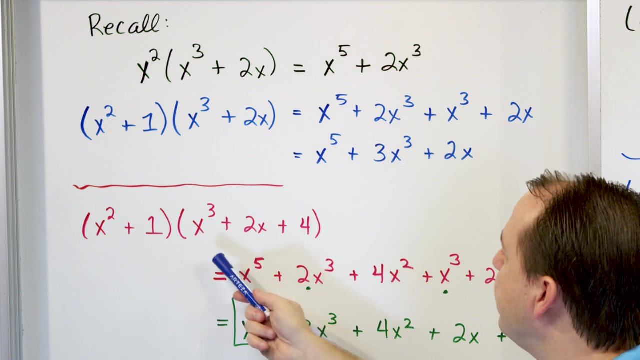 plus 7y, squared minus 2.. All correct. Now only one more problem in this lesson. Notice that what we've done is we've started with the simplest thing: Distribute on the outside. We got that, OK. What happens if we have two things on the outside? We distribute both of them, OK. What if? 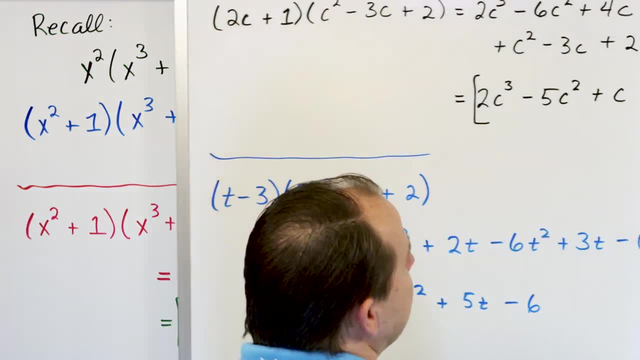 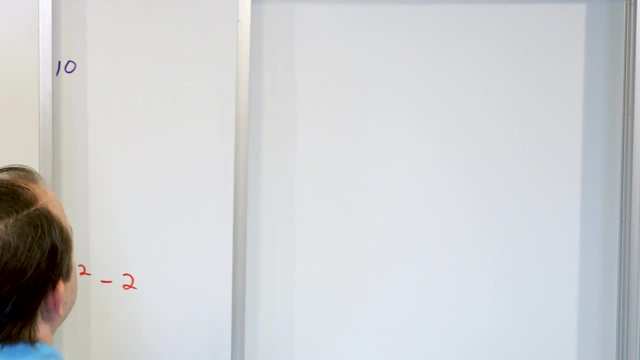 you have something bigger, We just distribute each thing in, as we've always done. What if you have three things on the outside? Well, you just distribute each term in From the outside to the inside. Now for our final problem of this lesson. 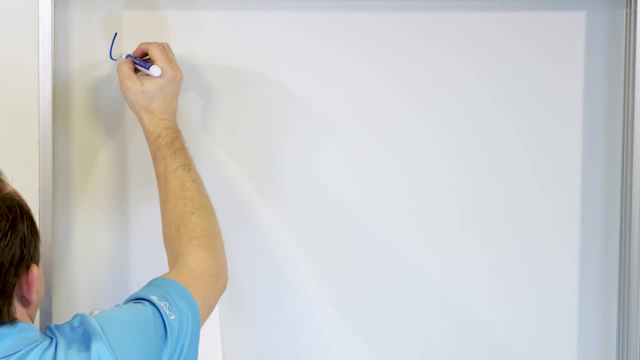 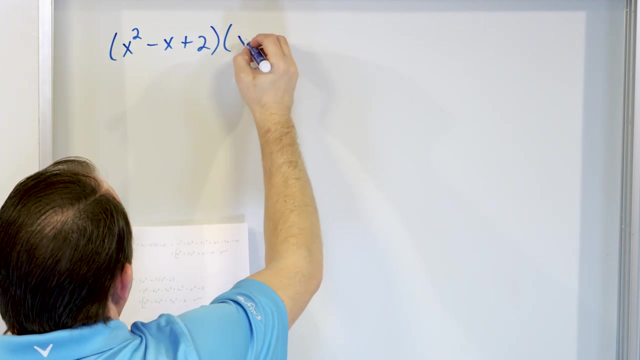 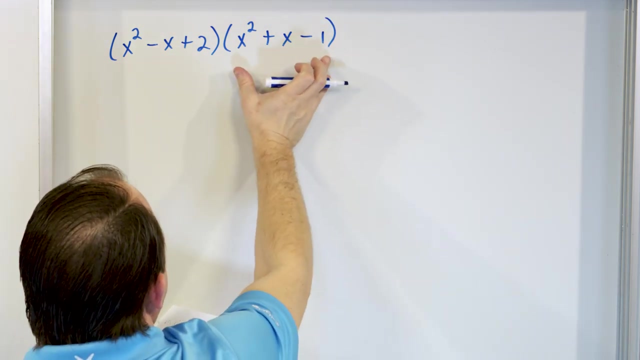 you should see the pattern by now. What do you do if you have this? What if you have x squared minus x plus 2, multiplied by x squared plus x minus 1? So this is three terms times three terms. So this one's larger than any of the other problems before. But by now you should see the. 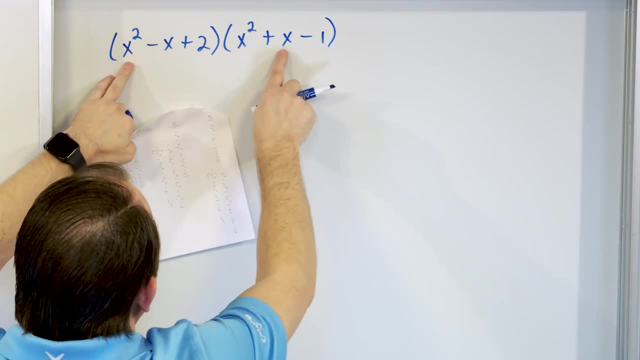 pattern. We just take this first thing and distribute it in Boom, boom, boom. That's three terms. right Now, what happens if we have x squared minus x plus 2 multiplied by x squared plus x plus 1? Right there, Then we move here, Distribute it in Boom, boom, boom. That's three more terms. 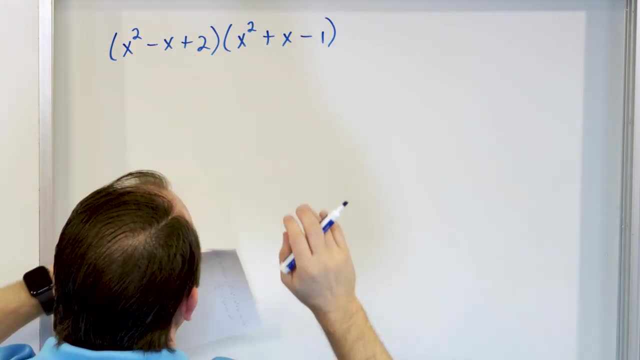 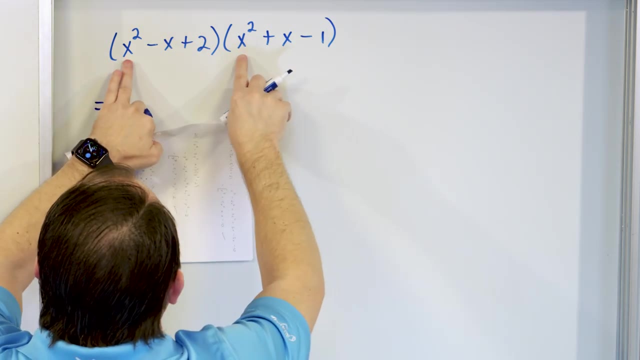 Then we move this one in: Boom, boom, boom. That's three more terms. So three times three, We should expect to see nine terms altogether. Let's just double check and see what we get. So we have x squared times. x squared gives you x. Add the exponents to the fourth power. 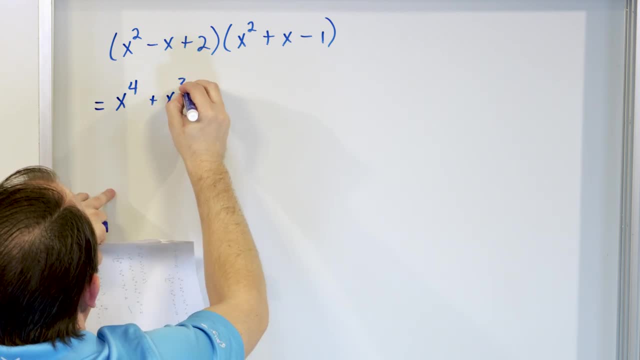 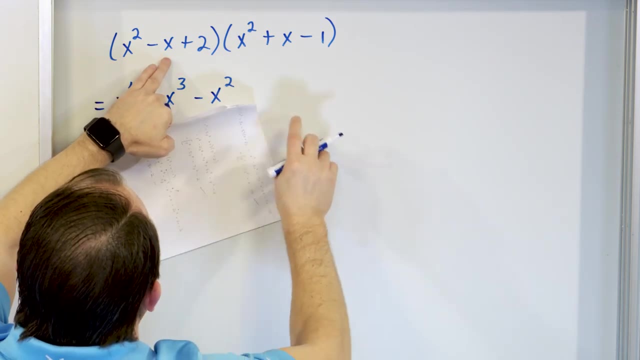 This times this gives you x. to the third: This times this Negative 1 here times that gives you negative 1x squared. So negative x squared is what you write down. Then you shift your finger to this Times this Negative 1 times the positive 1 means you get a negative x. You add the exponents and 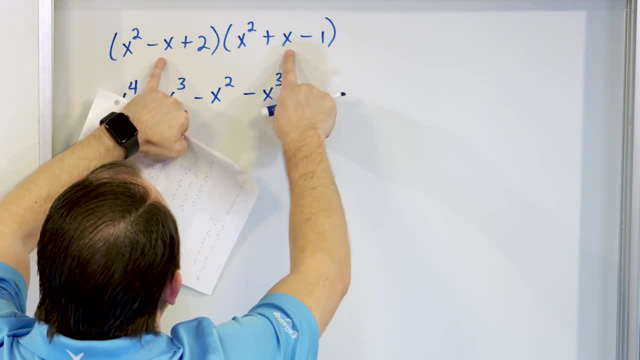 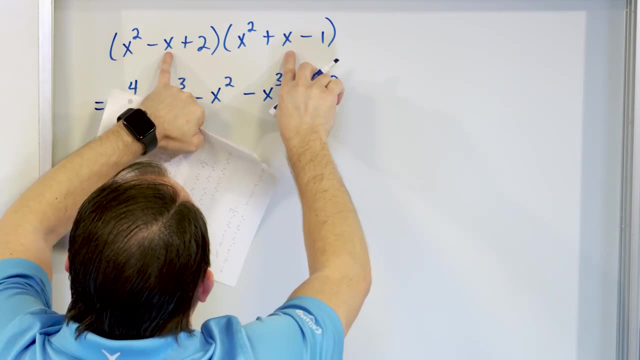 make it to the third power. Then this one times this one- This is negative times positive- gives you negative x And you add the exponents, which means x squared, Then whoops, we have one more times the negative 1.. Negative times negative is positive x. x times 1 is x. right, Then we shift. 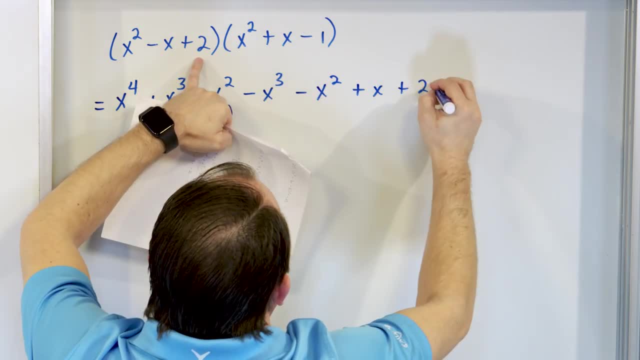 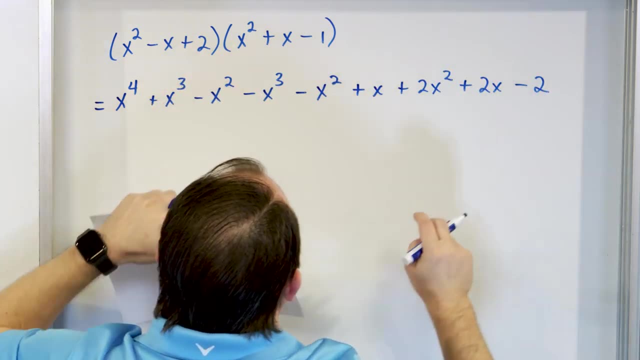 here We have 2 times the x squared, So we get 2x squared, Then we have 2 times the x, Then we have 2 times the negative 1, which makes negative 2 for the final answer. One, two, three, four, five. 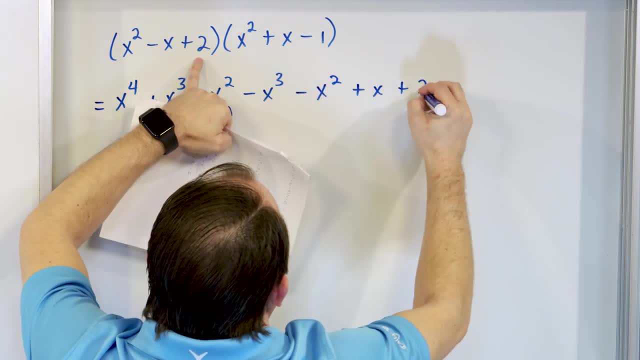 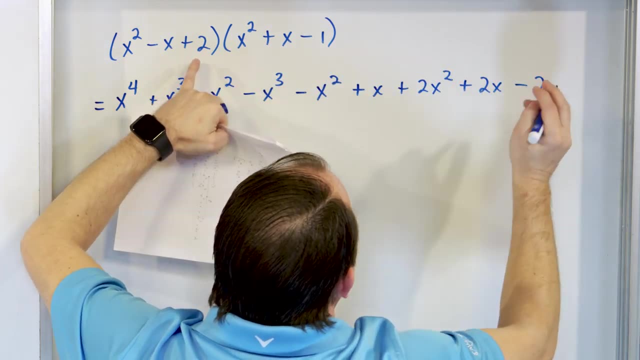 Then we shift here. We have two times the x squared, so we get two x squared, Then we have two times the x, Then we have two times the negative, one which makes negative x Negative two. for the final answer: One, two, three, four, five, six, seven, eight, nine terms. that's what we got. 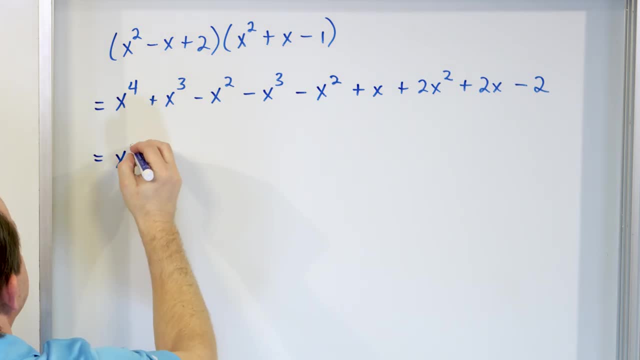 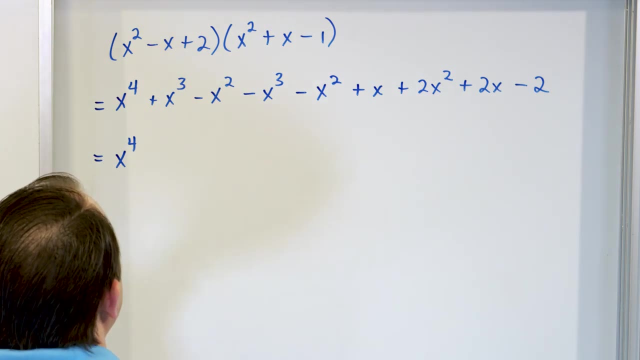 Now we simplify. There are no other x to the fourth, so he stays in the front. We have an x to the third term. Now here's where things get interesting. We have an x to the third term here. we have an x to the third term here as well, but it's. 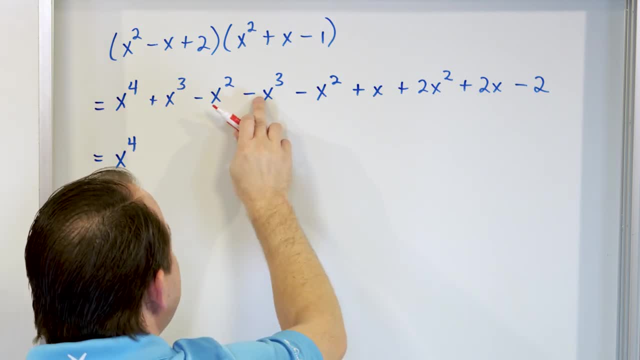 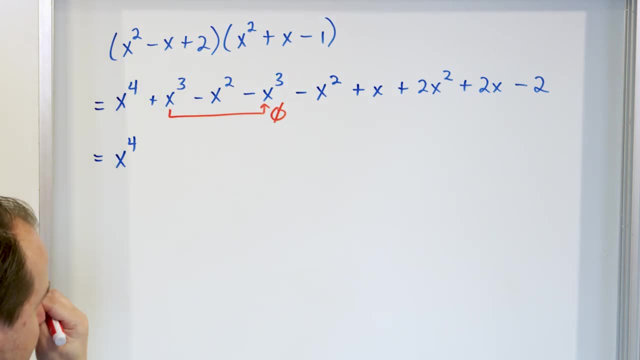 a negative, So this positive one cancels with the negative one in front of the x to the third. So here what we actually get is zero And we add these together right, Because one plus a negative one gives you zero. So the x to the third terms drop away completely. 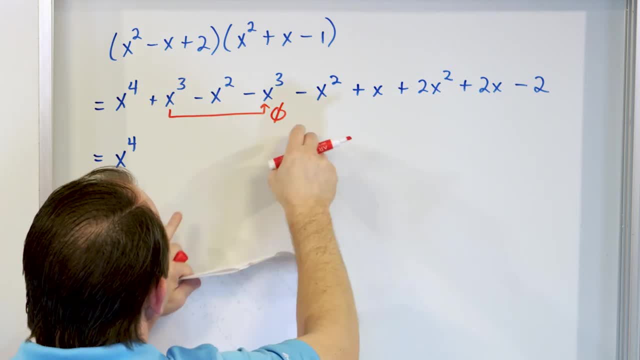 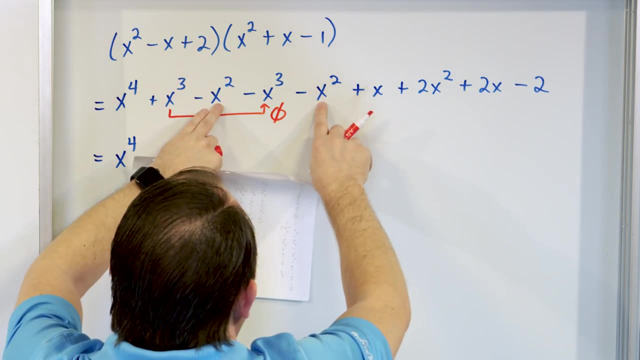 So we say, okay, we'll remember that. but let's go and take a look at the x squared. Well, here's a negative x squared and here is another negative x squared and here's another positive, two x squareds here. 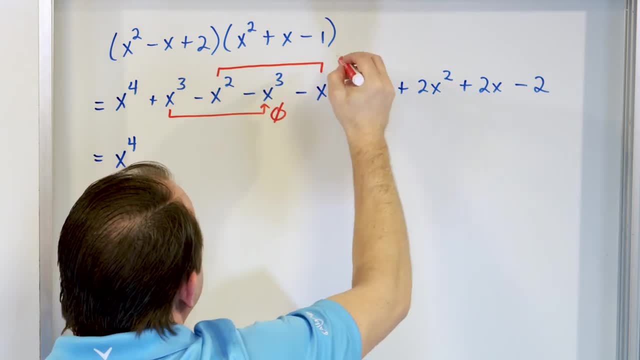 So we're going to basically add all these. So let's go and say: well, we're going to add these and we're going to add it to this one down here, because that's an x squared term, that's an x squared term and that's an x. 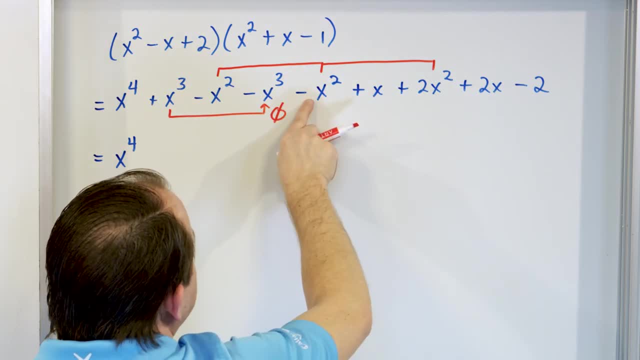 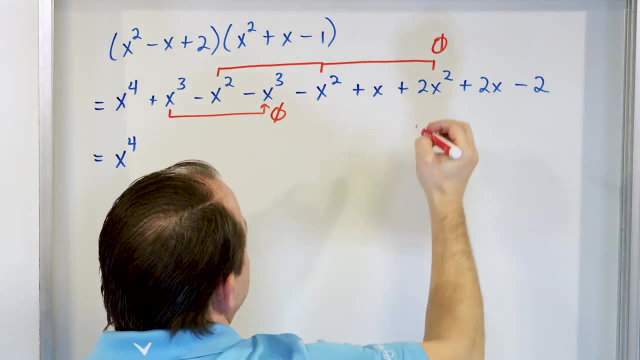 squared term. But here's what you have: Negative one plus negative one gives you negative two x squared. That negative two x squared is going to add with the positive two x squared, and these terms are also going to give you zero. I'm putting a slash through it so you don't think I'm writing an O or something. 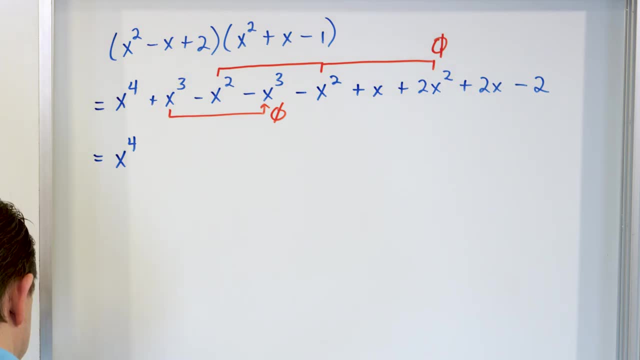 Basically these add to zero and the x squared terms add to zero. So you've actually canceled a lot of your answer because this term is not going to be in the answer. that term's not going to be in the answer. that term's not going to be. 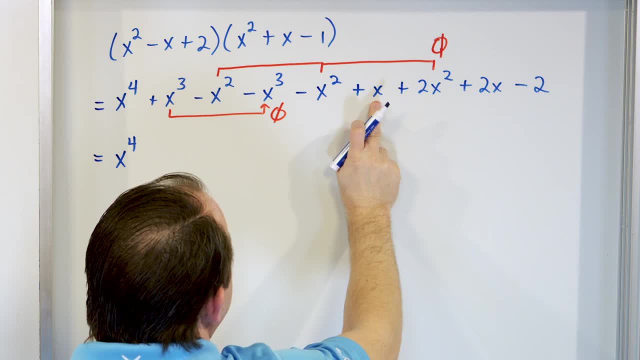 in the answer. that one's not going to be in the answer, This one I have done nothing for. Just because I've done so much, let me write it down. And then this one is not going to be, it's going to be in the answer. let's just keep. 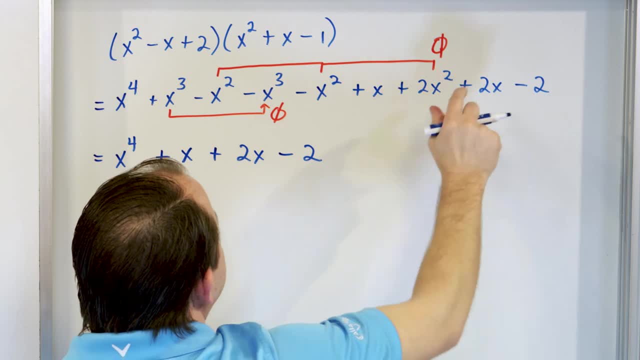 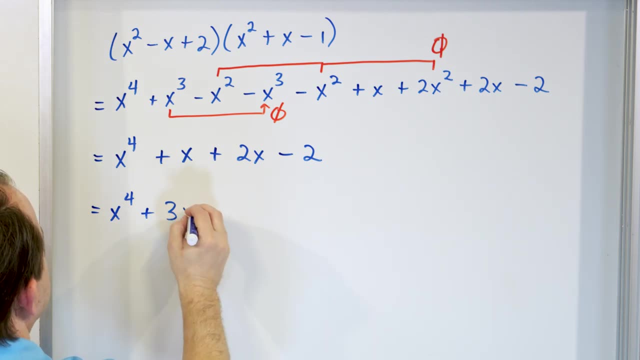 it for now. we'll add it later, and then we have the minus two. Basically, all of these terms that touched red are gone. Then in our final answer we just add these: one plus two is three x minus two. This is the final answer: x to the fourth plus three x minus two. 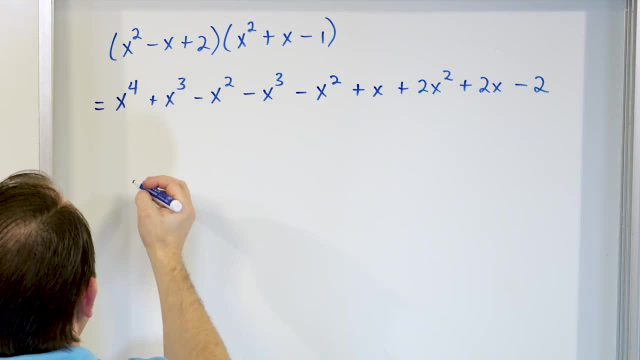 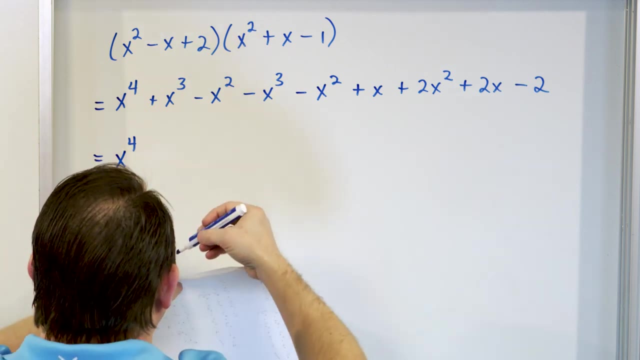 six, seven, eight, nine terms. That's what we got. Now we simplify. There are no other x to the fourth, so he stays in the front. We have an x to the third term. Now here's where things get interesting. 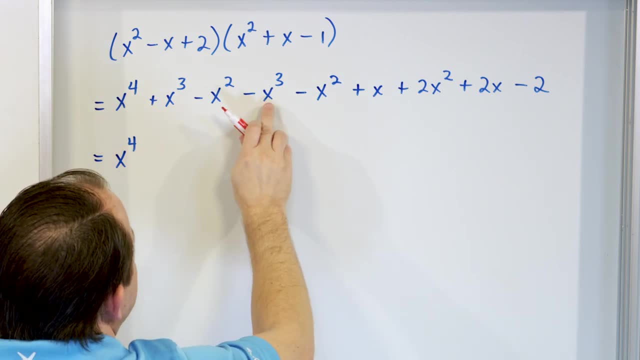 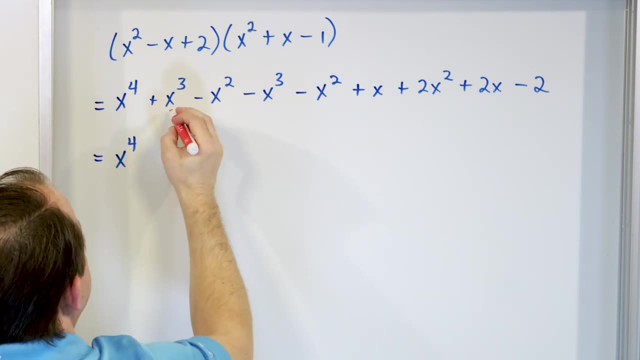 We have an x to the third term here. You have an x to the third term here as well, but it's a negative. So this positive 1 cancels with the negative 1 in front of the x to the third. So here what we actually get. 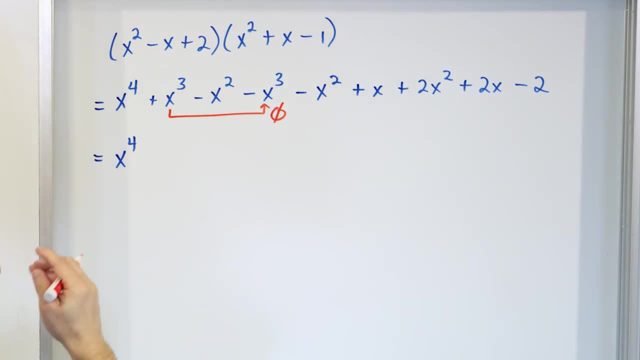 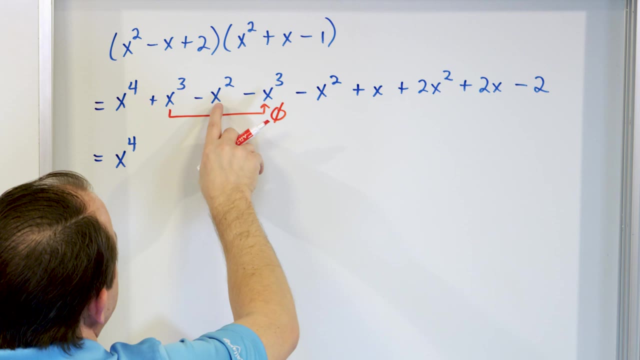 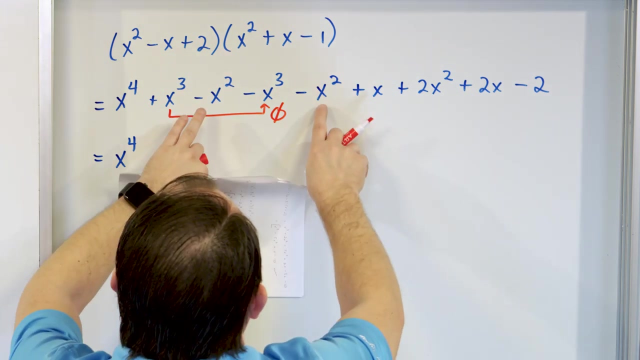 is 0 when we add these together. right, Because 1 plus a negative 1 gives you 0.. So the x to the third terms drop away completely. So we say, OK, we'll remember that, But let's go and take a look at the x squared. Well, here's a negative x squared And here is another negative. 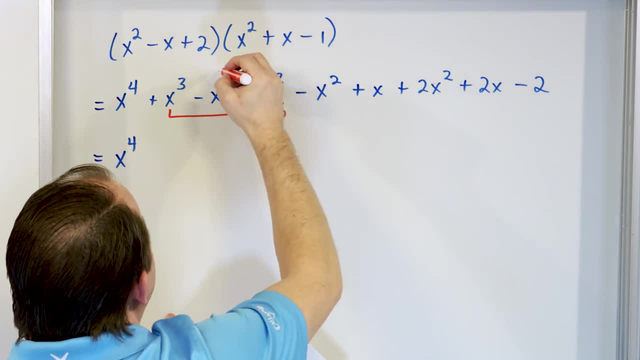 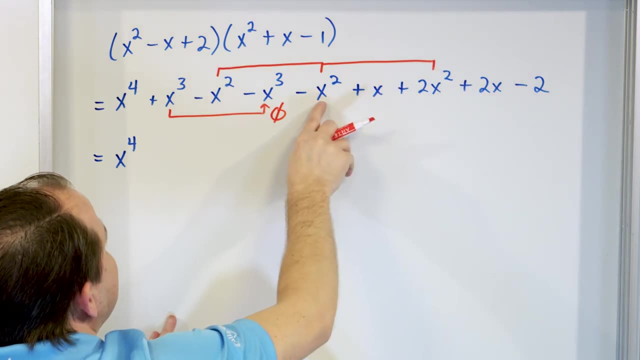 x squared And here's another positive 2x squared here. So we're going to basically add all these. So let's go and say: well, we're going to add these And we're going to add it to this one down here, because that's an x squared term. That's an x squared term. 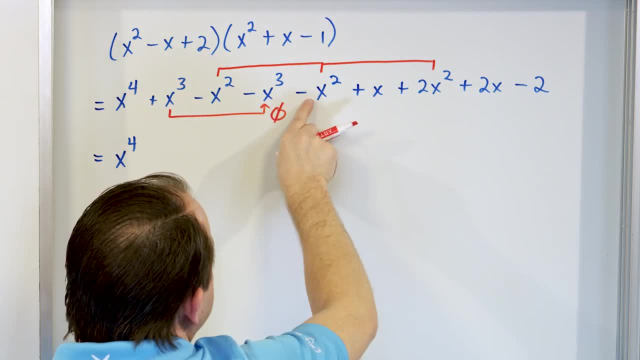 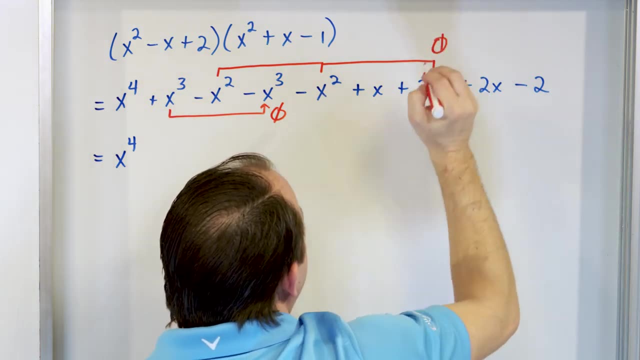 But here's what you have: Negative 1 plus negative 1 gives you negative 2x squared. That negative 2x squared is going to add with the positive 2x squared, And these terms are also going to give you 0.. I'm putting a slash through it so you don't think I'm writing an. 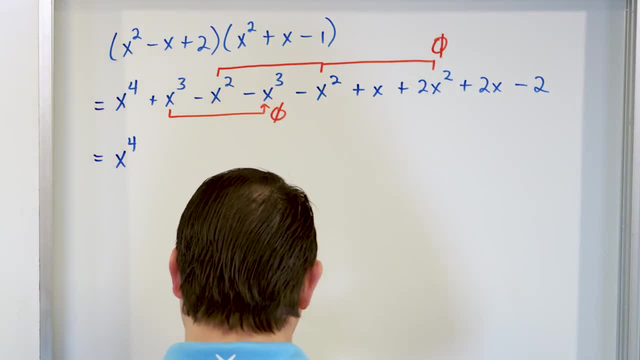 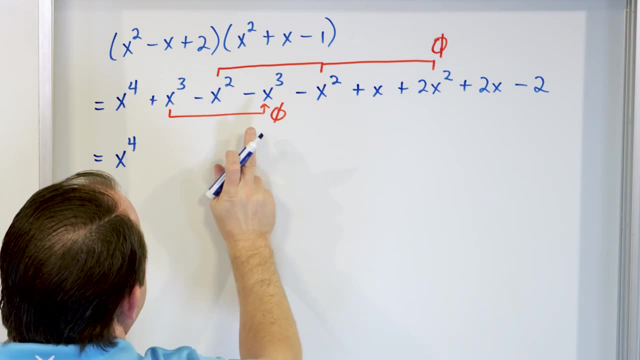 O or something. Basically, these add to 0. And the x squared terms add to 0. So you've actually canceled a lot of your answer because this term is not going to be in the answer. That term's not going to be answered. That term's not going to be in the answer. That. one's not going to be in the answer, This one I have done nothing for, So I'm going to do this, I'm going to do this, And then I'm going to do this, And then I'm going to do this, And then I'm going to do this. 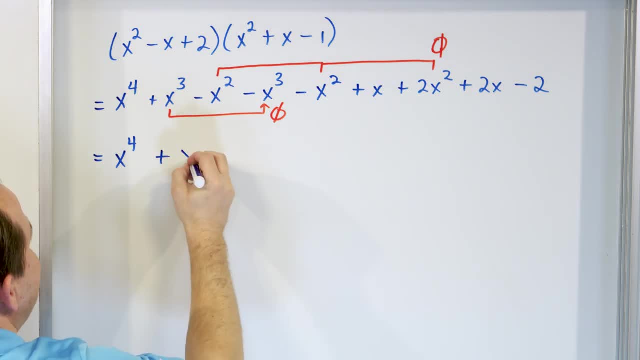 done nothing for. So for now, just because I've done so much, let me write it down. And then this one is not going to be. it's going to be in the answer. Let's just keep it for now. We'll add it. 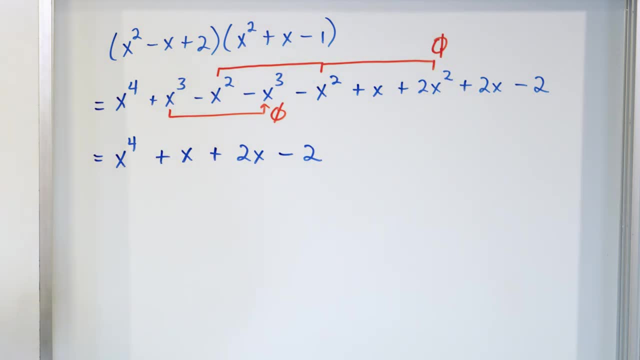 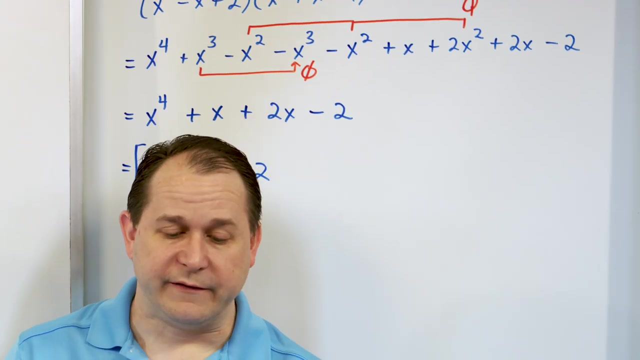 later. And then we have the minus two. Basically, all of these terms that touched red are gone. Then in our final answer we just add these: One plus two is three X minus two. This is the final answer: X to the fourth, plus three X minus two. So congratulations, You now know how to multiply. 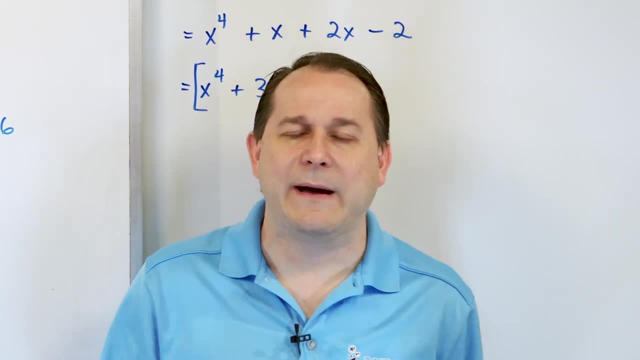 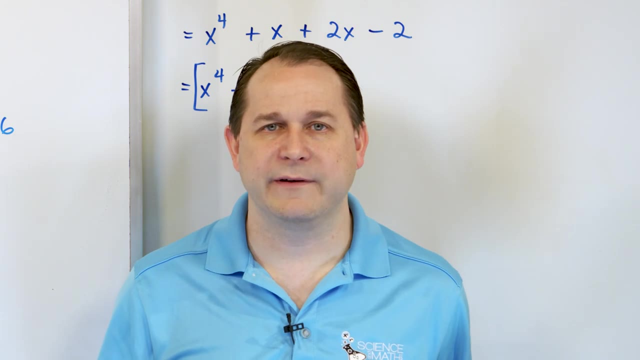 polynomials. right, We start off by teaching you the basic idea about how to distribute terms in, and then you learn binomial times binomial. Then you learn trinomial times trinomial, And now I hope you can see that you can now multiply anything times anything, no matter how many. 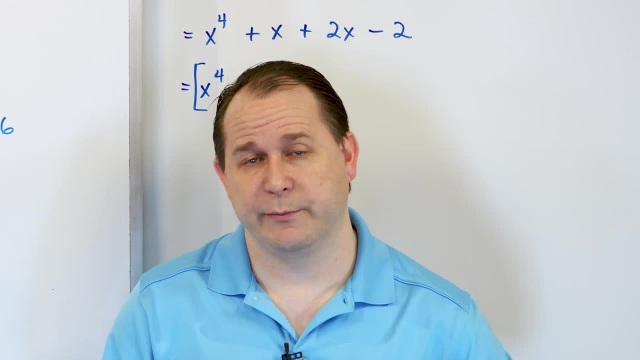 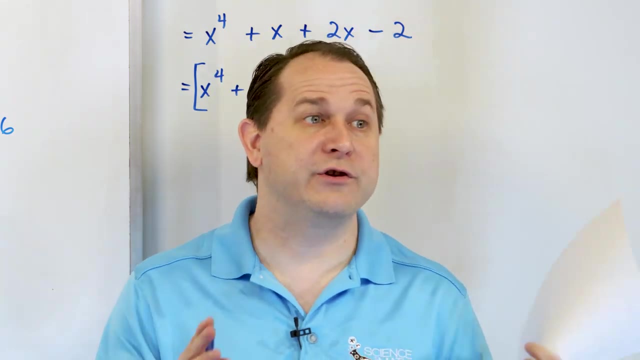 So, congratulations, you now know how to multiply polynomials, right? We start off by teaching you the basic idea about how to distribute terms in, And then you learn binomial times binomial. then you learn trinomial times trinomial. 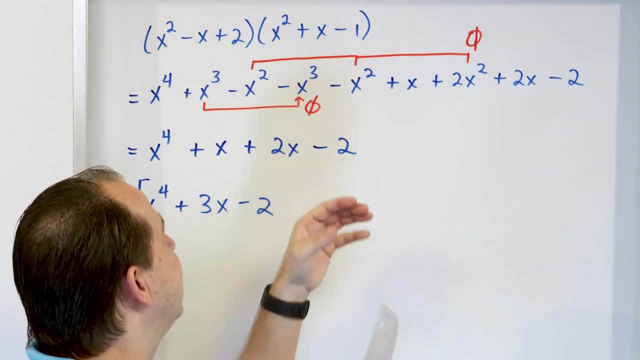 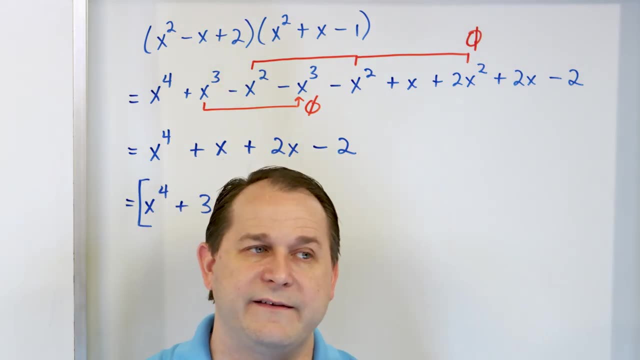 and now I hope you can see that you can now multiply anything times anything. no matter how many terms I give you, The same pattern holds: you just distribute everything on the outside times everything on the inside, and as everything gets larger, you're going to have more and more terms to. 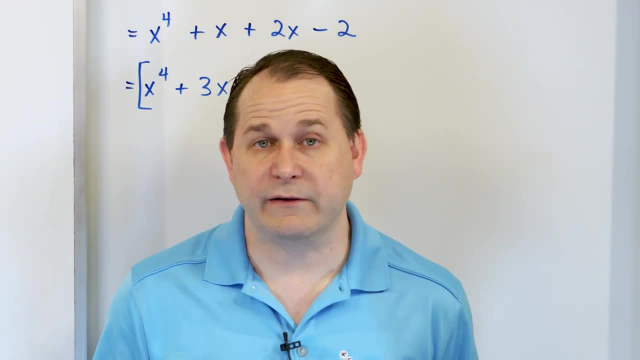 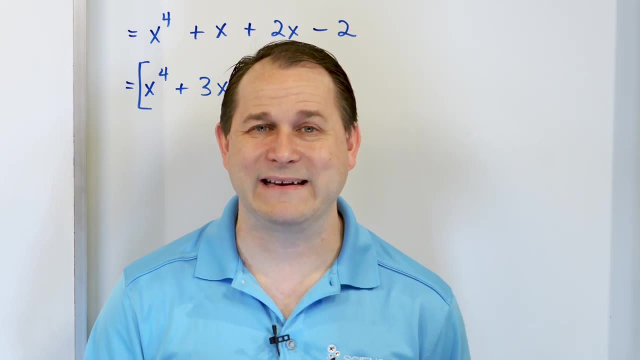 simplify at the end. So we've done this and you should have a good foundation for how to handle these things. but follow me on to the next lesson. we'll continue multiplying polynomials. crank up the problem of complexity just a little bit. 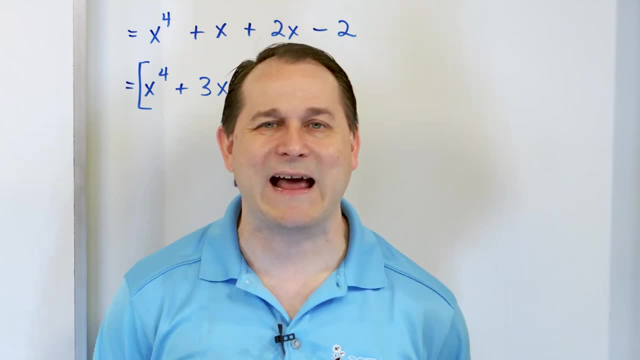 But you will be able to understand how to do all of them, because all of them follow the exact rules that we've laid out in this section. 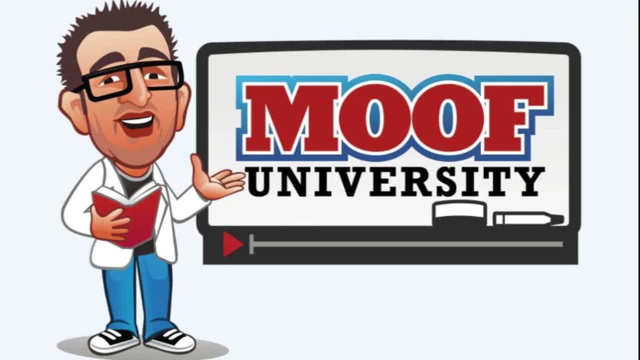 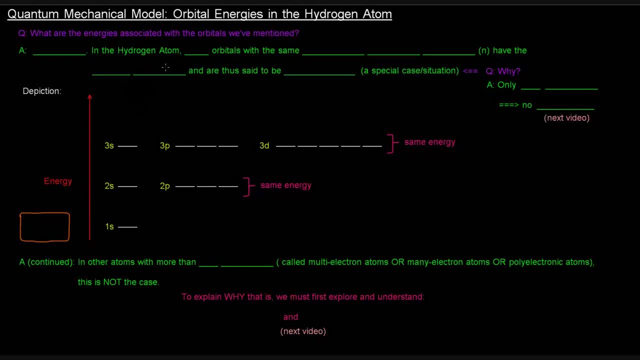 For more information on tutoring or how to support MUF University and the production of more videos, please visit MUFUniversitycom. Thank you and enjoy. So this question is: what are the energies associated with the orbitals we've mentioned? And the answer to that question depends. 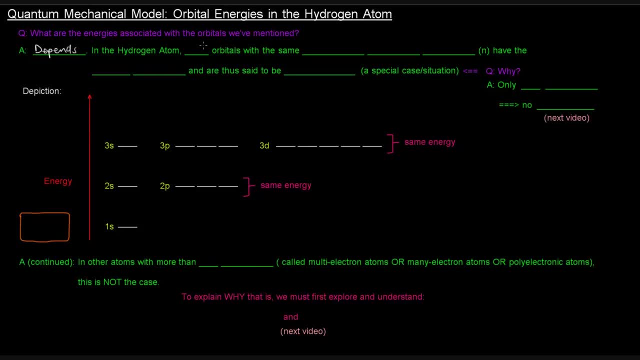 So, if you're talking about the hydrogen atom, which is what this video is particularly going to cover, the orbitals, all of the orbitals with the same principal quantum number, which is n, all the orbitals with the same principal quantum number, n, have the same energy. 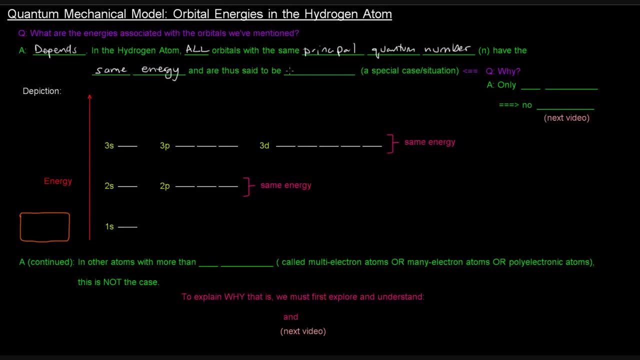 They are all of equal energy and they are thus said to be degenerate, So that's a special case or situation. Now, why is this? It's specifically because the hydrogen atom has only one electron. It has only one electron, So there is no shielding, which we'll kind of talk about in the next video. 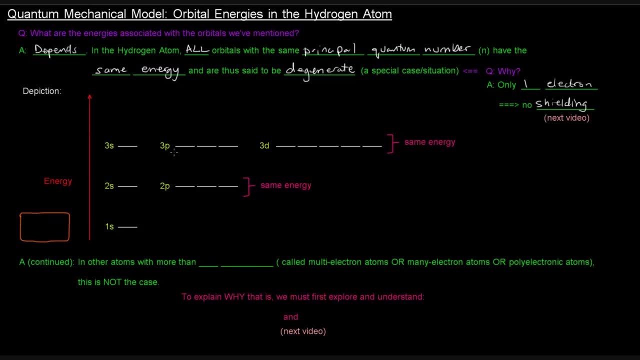 I'll get to what that means later, But the way that's sort of depicted, with all these orbitals with the same principal quantum number having the same energy, is like this: If we think about this axis here, this arrow pointing up to mean energy increasing right.